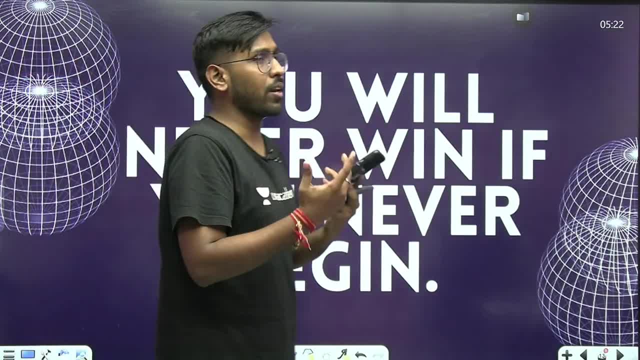 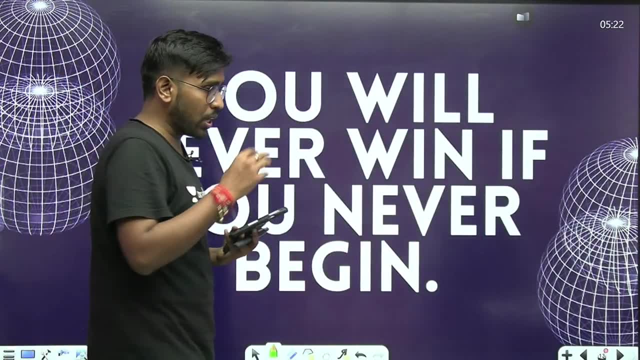 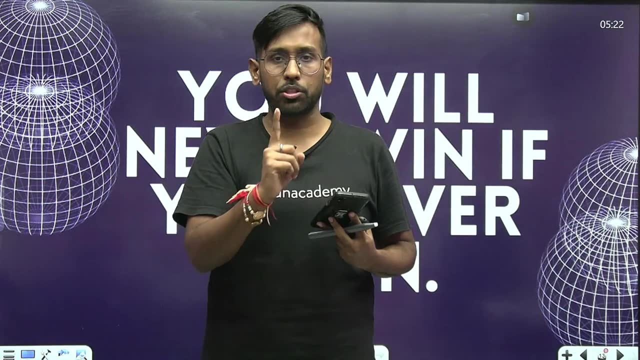 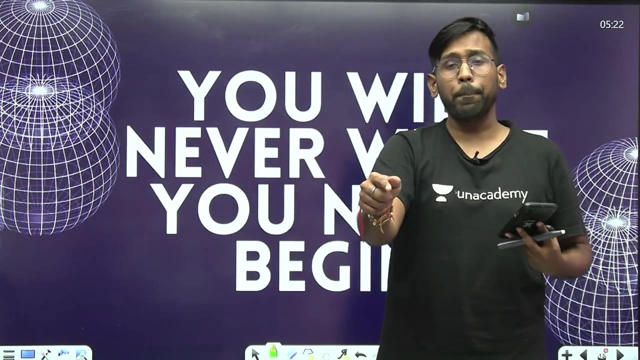 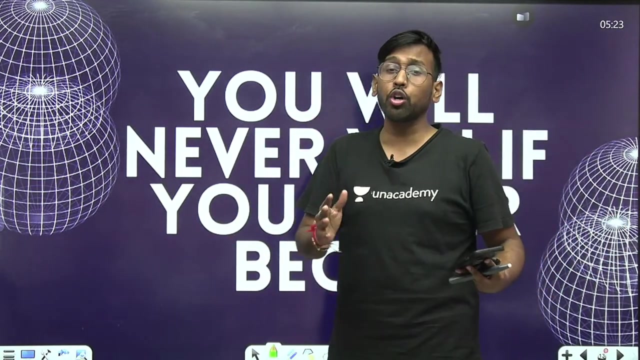 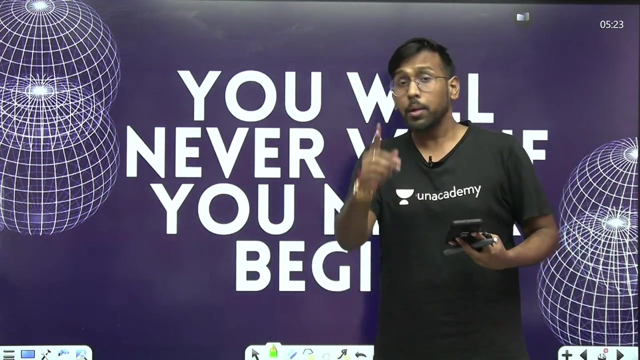 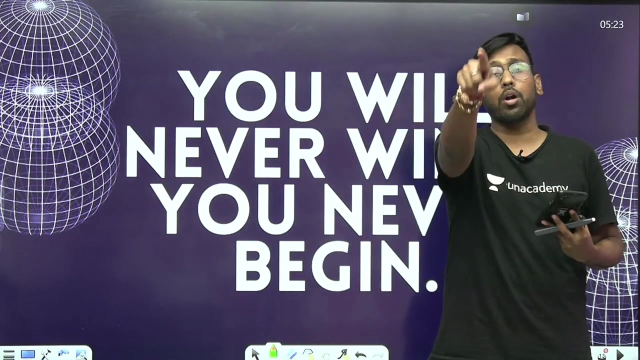 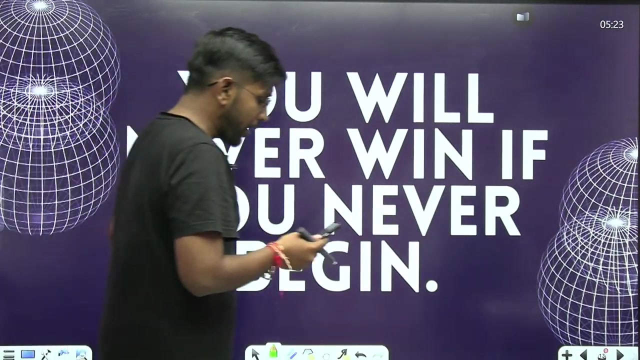 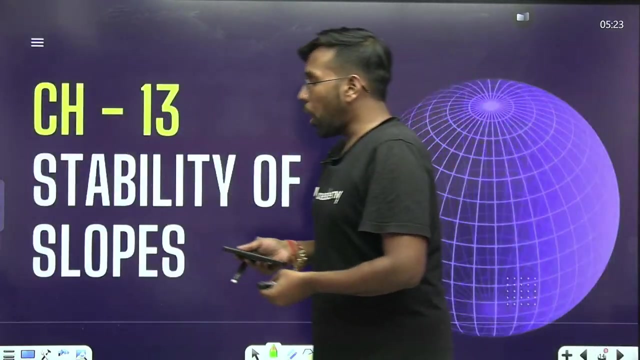 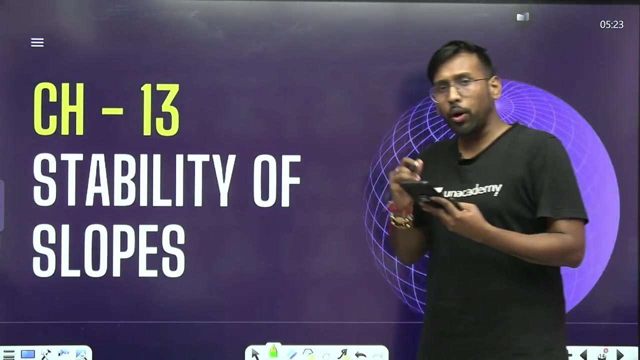 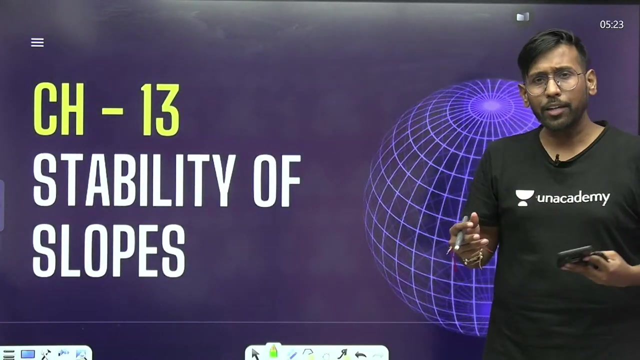 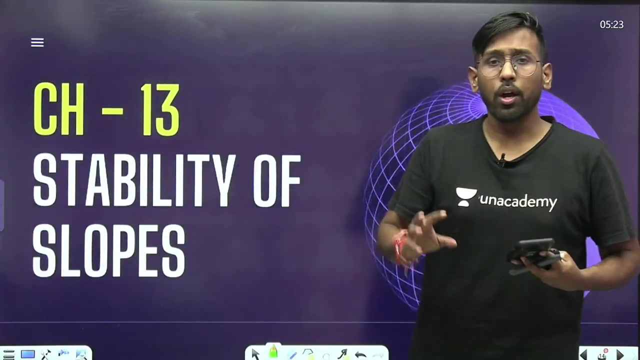 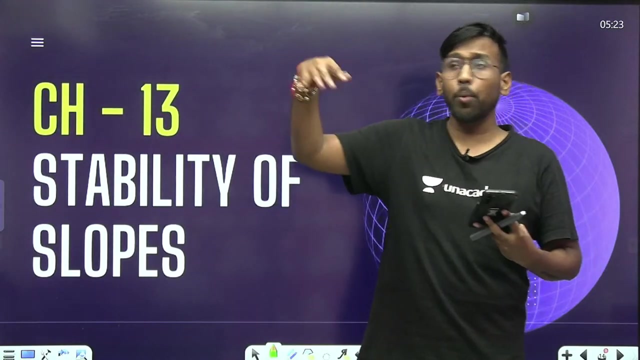 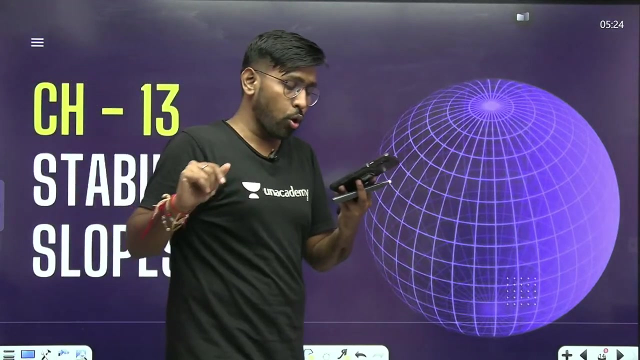 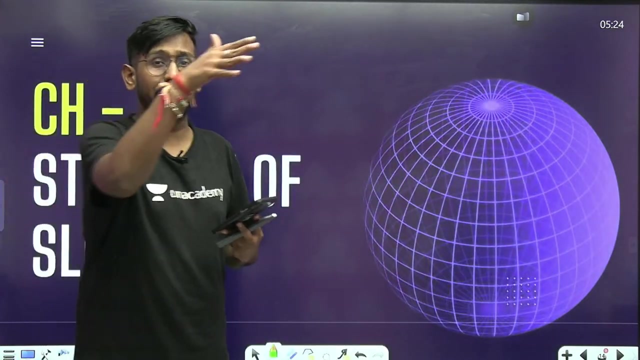 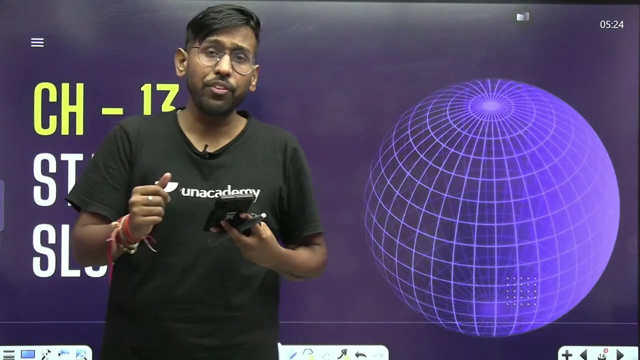 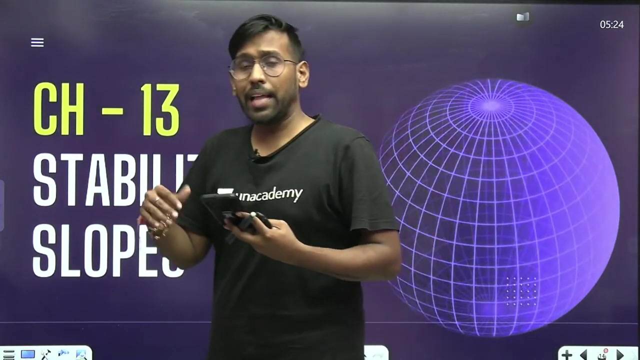 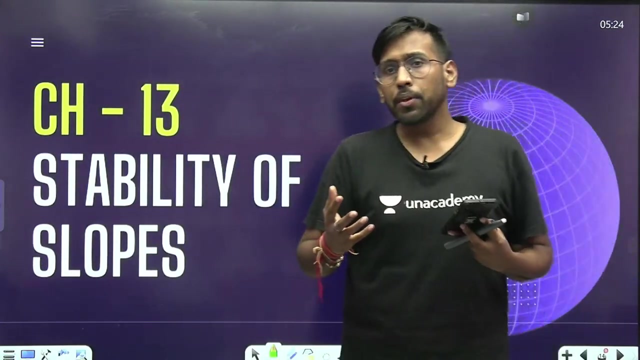 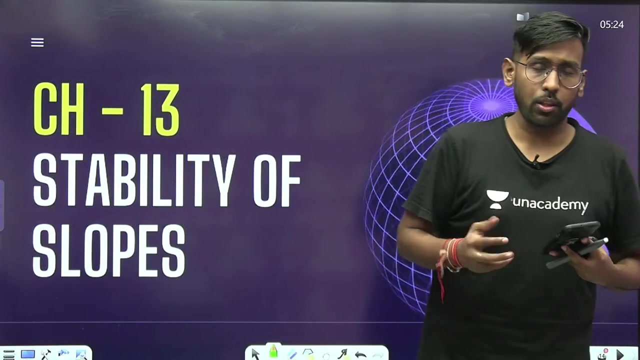 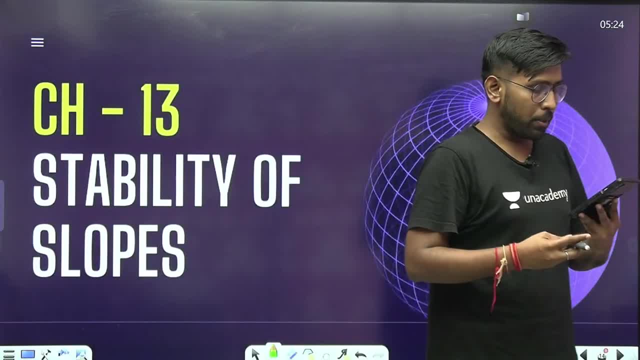 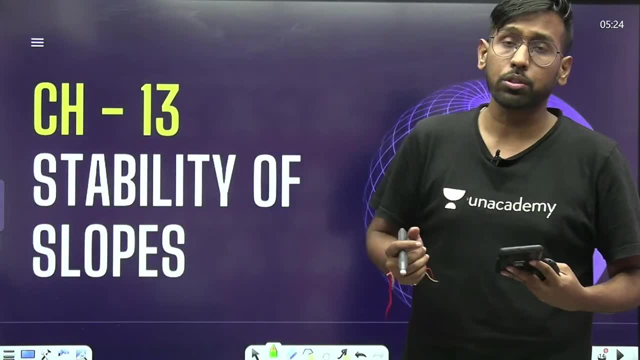 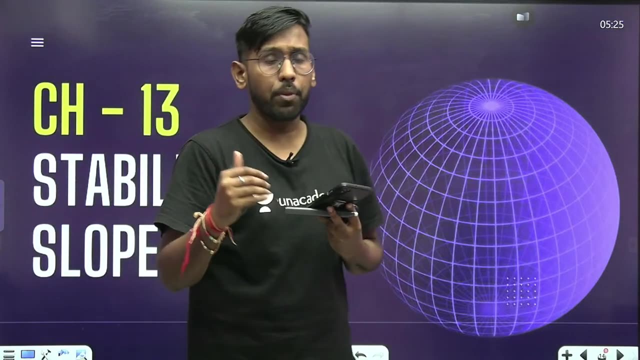 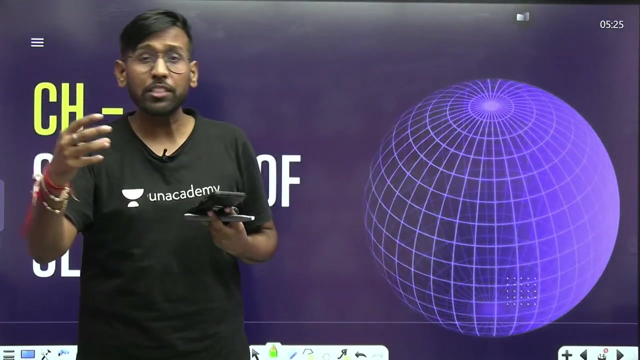 Which forces will be used. It may be gravity force. it may be the sudden drawdown of water table. What happened to the water table? It suddenly came down. So what happened? Effective stress increased, due to which it can slide down. It may be your seepage force. Water is seeping. It is a seepage force. It may be due to seepage force. 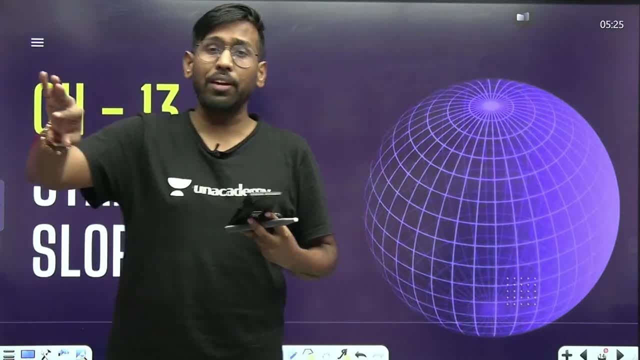 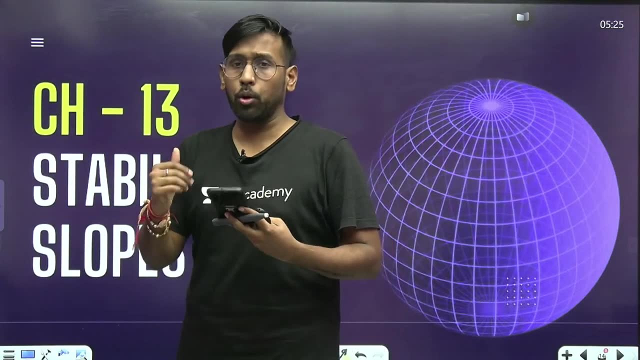 What else can happen? You are doing the excavation near the slope. What are you doing the excavation? You are doing the excavation near the slope. It can be seen there. It may be due to soil erosion. It may be due to earthquake, loading. 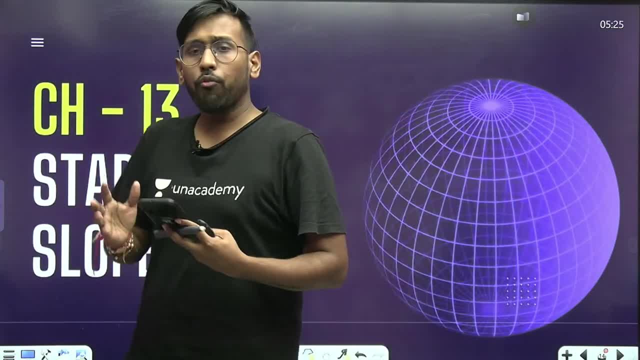 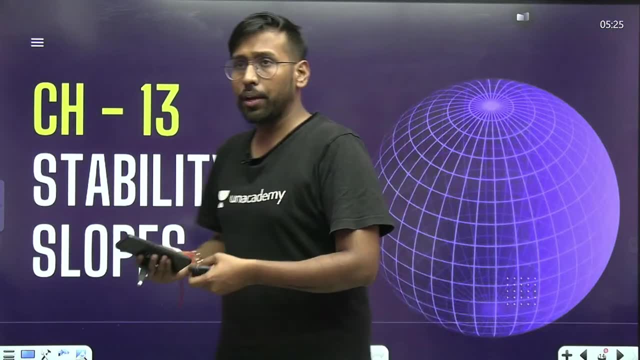 What is earthquake loading? It may be due to earthquake loading, So there are various reasons for the various forces that can act for the failure of the slope. Is it clear? Is it clear? Okay, If the water table comes down, the effective stress will increase. It will not decrease. 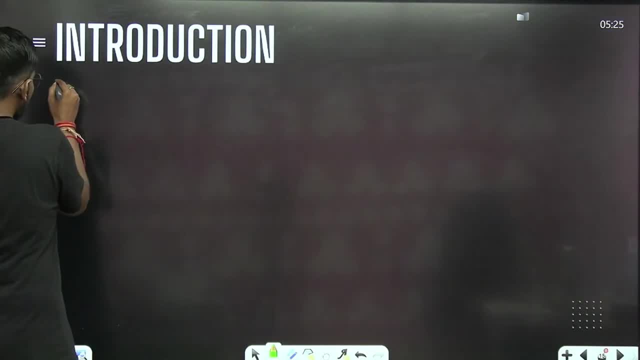 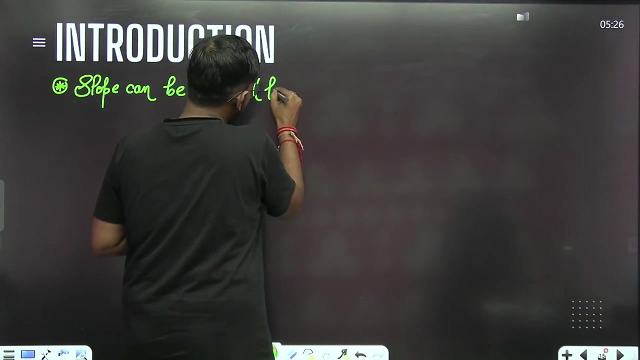 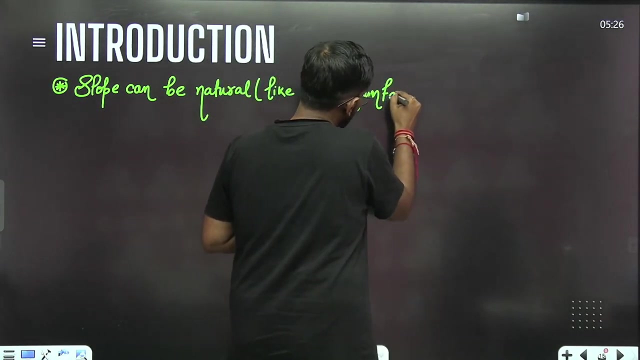 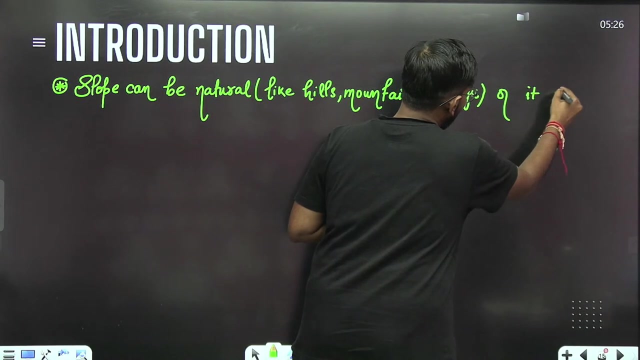 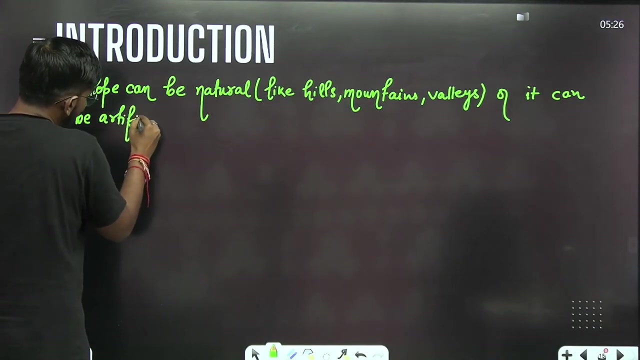 So what are we writing here, my friends? The first point: Slope can be natural. Natural, Like hills, Hills, Mountains, Mountains, Valleys, Right- Or it can be artificial. It can be artificial, It can be artificial. 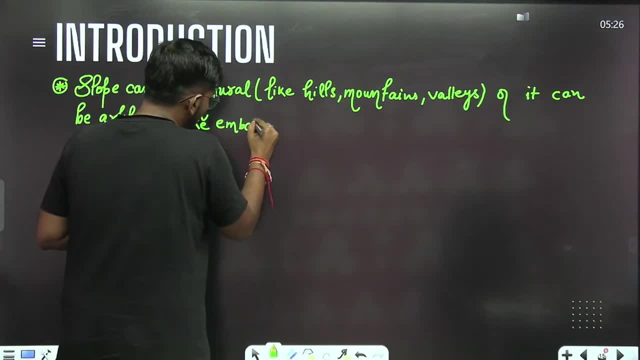 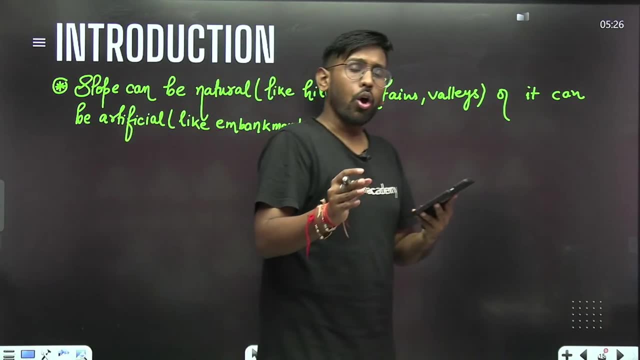 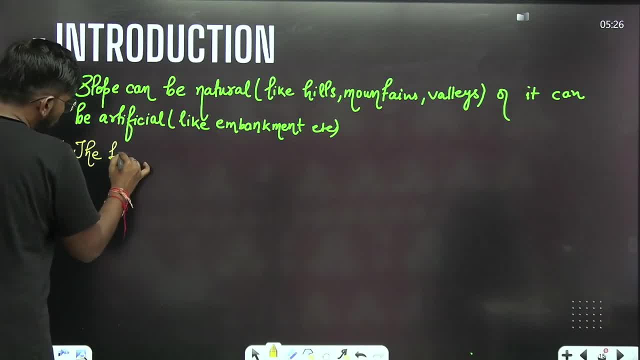 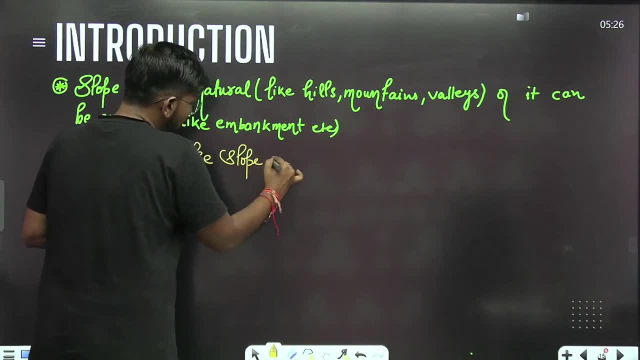 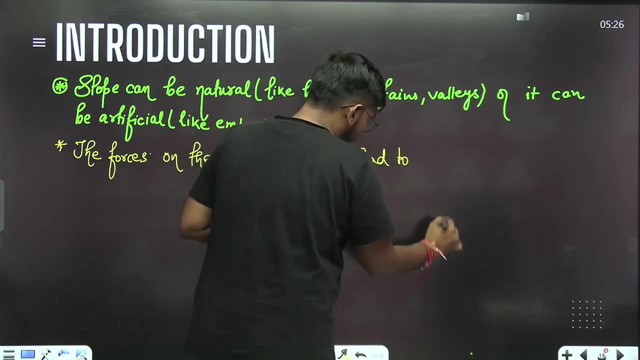 The forces, Forces On the slope, On the slope, Which can Which can Lead To its failure. Yeah, Forces acting on the slope, On the slope Which can lead to its failure, Which can lead to its failure. 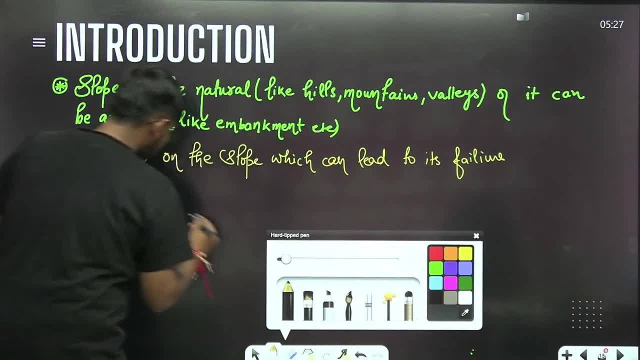 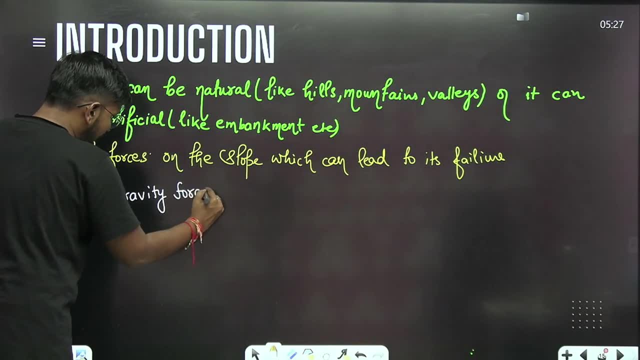 What can happen? What can happen? Yes, It can be gravity force Because of gravity, Because of its own weight, Gravity force. Second Seepage force. Seepage force, Seepage force. It can be earthquake force. 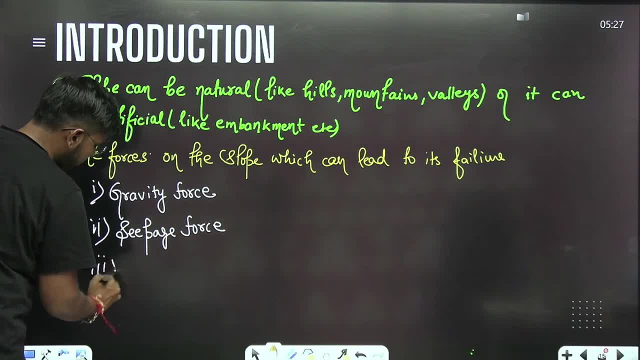 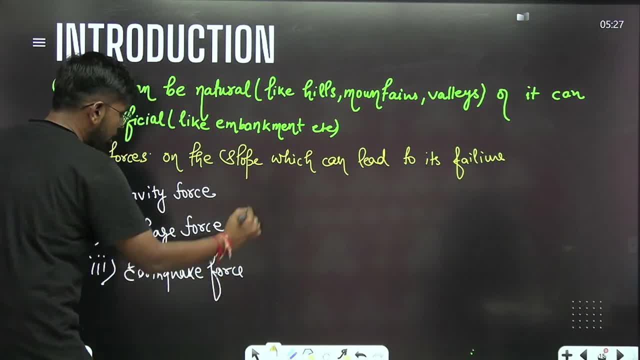 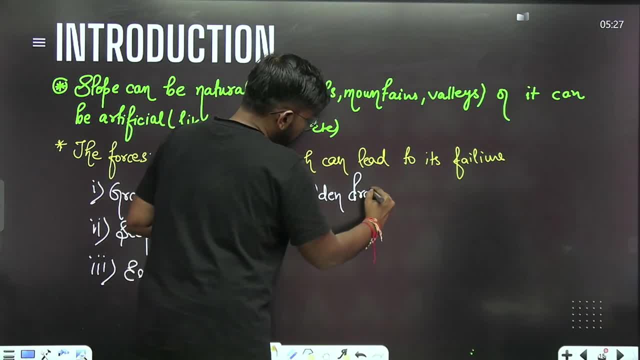 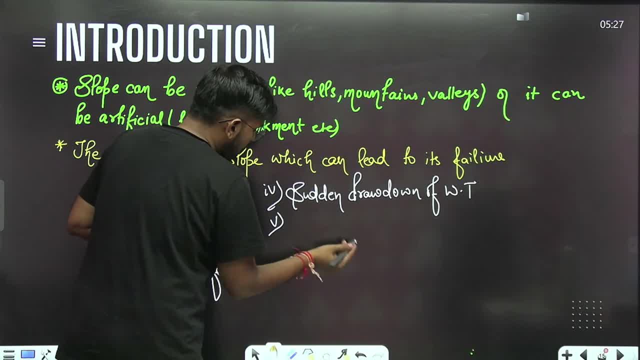 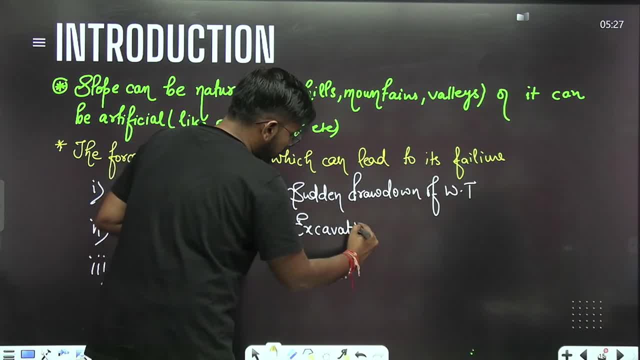 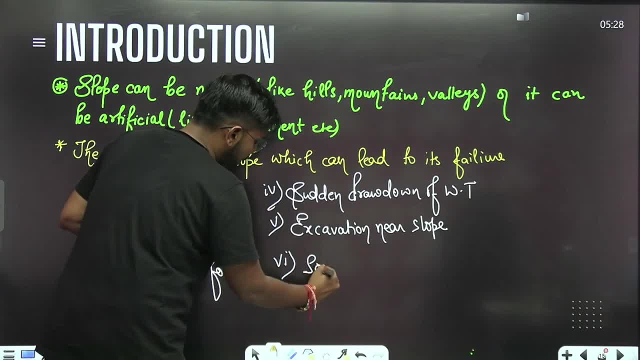 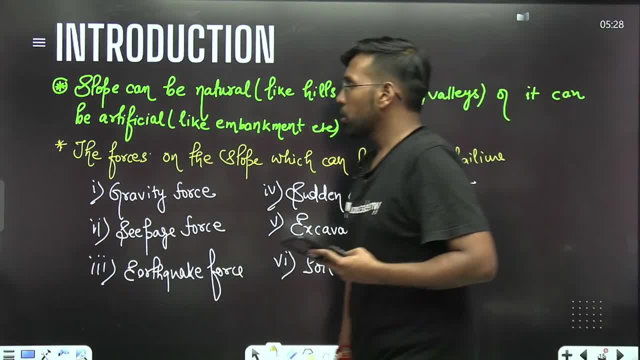 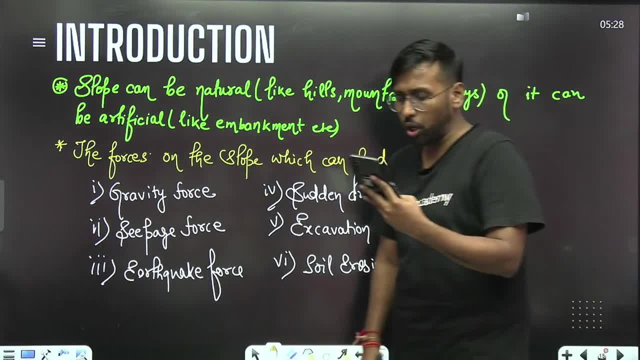 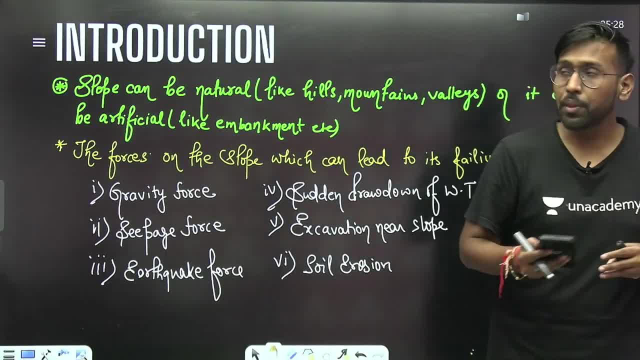 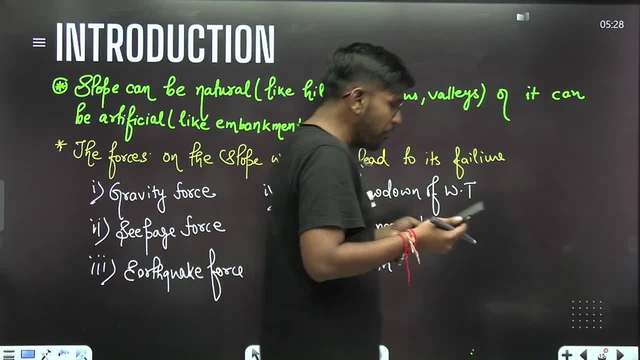 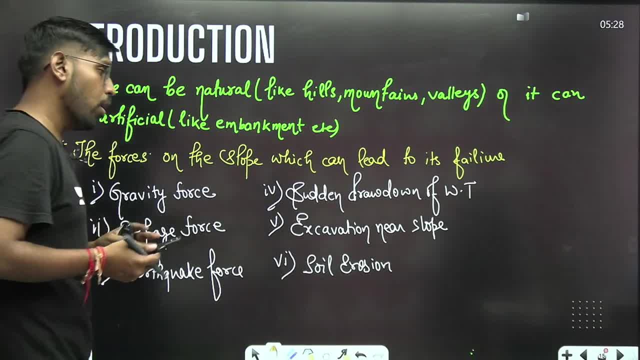 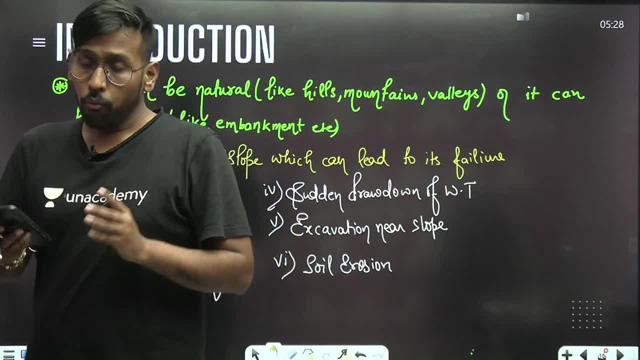 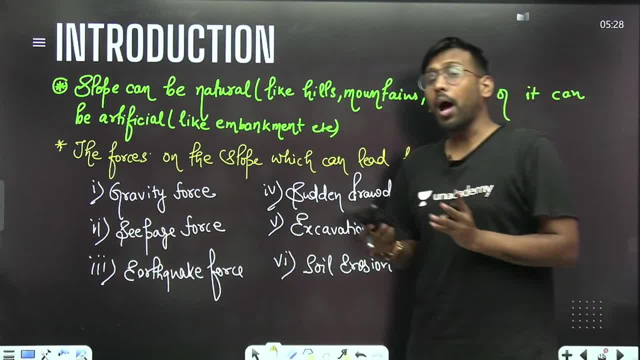 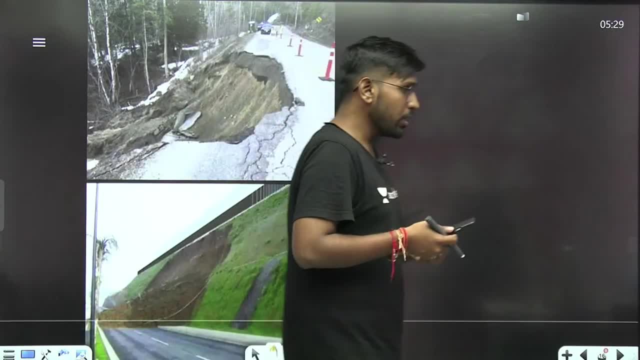 Sudden drawdown of water table. Sudden drawdown of water table means we can't leave any part for IT Kharagpur paper. so, my friends, these are certain slope failure. can you see it? can you see any failure like this? 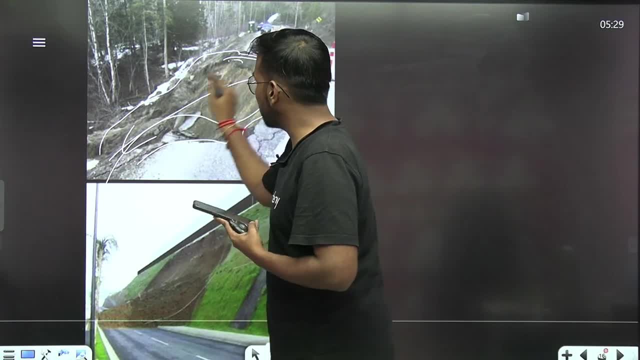 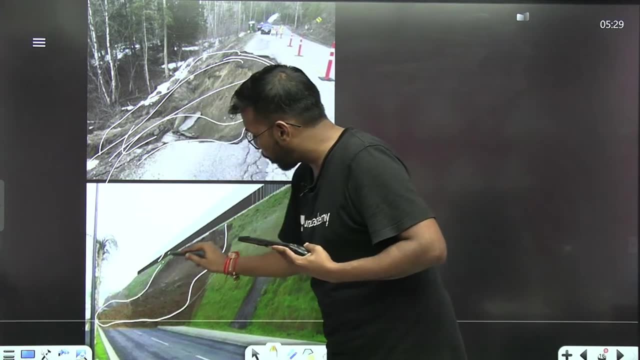 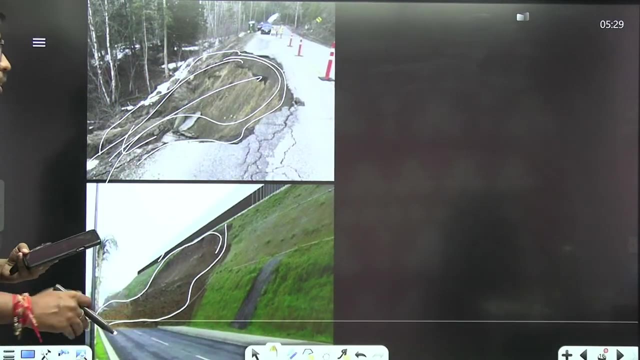 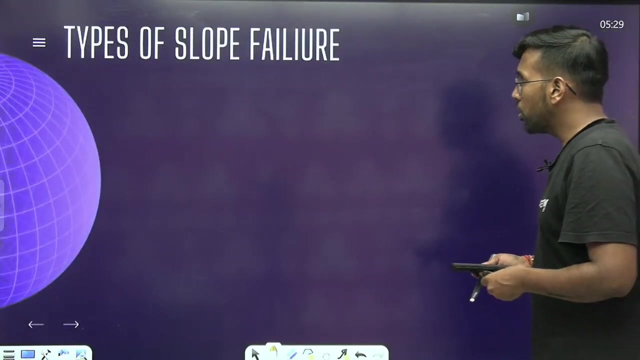 can you see? the entire soil mass gets slide down. see here, this was the road and this was the normal slope. so this entire soil mass came on the road. can you see it? yes, clear point. these are the slope failure. so, my friends, if we talk about slope rather than types of soil failure, slope failure, 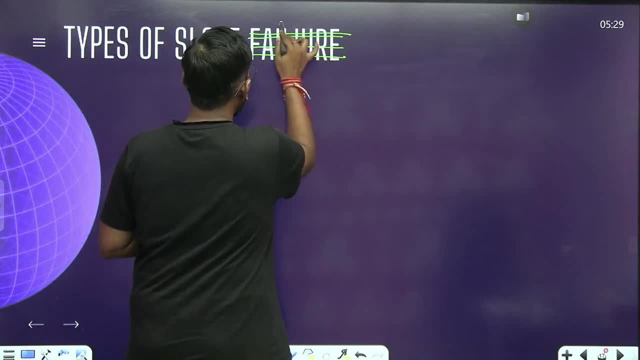 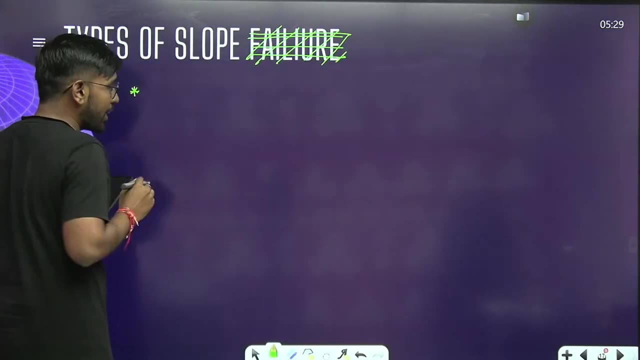 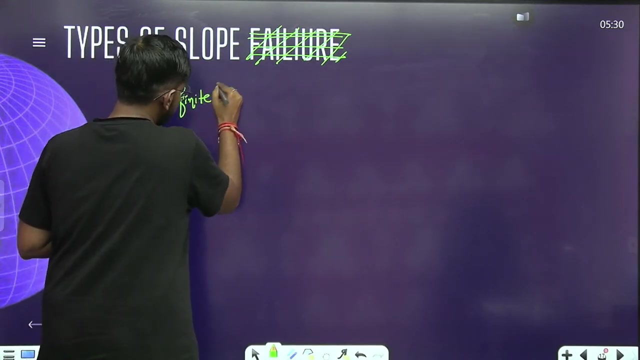 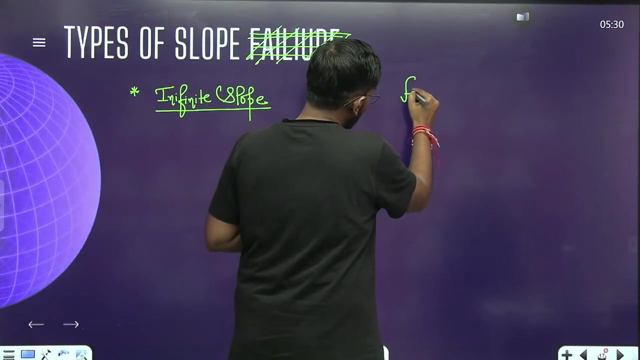 we are going to discuss types of slope. how many types of slope can there be? see, slope are basically classified in two parts. slope is basically classified in two parts. one is infinite slope and the other is finite slope. there are two types of slope, my friends. 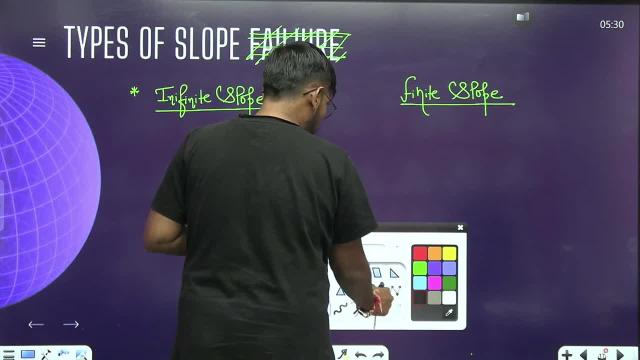 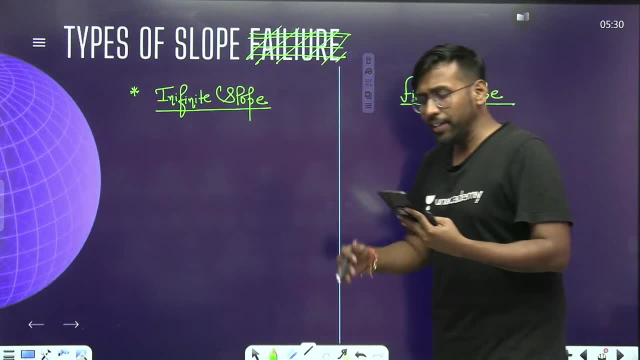 one is infinite slope and the other is finite slope. there are two types of slope, my friends. now, can anyone tell me what is the difference between the two? can anyone tell me what is the difference between the two? infinite slope? what do you understand by infinite slope? 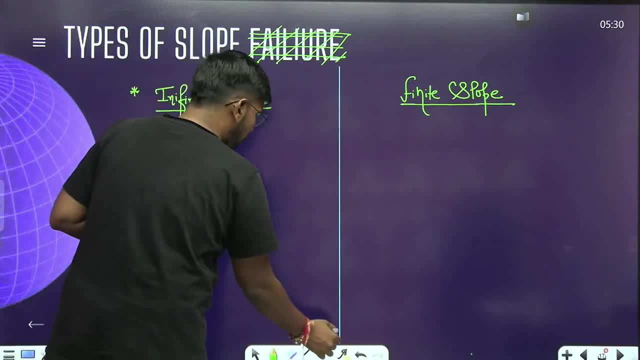 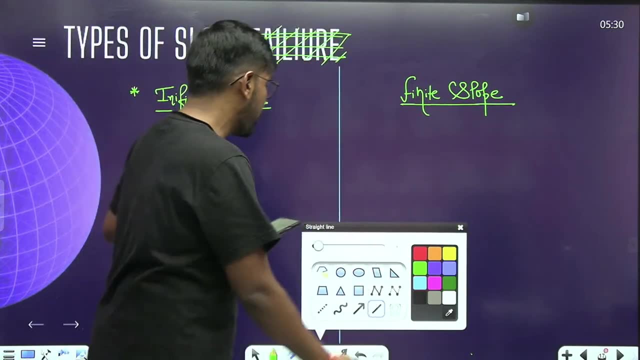 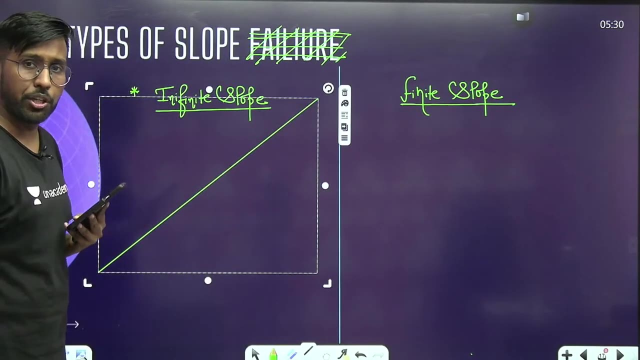 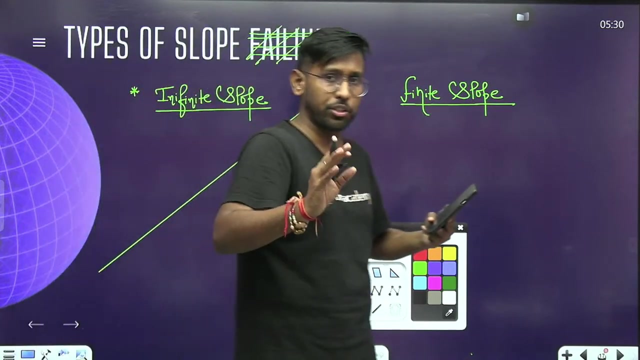 what do you understand by infinite slope? infinite slope means that there is no end to it. it is extended up to infinite dimension. it has no limitation. is it clear? no limitation. it has no limitation, not bounded. it does not have any upper or lower boundary. there is no limitation. 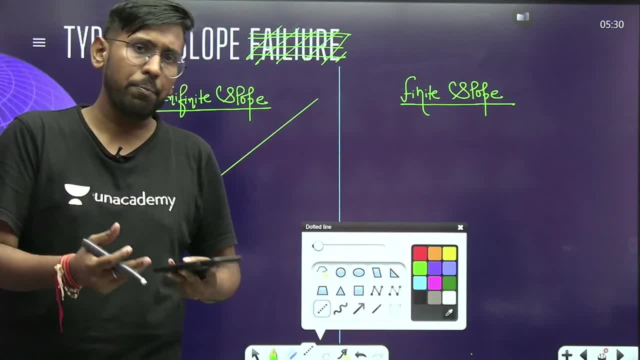 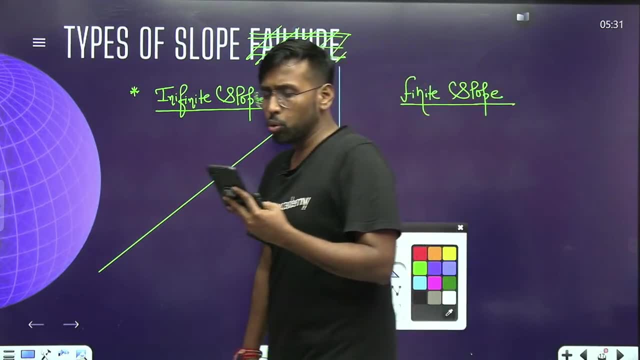 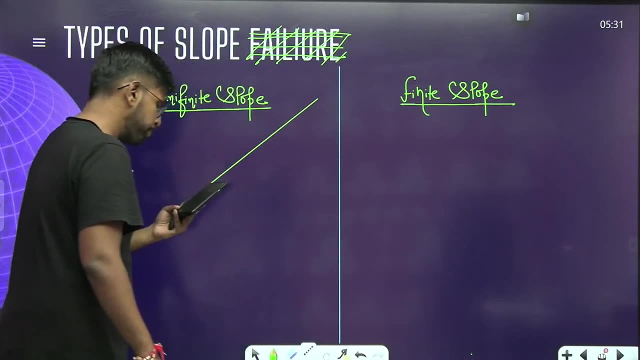 generally, the hills or the mountains are finite or infinite. can you tell me quickly: are they finite or infinite? those are finite or infinite. can you tell me quickly, my friends, are your mountains finite or infinite? those are infinite, those are infinite. 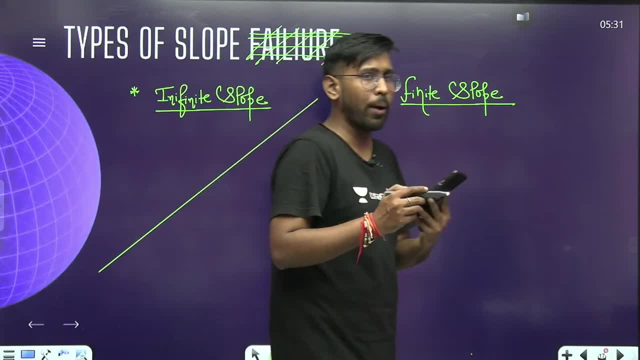 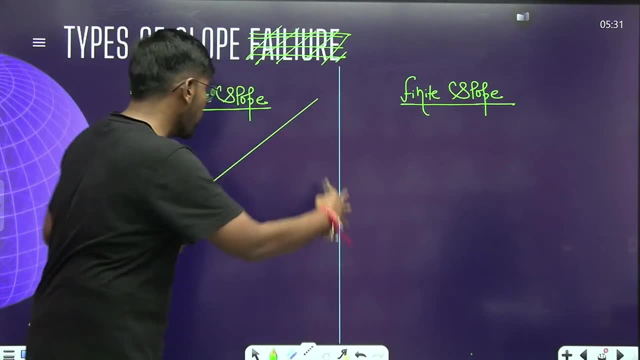 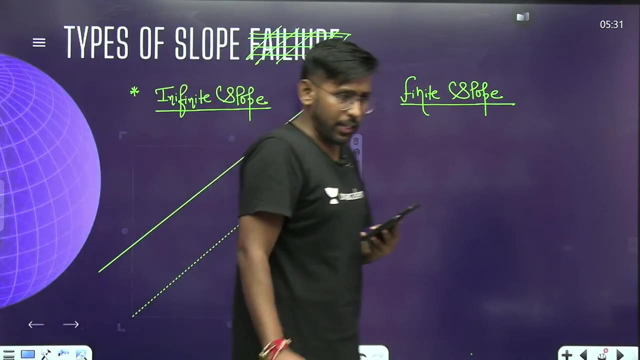 those are infinite. ok, now, whenever you see a failure, how will you see a failure? you will see a failure that the land mass is sliding, the whole land mass, about a plane. what is it doing about a plane? it is sliding down. ok, this is called landslide. 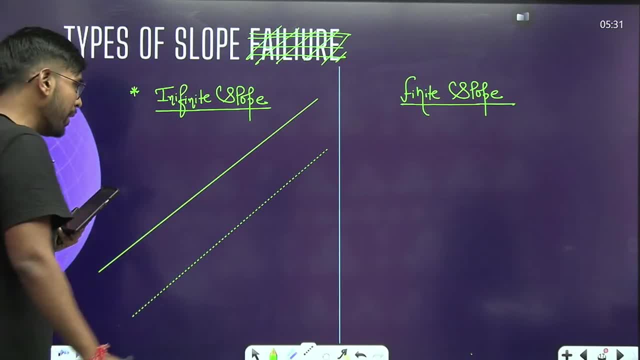 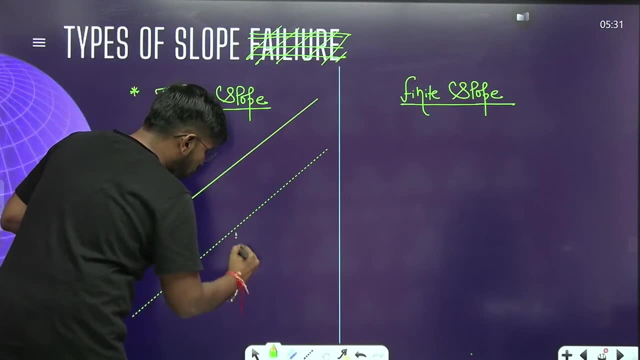 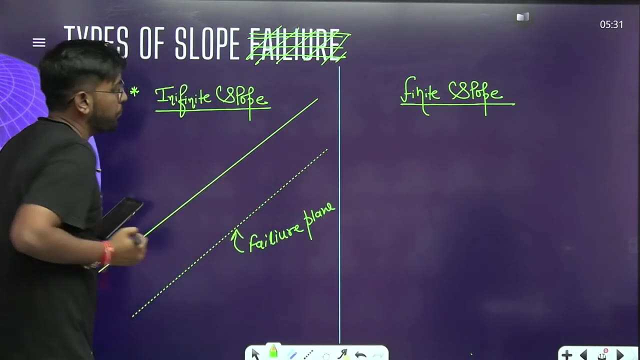 what do you call this? landslide, yes or no? what is happening here? is that the whole soil about a plane. it is going to fail, is it clear? so what has happened here? failure plane, failure plane. this is the failure plane. this has become your failure plane. 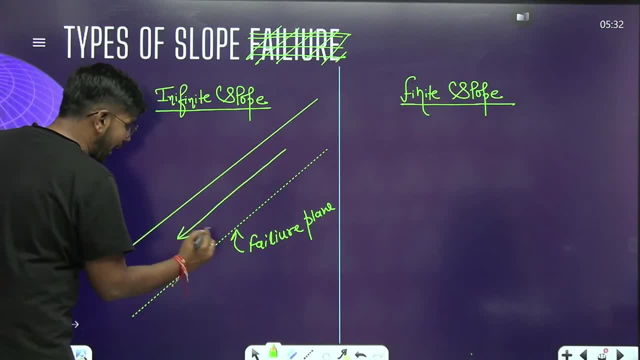 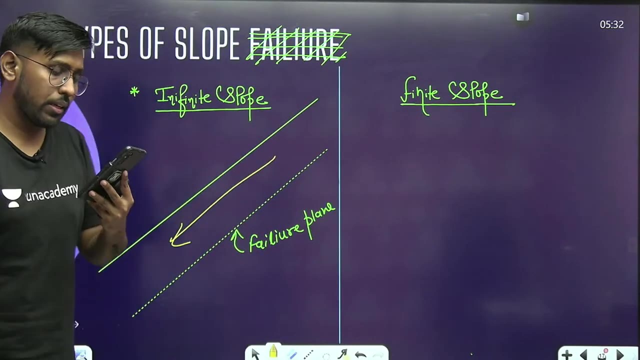 so what is it seeing? the entire mass is sliding down. the entire mass of soil is sliding down. the entire mass of soil is sliding down about this layer. what has happened to the entire mass above this? it has slided. this is called landslide, yes or no? 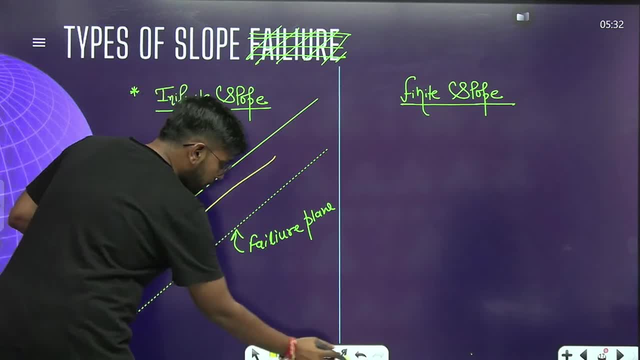 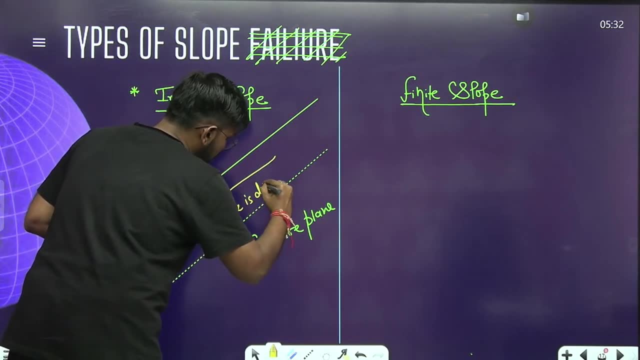 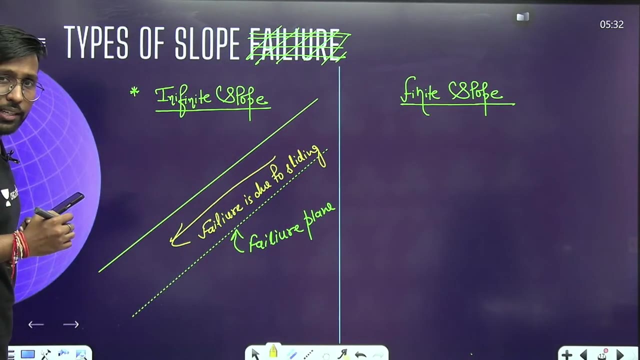 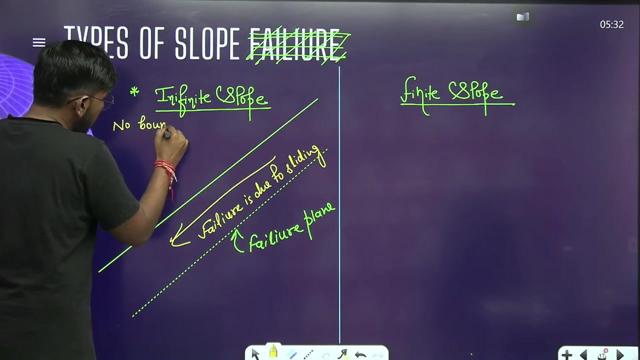 so, my friends, the failure here, the failure here failure is due to, is due to sliding, sliding, ok. failure is due to sliding, ok. what is the infinite slope here? no boundary, boundary, no boundary. there will be no boundary, there will be no boundary, there is no boundary. 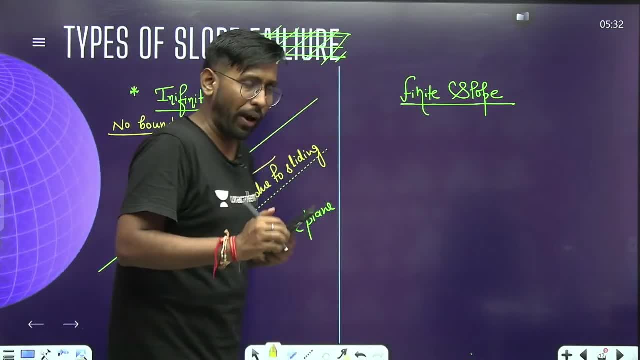 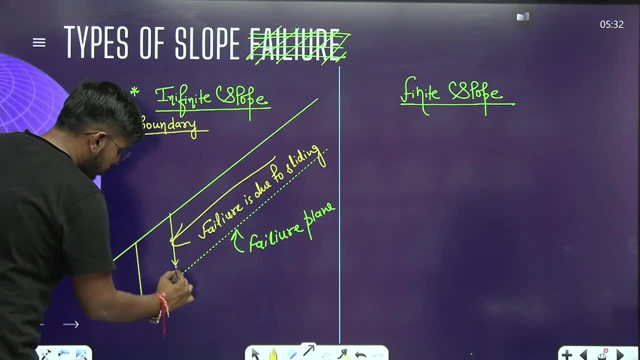 the failure is due to sliding. the failure is due to sliding. now, my friends, here one point is considered in infinite slope: that at all the depths means if you are talking here, ok, see here here, what do you say for infinite slope? that from the surface. if you talk on z depth. 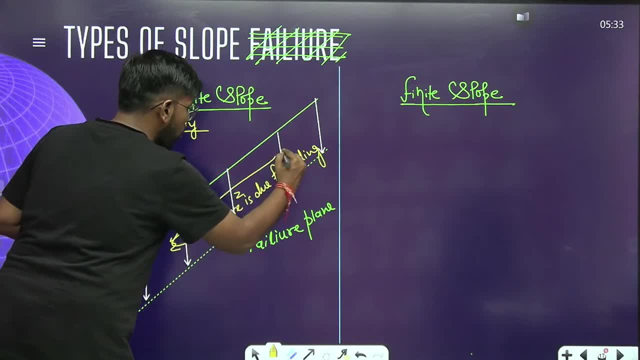 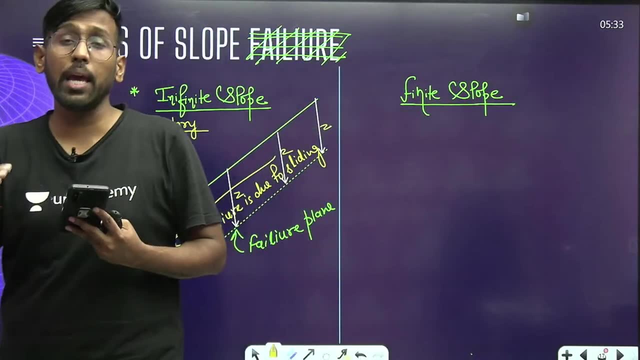 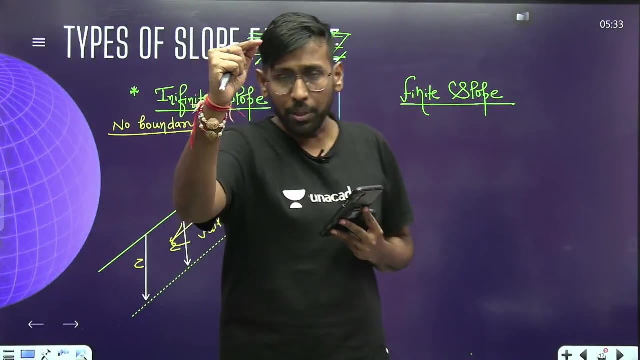 from the surface. if you talk on z depth, so at that z depth, from all the points, the property will be. what will be same? the property is assumed to be same. that means at a depth, at a certain depth from the ground surface, at all the points, the properties are assumed to be same. 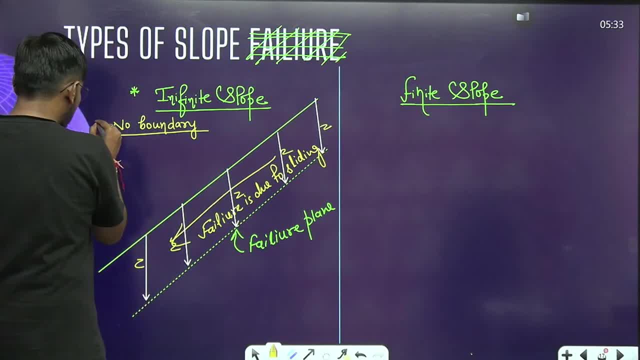 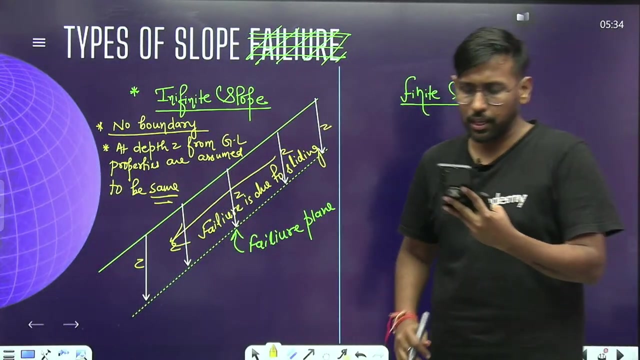 is this point clear? properties are assumed to be same at a depth z. at a depth z from ground level, properties, properties are assumed to be, are assumed to be same. this is called infinite slope. so, practically, tell me, can such a slope exist? practically, can such a slope exist? 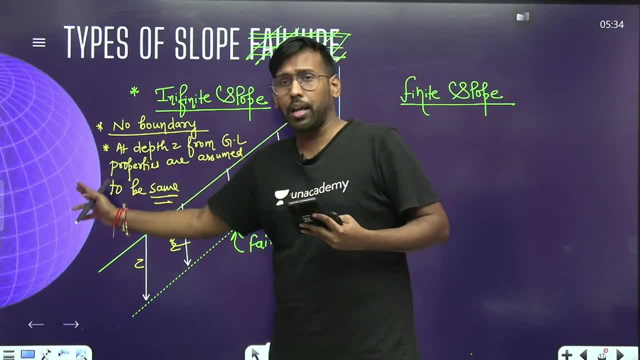 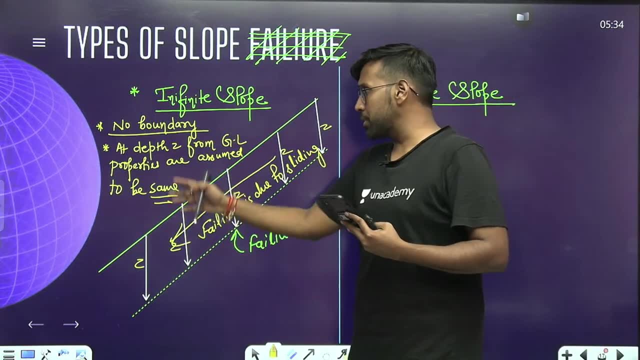 if we talk practically, if we talk about this property. so can such a slope exist? tell me yes or no, say my friends. practically at a depth z from the ground level. if we say that the property is same at all points, can such a slope exist? no, it does not. 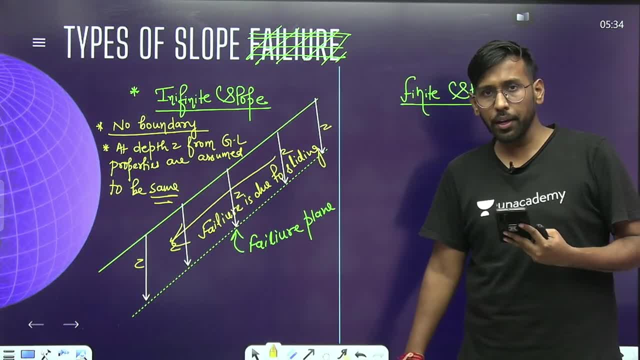 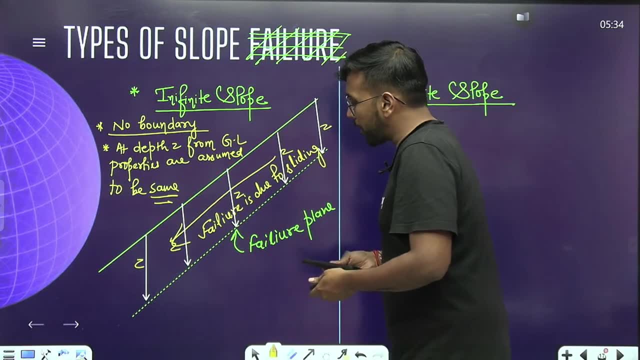 ok, so practically not possible, but we will accept. ok, we will accept. that is why, when you see here, when you are looking at the cut, then what is the cut? what is it looking like? is it straight? is this cut straight? just check, is this cut straight, is it straight? 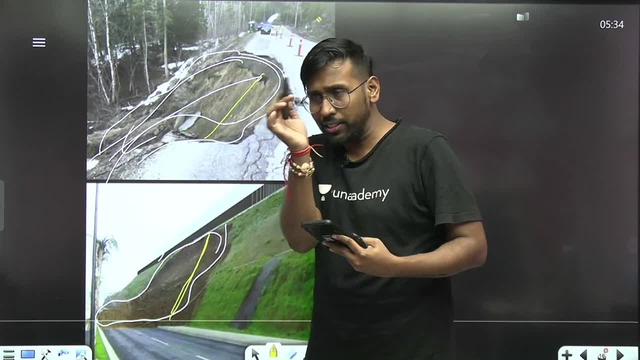 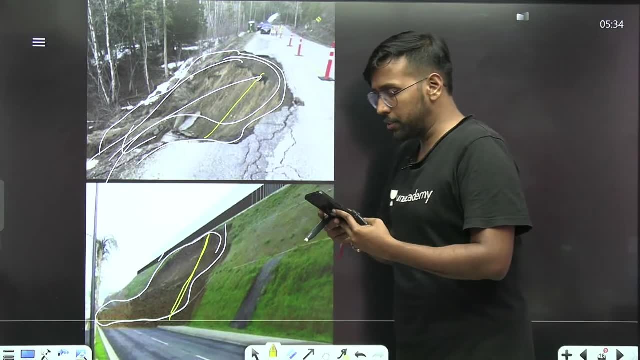 what is this cut? what is this cut? straight hoga nahi, thoda sa variation hoga right, but we are assuming it to be a plane that is ek layer ke about ye fail kar raha hai. is it clear, ye point? clear hua sabko. 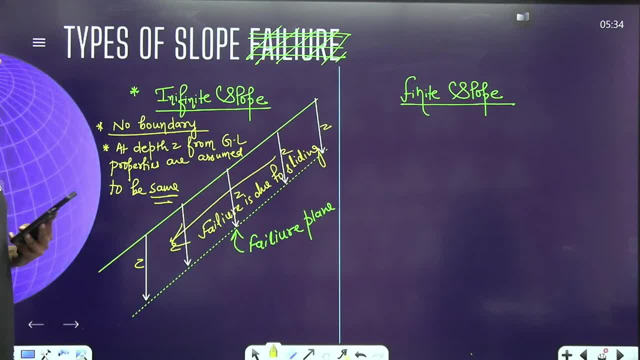 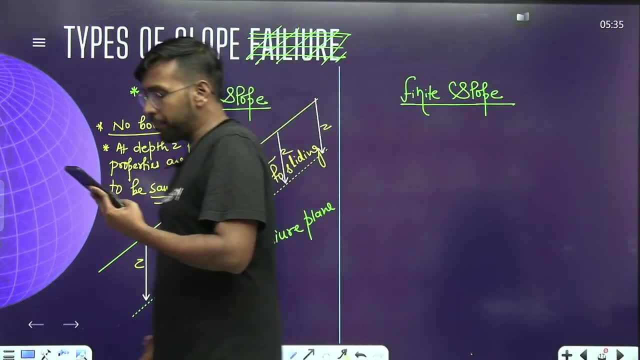 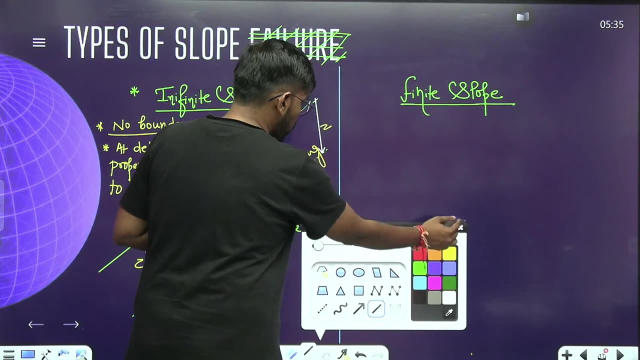 bolo mere dost to. infinite slope ka basic, samajh me aaya. infinite slope ka basic, samajh me aaya. tell me yes or no. tell me yes or no. infinite slope clear, hua. tell me, my dear friend, is the infinite slope clear to all? is the infinite slope clear to all? ok, agla. 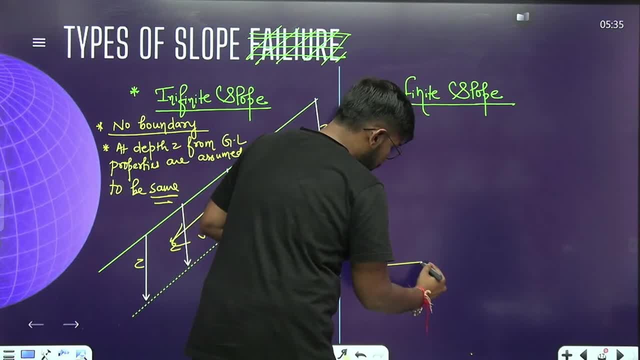 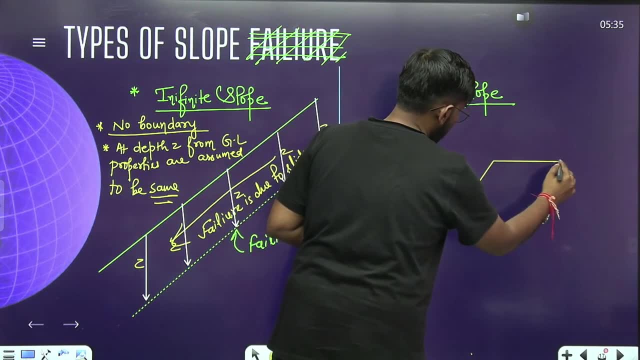 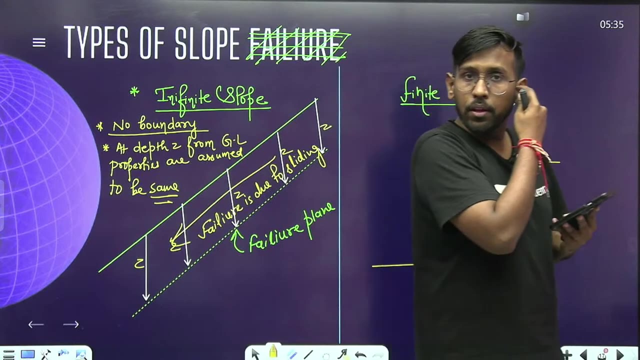 baat karte, mere dost, hum log finite slope agla baat karte hum log finite slope. acha, ek baat puche hai. kitne log pehle ye padhe ho, kitne log pehle ye sab topic padhe ho. 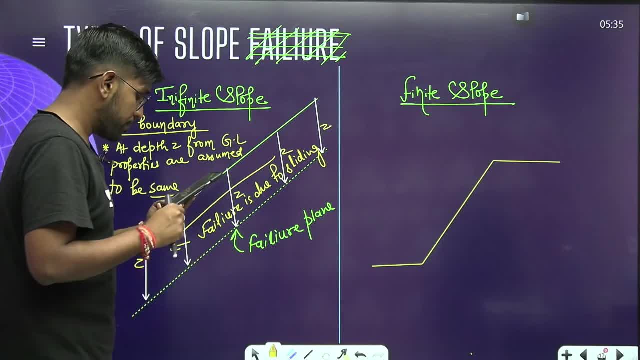 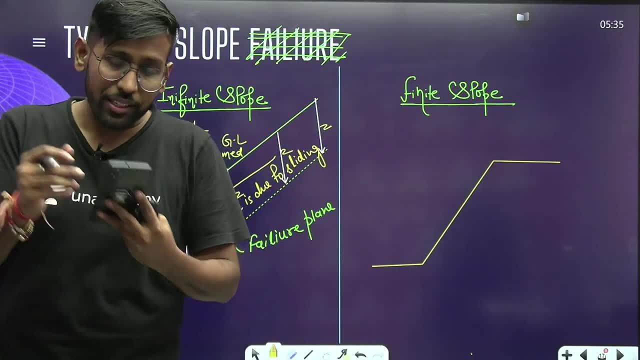 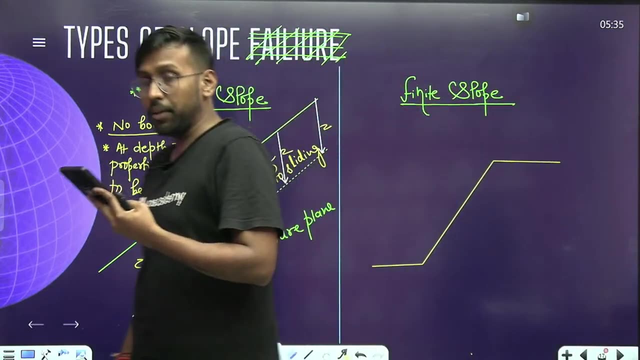 last year. mere hi se hi padhe hoge kitne log pehle ye sab topic padhe ho. Because today we are going to tell you something that you have never seen, which you will not find in any book. you will not find even if you look for it. so today we are going to 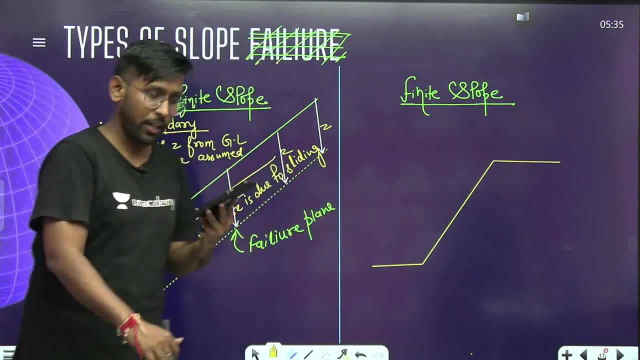 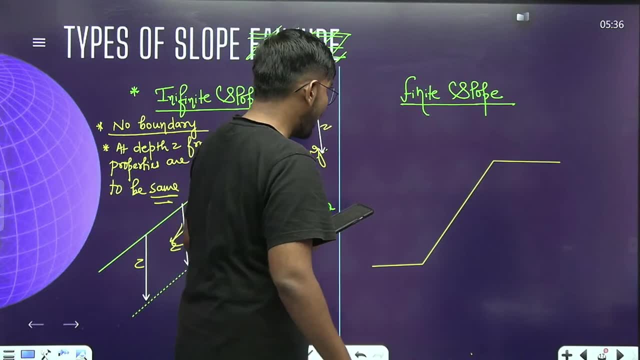 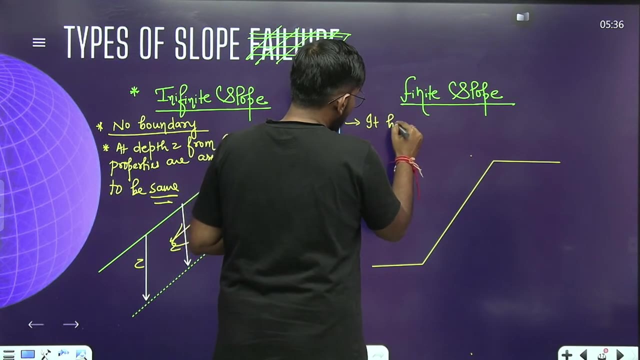 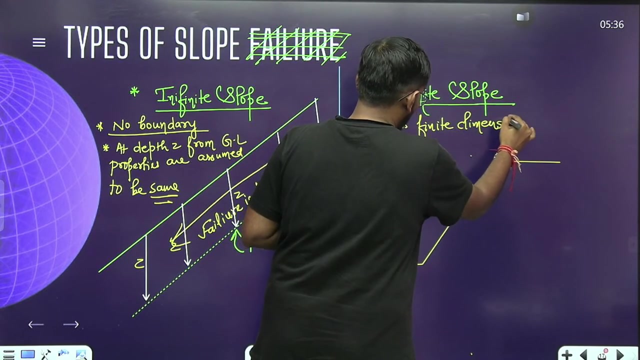 tell you something like this: today's video has become very important. okay, let's go. okay, finite slope. so if we talk about finite slope, so it has finite dimension. finite dimension have upper and lower boundary. so now, what will happen here? what will happen? 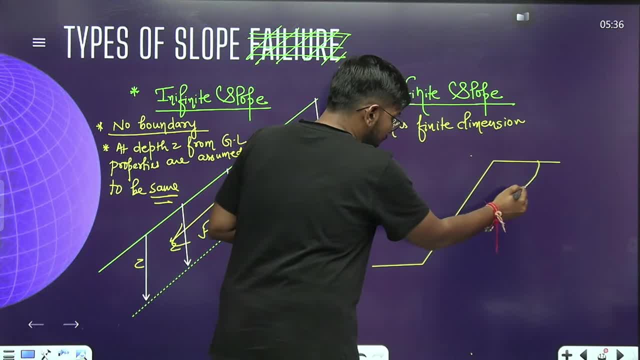 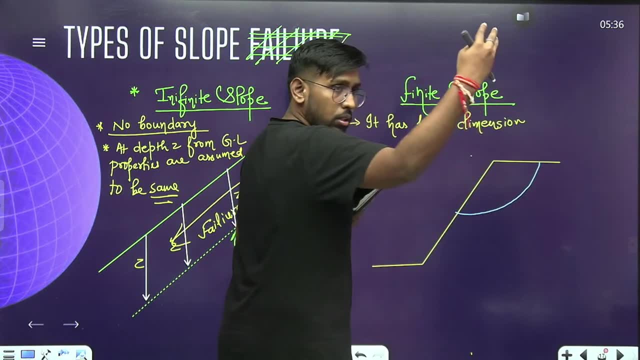 here that the soil surface, if we talk about failure plane, so it is not. it is not. it will not be good. Now, what will happen here? The soil, the soil is going to roll out, the soil is going to roll out and it will go out. 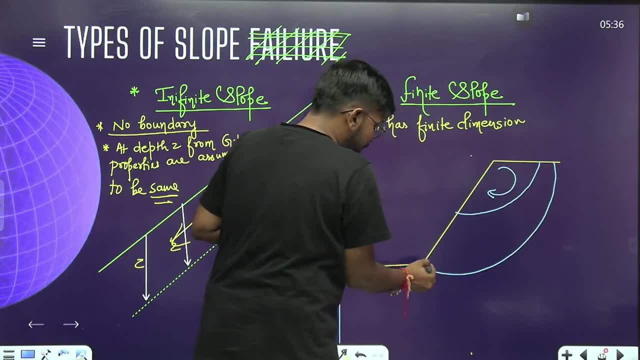 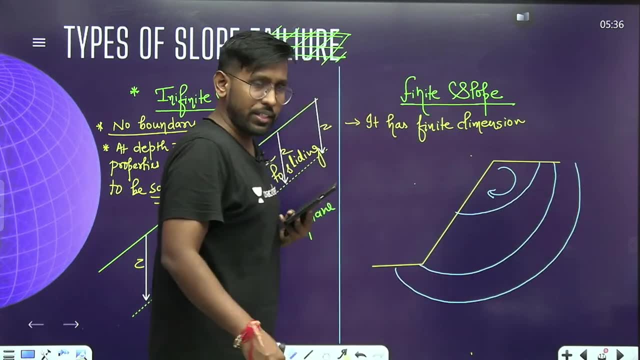 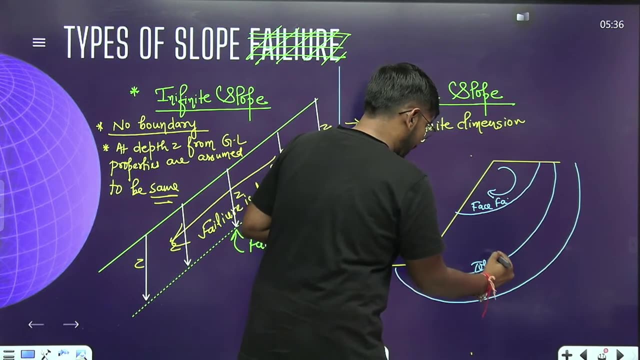 so this part is cut and excreted, or failure can be made in this way that this whole part is cartoon and it can fail like this, also in different names, given this is known as what we called it: face failure, face failure. what do we call it? priority toes failure. 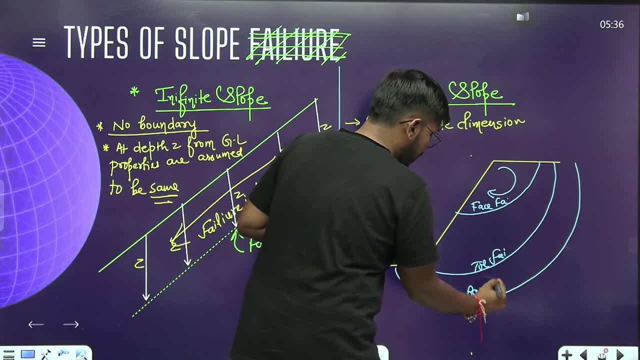 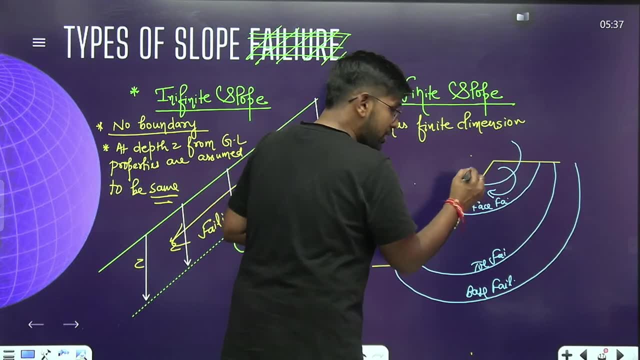 this. we'll do this, don't worry. and this is called base failure, and we call this a base failure. so please remember this. now we are done. So, my friends, face fillet, toe fillet, base fillet. what will happen here? there is not sliding, but rolling of the landmass. there is not sliding. 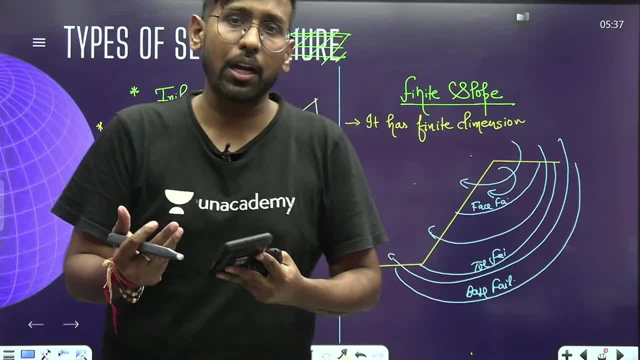 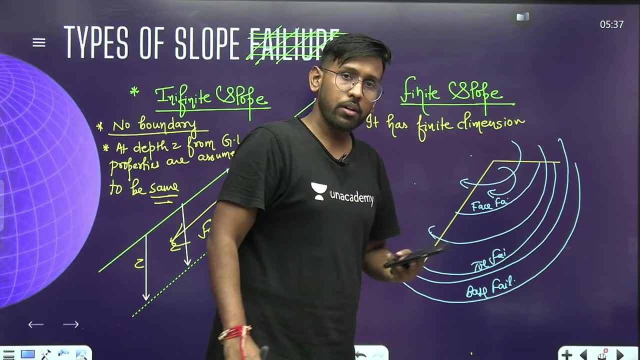 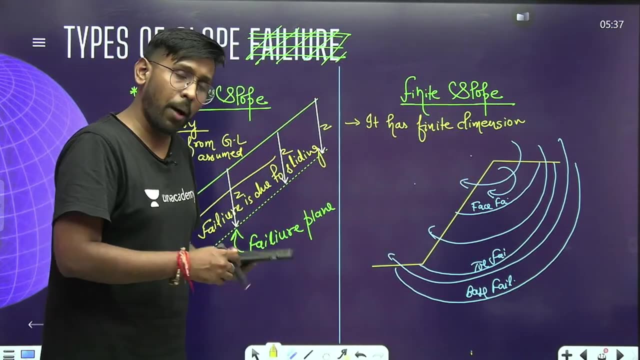 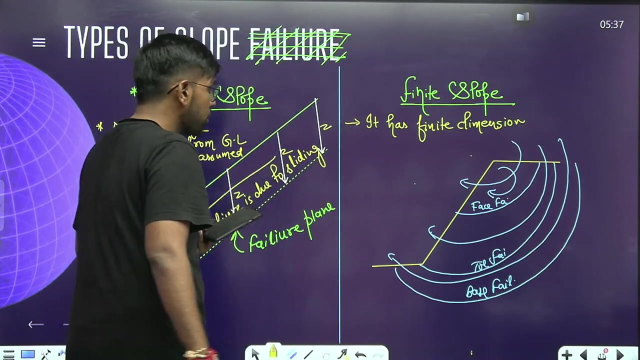 And the failure surface can be circular or it can be spiral. Soil will fail due to shear. only Now, when and what will happen, we will read. This is the chapter only Name is finite and infinite slope. So when and what will happen? we will tell you when that topic will come, Don't worry. 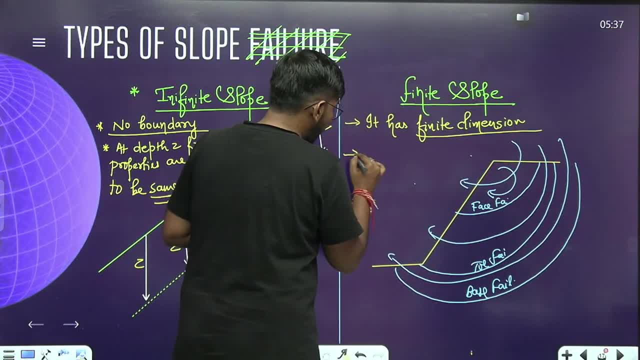 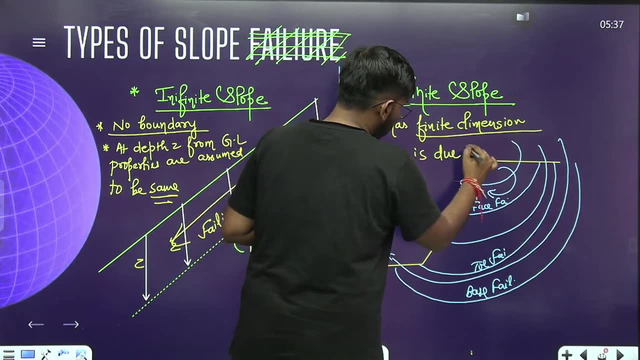 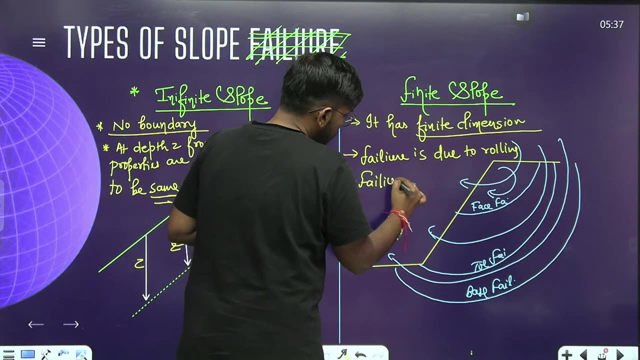 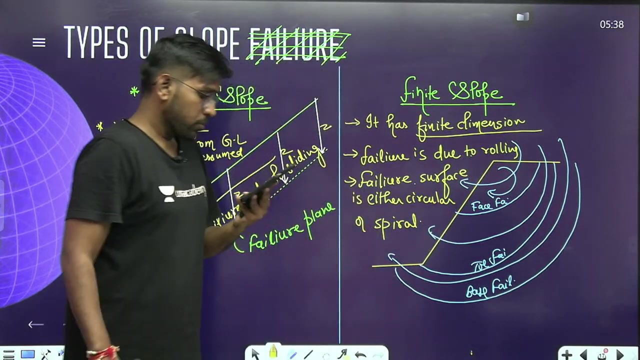 It has finite dimension. What is said here? Failure is due to rolling. Failure surface, Failure surface. Failure surface is either circular or spiral Or spiral. Is it clear to all? Is it clear to all? Tell me, my friends, This point is clear. So infinite and finite slope. 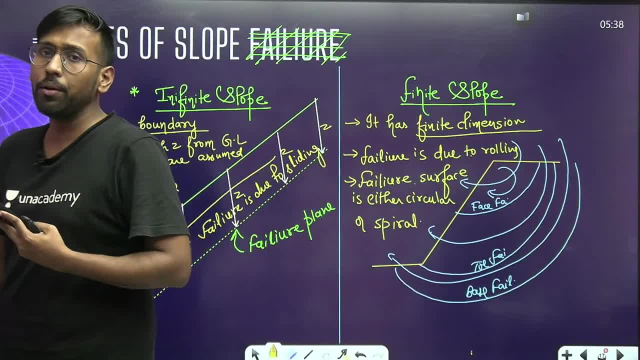 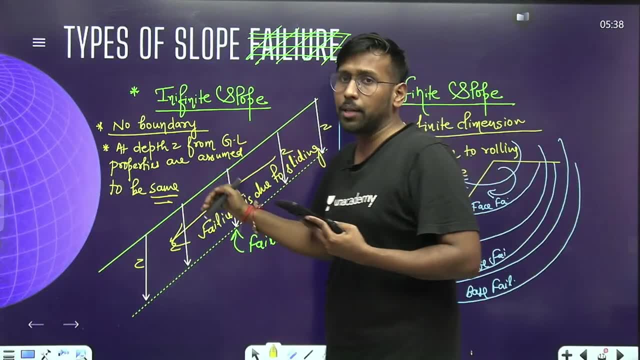 Infinite and finite slope. Infinite slope, no boundary. There is no boundary in infinite slope. There will be boundary in finite slope At a certain depth. jet at every point. what will be your property? Same. It is not like that in finite slope. 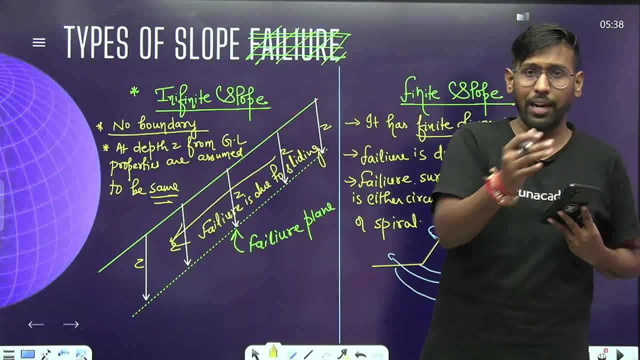 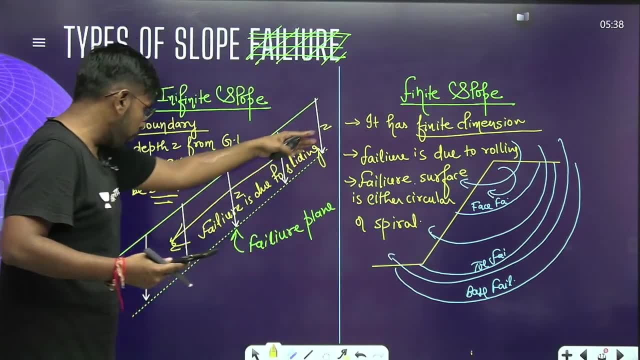 In the infinite slope, the failure is due to the sliding of the landmass. In the finite slope, it is due to the rolling of the landmass Here failure. surface will be circular or spiral. Here you will see a plane. I hope it is clear to all. 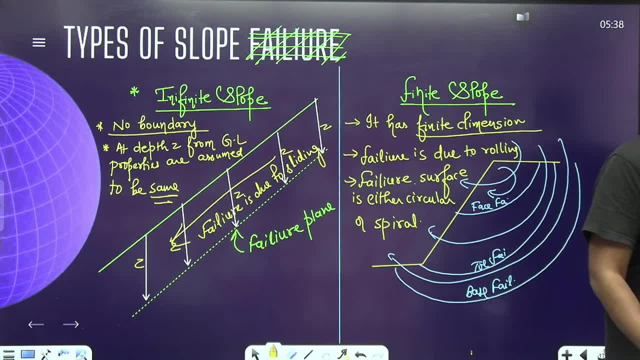 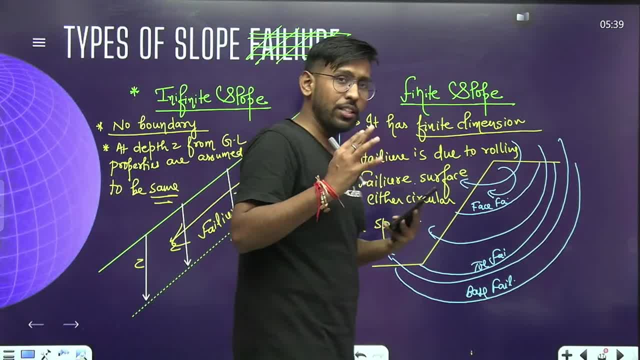 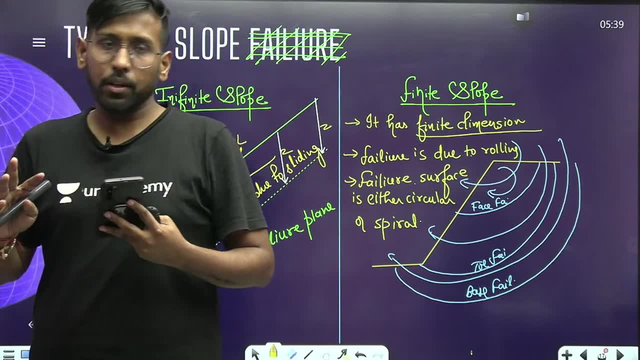 We will have fun. We need to feel, We need to lead a feeling. Without feeling, there will be no reading in condition of feeling. See, if you will read without feeling, there will be no problem. You will just read but will not enjoy. 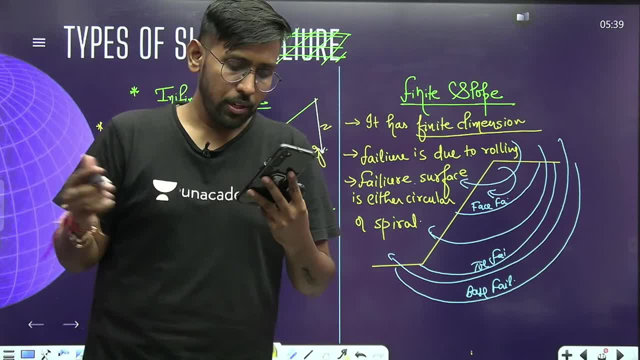 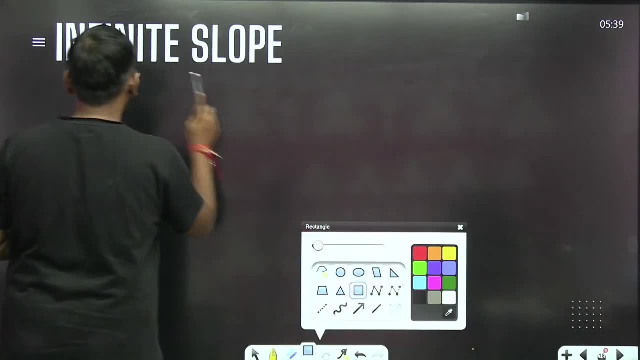 However, if you will read with an feeling, it will make the life easier. And I say first, oriented with the, I will be very much oriented with the content or with the syllabus. Okay, We will be teaching according to our syllabus. 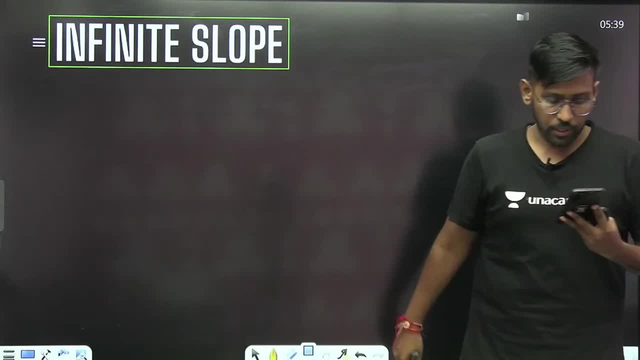 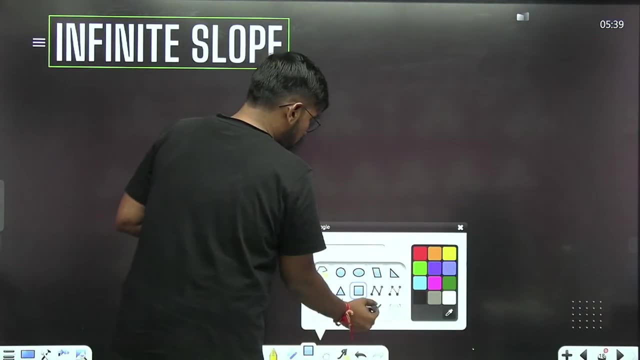 Neither more nor less. Okay, Okay, Okay, Will you see, my friend? Infinite slope. Let us look at the infinite slope. So we are starting infinite slope. You must have seen today's heading: Infinite slope. Today we have to study infinite slope. 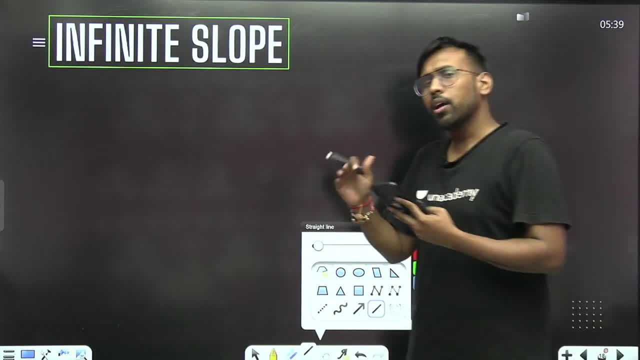 In which today it will not be completed. Tomorrow we will complete it Today. we will see the basics first. We will check the basic points first. Fine, Infinite slope, Embankment, Embankment- Do you provide embankment in Railways? 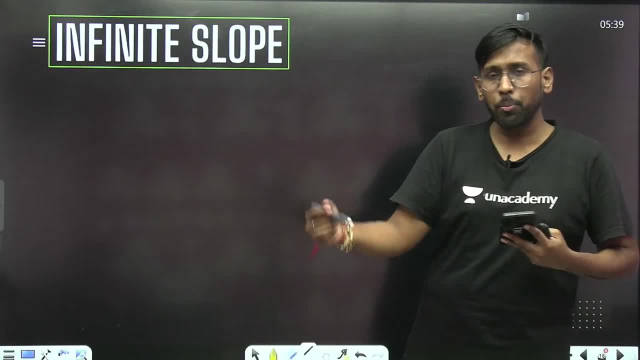 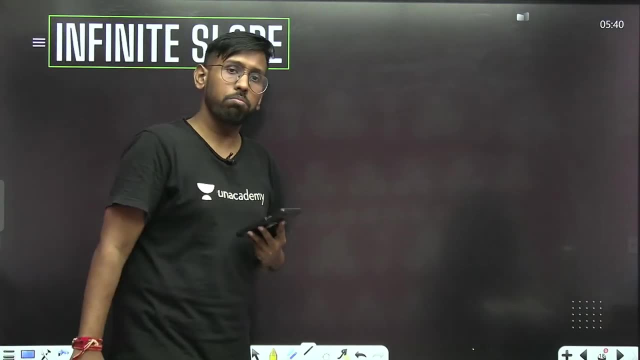 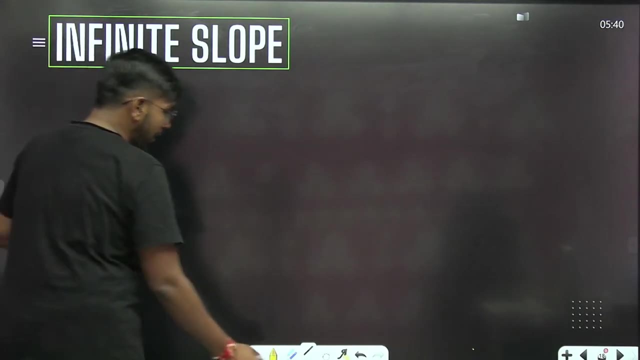 Yes, You are giving embankment. Dam's slope, Dam's slope. These are the finite slope examples. Come on. So infinite slope- Now look at my friend here. Let us say this is the ground slope. Let us say that this is the end of the ground. 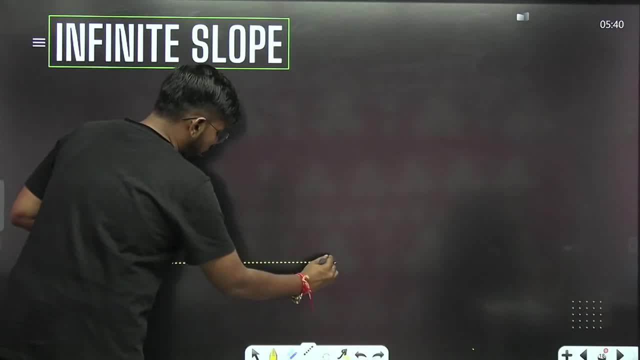 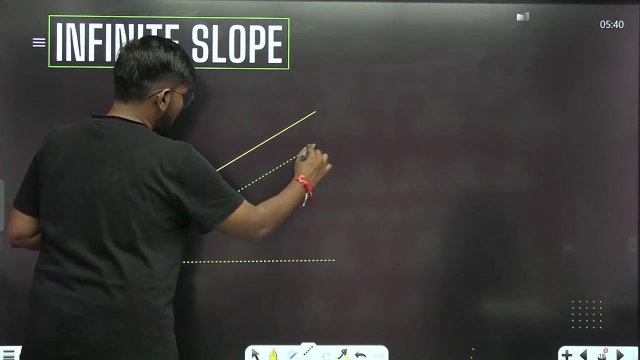 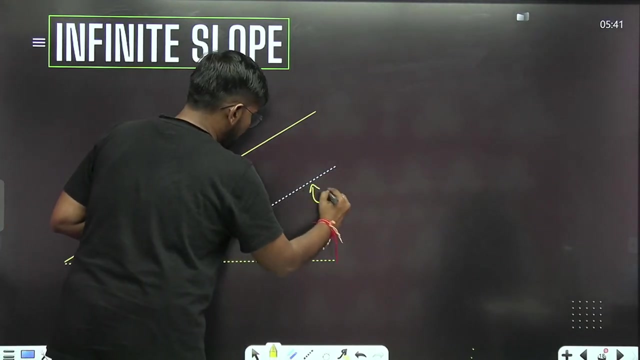 Okay, So So level: This is horizontal. Your slope is at angle of beta. Let us say this is the failure plane. Let us make it a little bigger. This is your failure plane or critical plane, about which we have to do analysis. This is your critical plane We have to do analysis for. 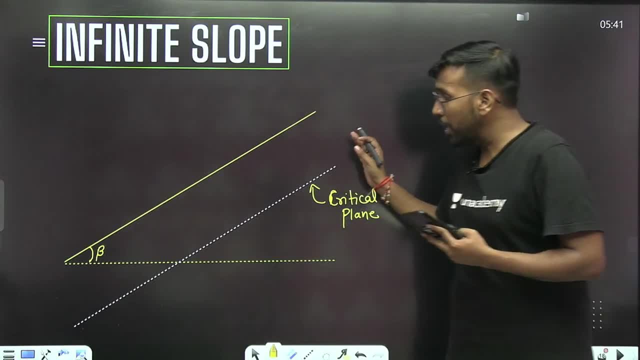 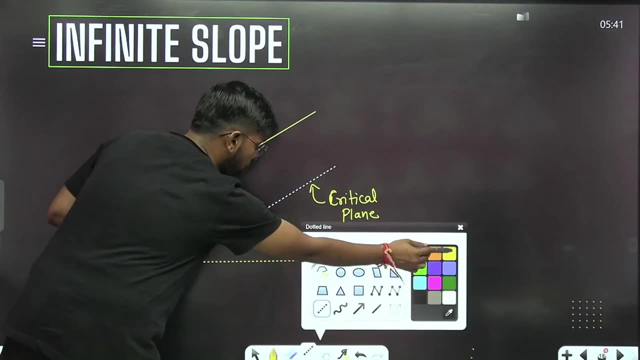 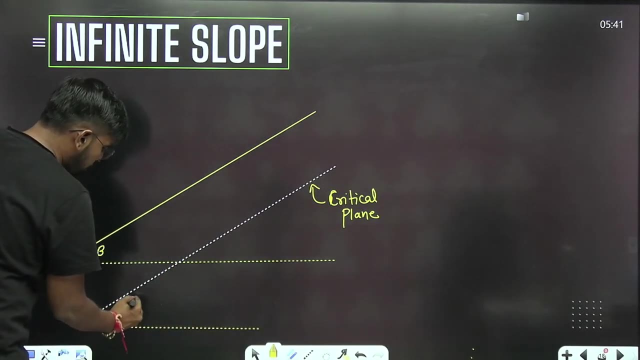 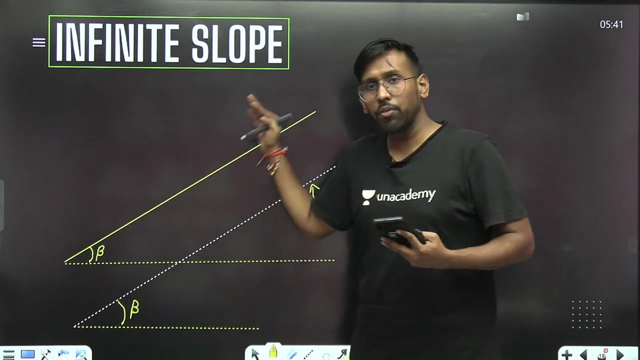 this. How much will be the angle of this critical plane with respect to horizontal? This will also be beta, Why? Because there is a sliding of the landmass at a certain depth, z The property is same. If it comes on this, then it will also be same. 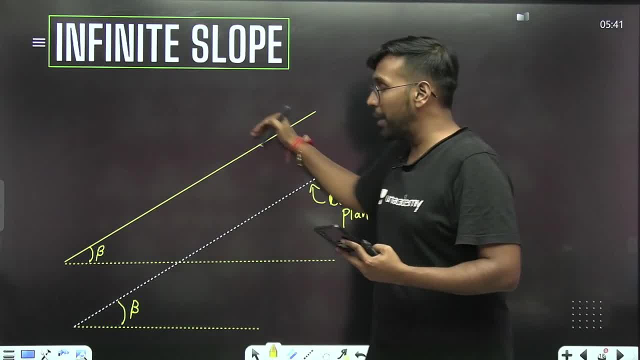 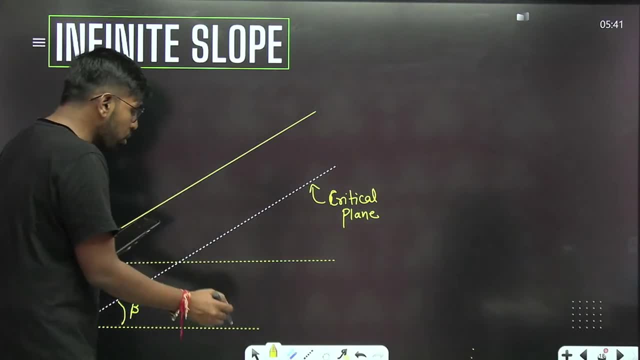 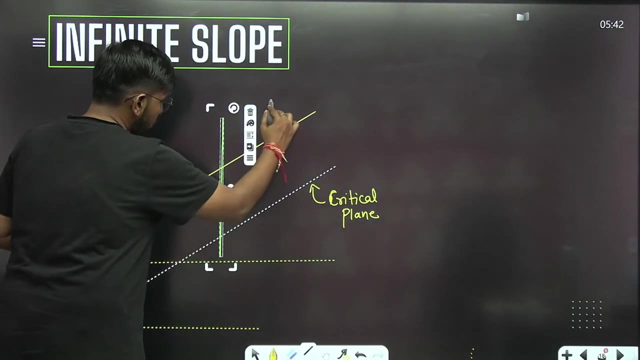 If there is unfavorable slope in the same depth, then it will be parallel to the surface. Zubleve will also be parallel to the surface. Now you will understand it in detail. To analyze this, we are going to take a certain portion of the soil, As they were saying. 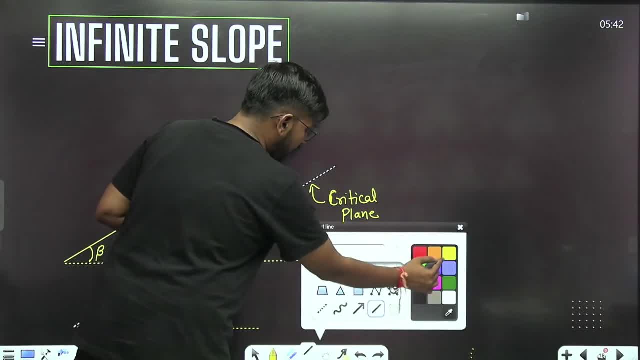 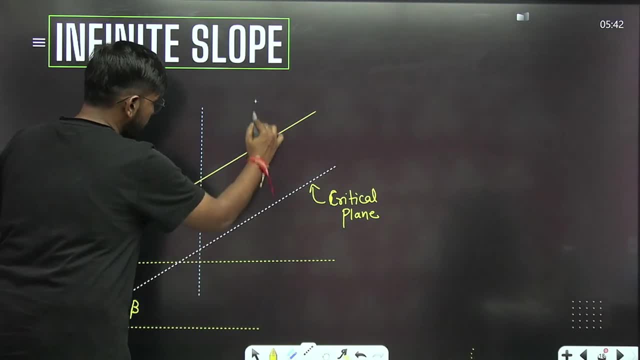 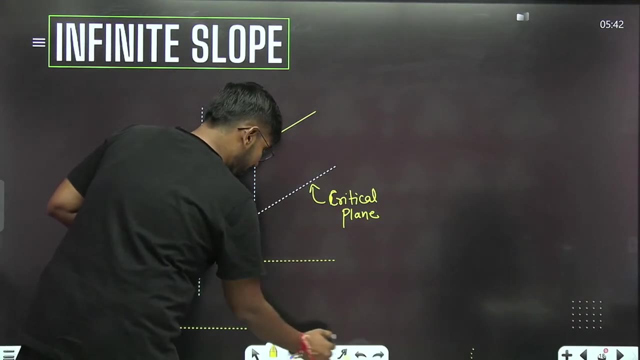 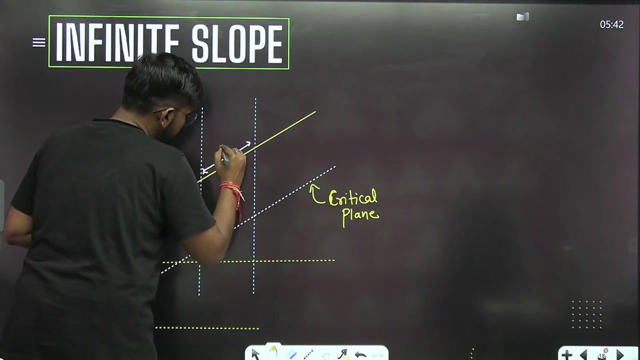 you're going to take a certain portion of the soil, That means we cannot have soil anymore. It will still be parallel. In addition, there will be a lot of air as well, of the swan. So, my friends, let us say width of the section is B. This depth is equal to. 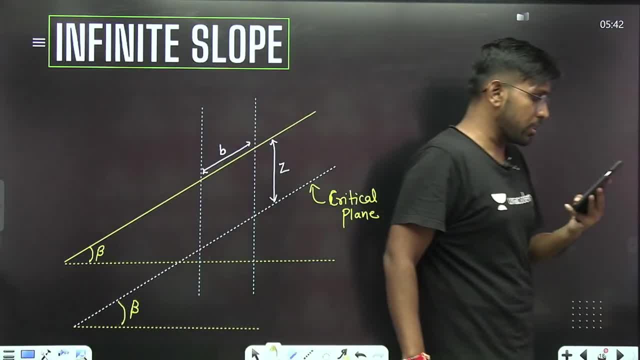 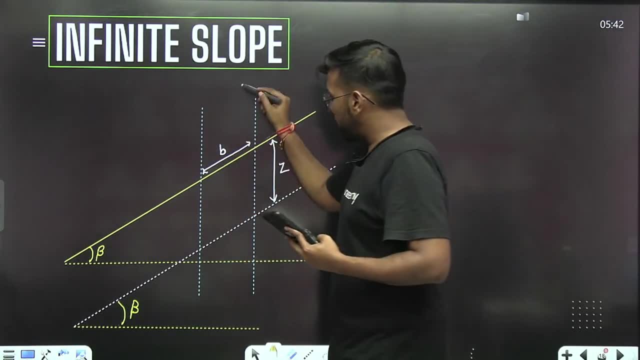 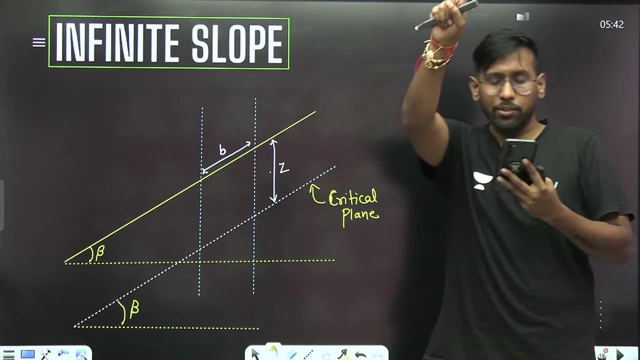 Z. This depth is equal to Z. The figure is clear. We will analyze this part. We are going to analyze this part And the thickness is assumed to be 1.. The thickness is assumed to be 1.. This point is clear. Thickness is assumed to be 1.. What thickness are we assuming? 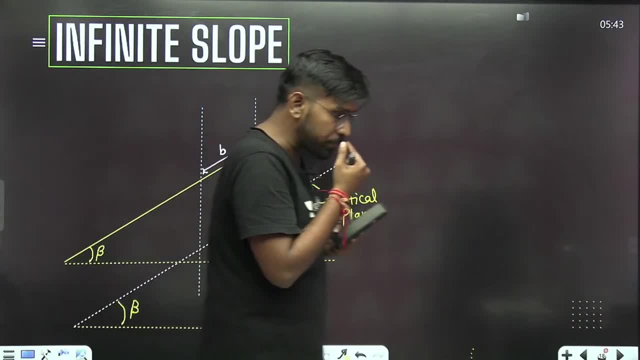 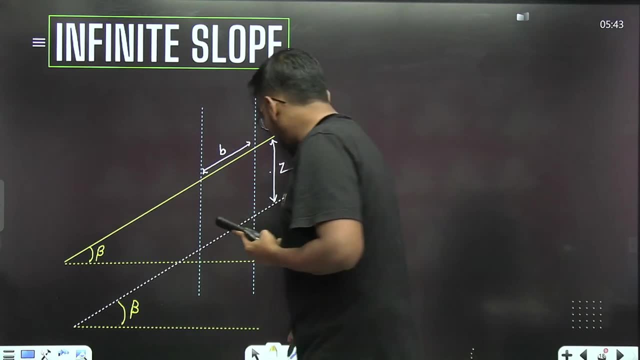 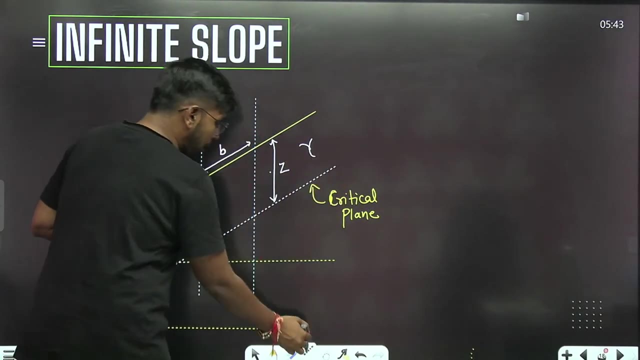 my friends, I am taking it as 1.. Okay, my friends, You will understand this thing carefully. I want, I want weight of the swan. If we are saying that weight density is Gamma, Weight density of the swan is Gamma, So what I want, I want how much weight is being applied downwards? 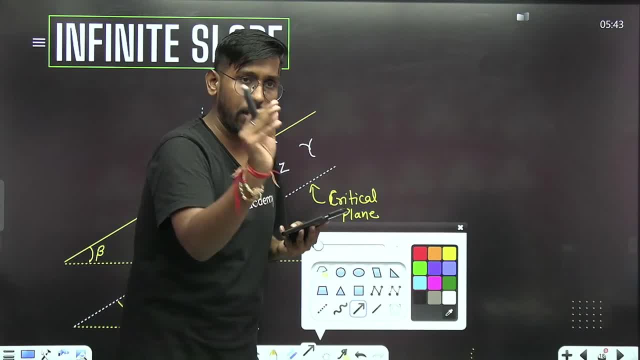 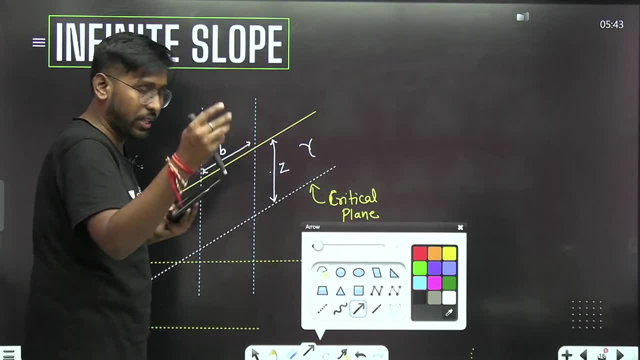 On this layer. this butt is not horizontal, it is inclined, So we will have to do it accordingly. So, on this layer, how much weight is being applied downwards? we have to see this over the width too. Is it clear? Now understand how we will take it out. 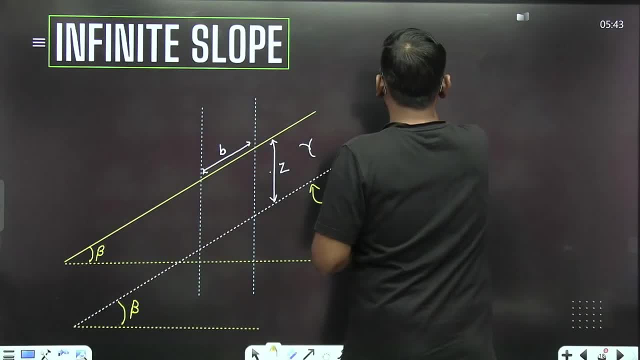 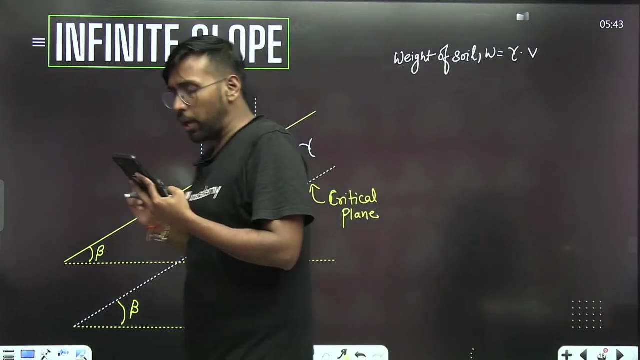 So, my friends, if we want W, weight of soil, Weight of soil, So what will the weight of soil be written? We are writing W, So that is nothing but Gamma into volume. Weight of soil is nothing but Gamma into volume. Yes or no, Weight of soil is nothing but Gamma. 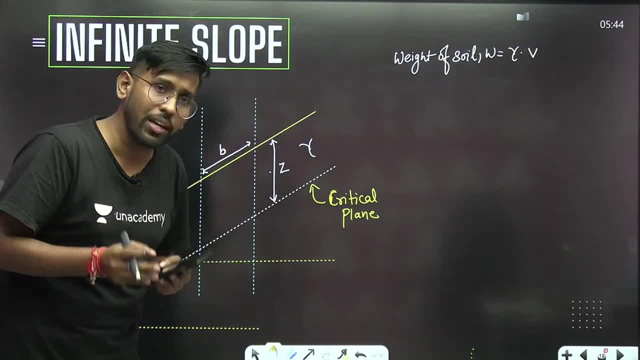 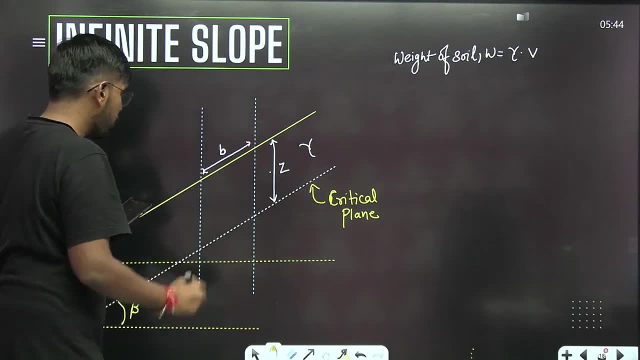 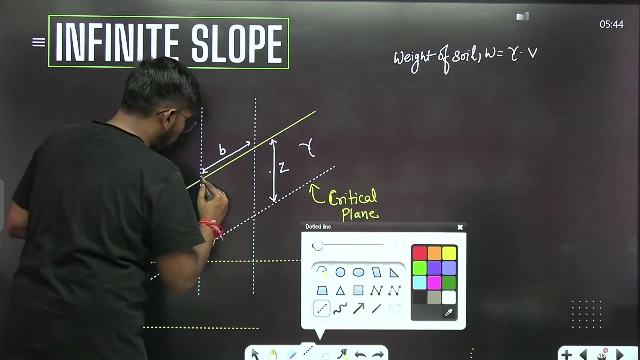 into volume, Son. we cannot write Gamma into B, into Z. Why cannot we write? Because it is not a horizontal plane, This is an inclined plane. so we will have to be patient- See here, my friends- to get the volume. we will divide it into three parts. 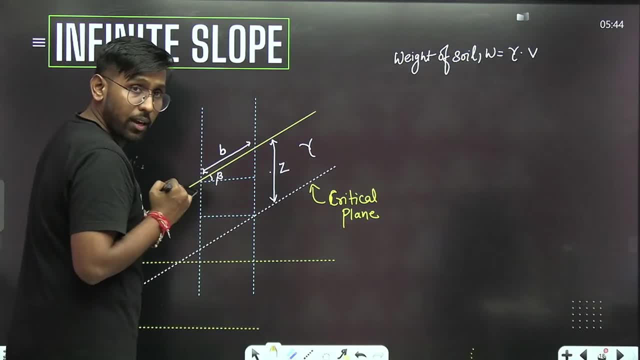 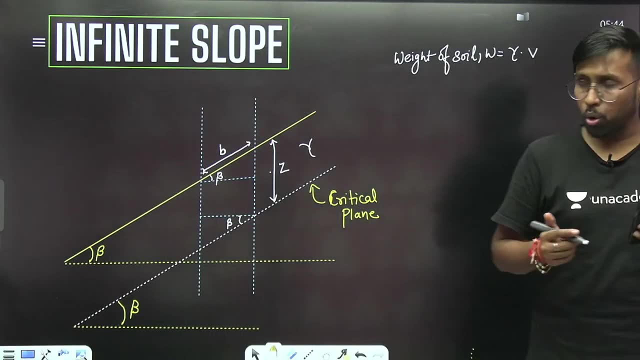 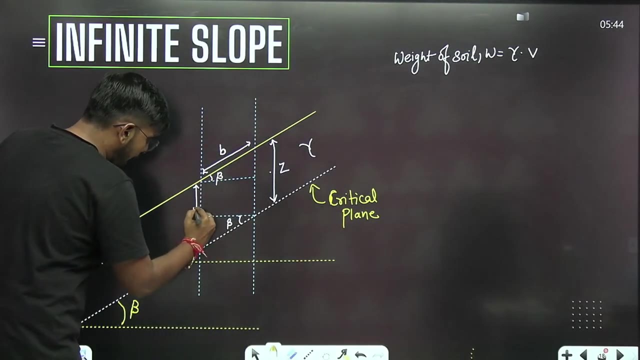 This angle will be beta. this angle will be beta. this angle will also be beta. Any doubt, Both angles are beta. Now, my friends, if we call this height y, then what will be the remaining height? z minus y? Similarly, if this is y, then what will be the remaining height? 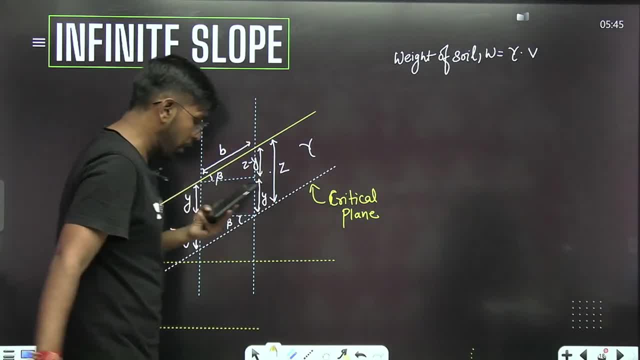 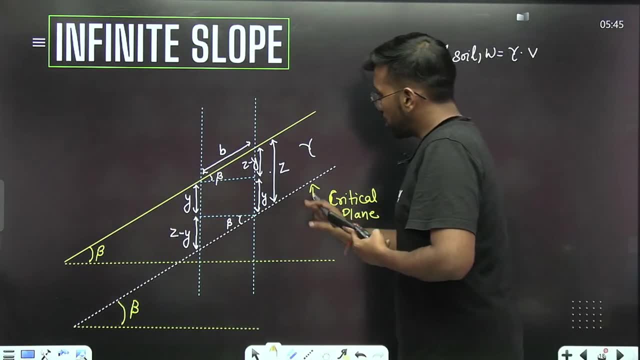 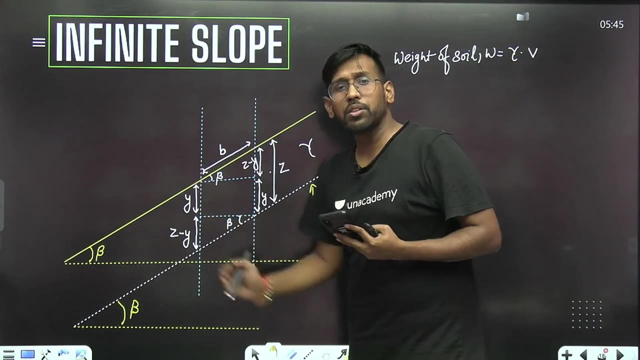 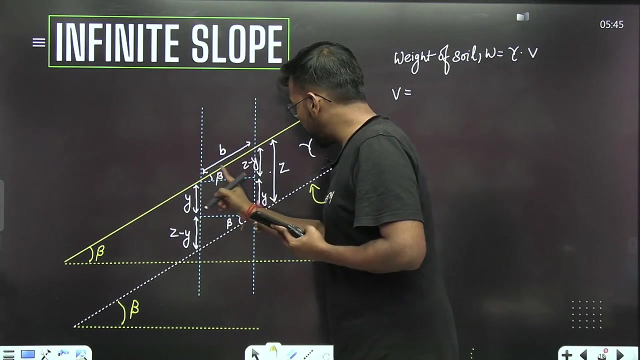 z minus y. Any doubt. Now, my friends, if you take out the volume, then what will you write? Area, whatever, your area is, multiply with 1, because you have considered thickness as 1.. So volume is equal. to check it. 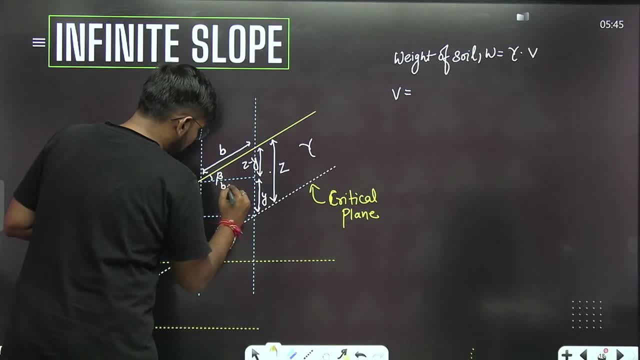 If this is b and this is beta, then what will be this b cos beta? If this is b, if the inclined length is b and the angle is beta, then what will be the length of the base? b cos beta. 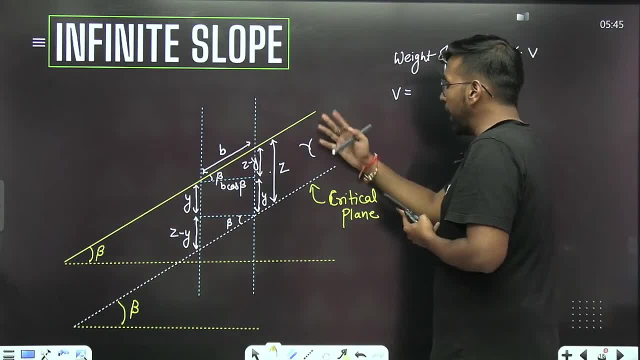 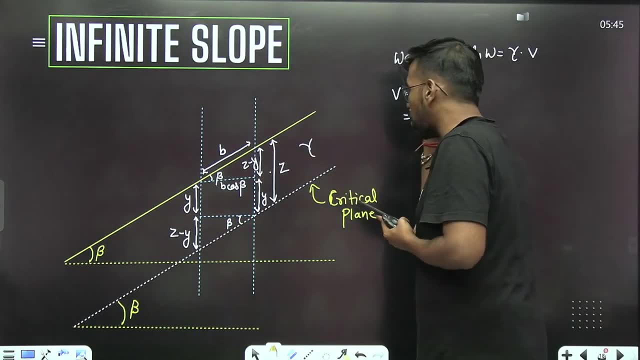 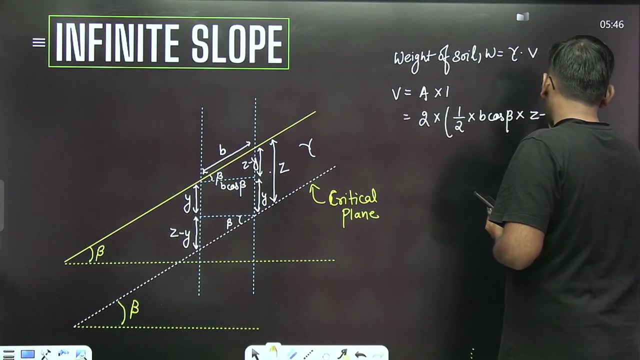 Right Now. what is the volume? Area into 1.. Total area multiplied with 1.. So what is the total area? What is the total area? 1 is used, So two parts: 2 into half of b, cos, beta into z minus y. 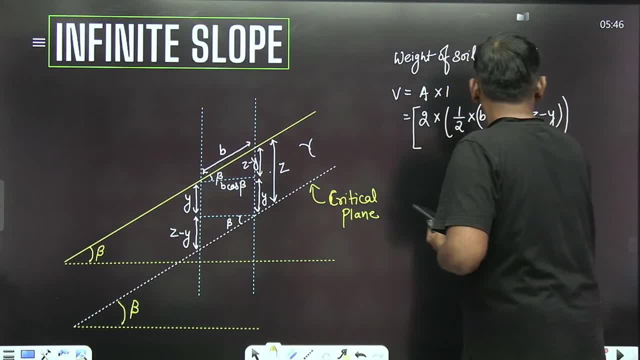 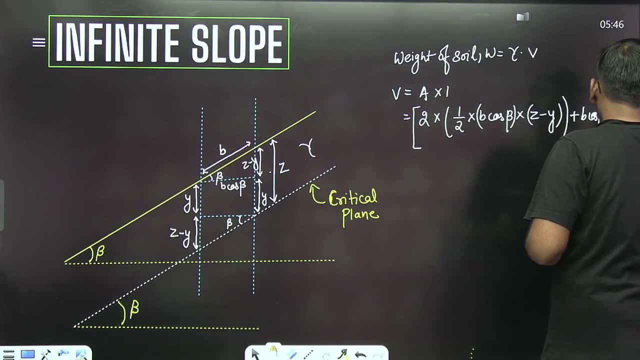 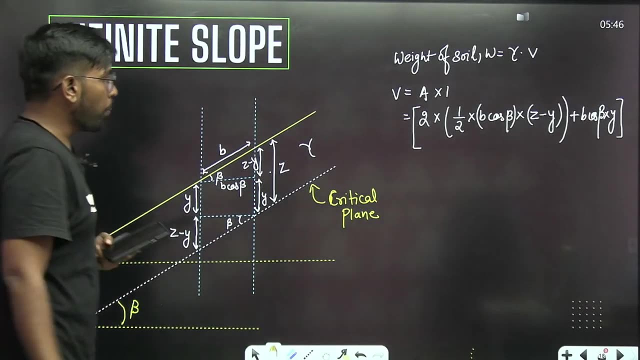 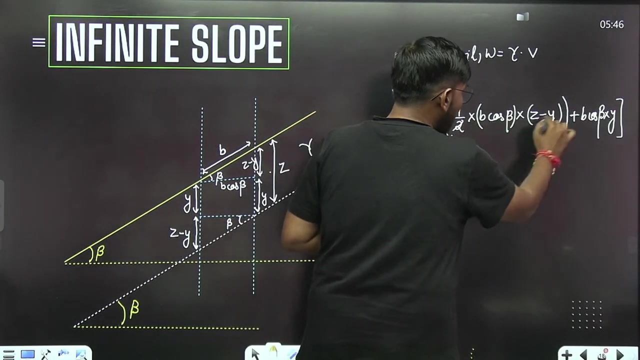 Yes or no, Plus b cos beta into y. Any doubt till here? So my friends, look here: 2, 2 is gone. 2, 2 is gone. b cos beta into y is cancelled. What did you get? 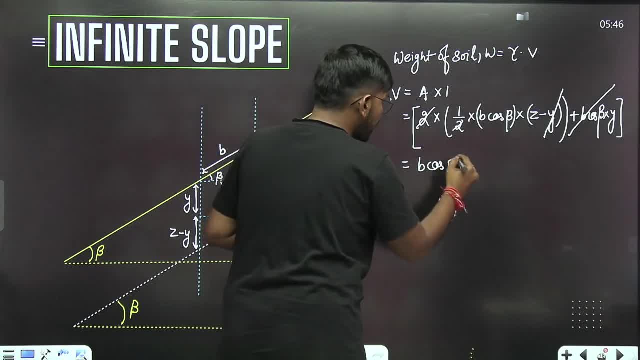 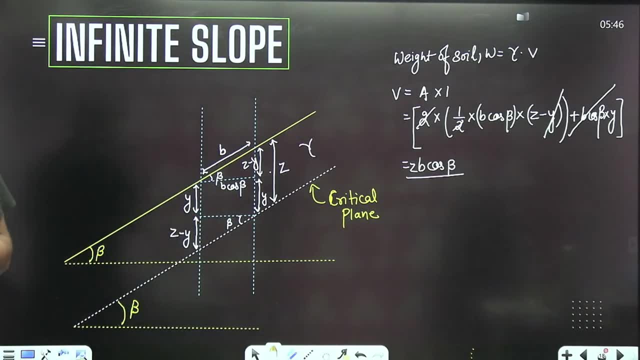 b cos beta Into z, That is, b into z, z b cos beta. This is the volume. This is the volume z b cos beta, Yes or no? The term y will be cancelled. my friend, The term y will be cancelled. 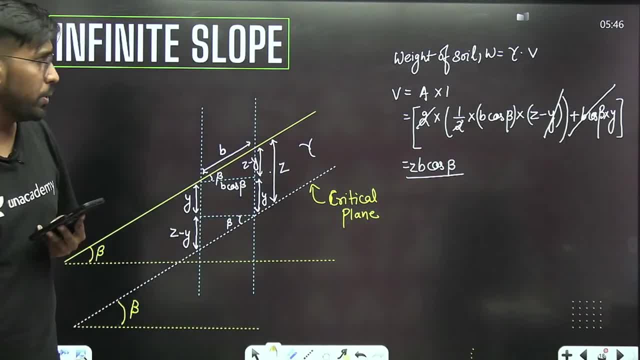 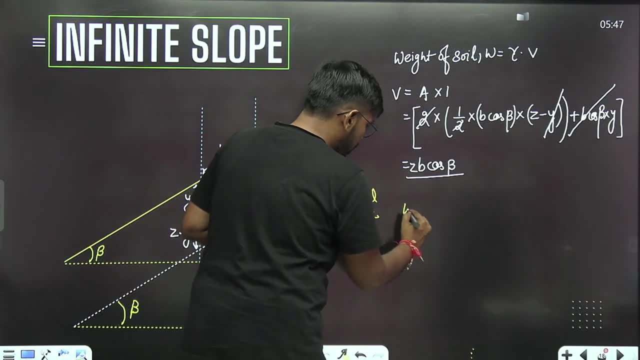 So volume is z b cos beta. The volume is z b cos beta. This is your volume. So what will be the weight of the soil? What will be the weight of the soil? Weight of the soil will be gamma, into z, into b cos beta. 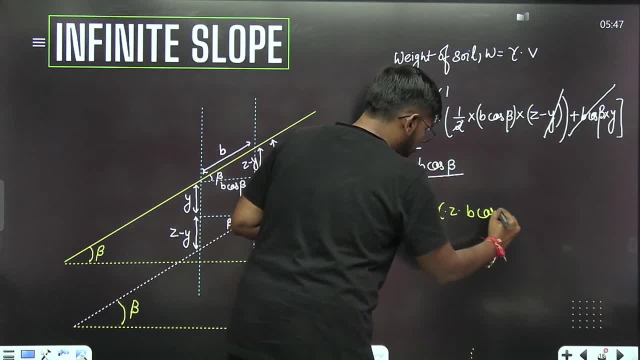 This is the weight of the soil. This is the weight of the soil, Yes or no? This is the weight of the soil over the width b on the critical plane. This is the weight of the soil over the width b on the critical plane. 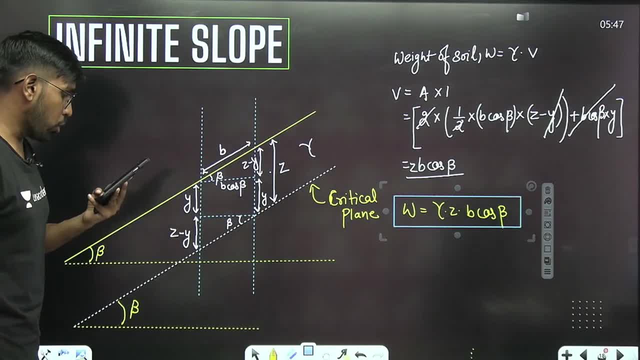 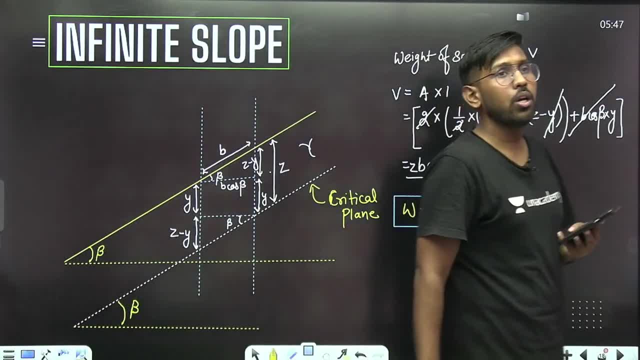 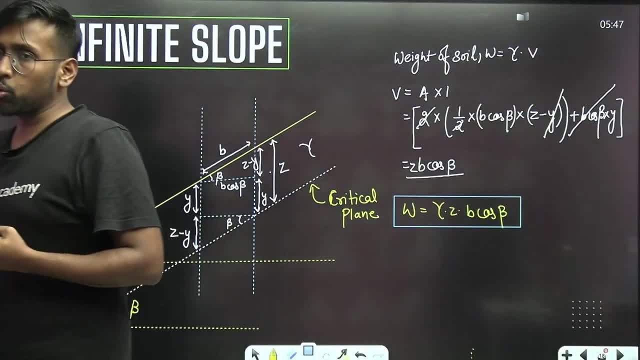 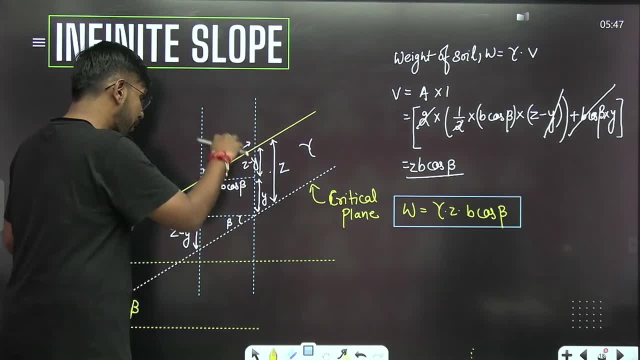 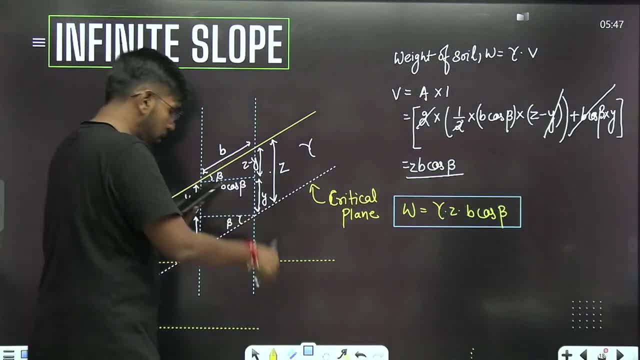 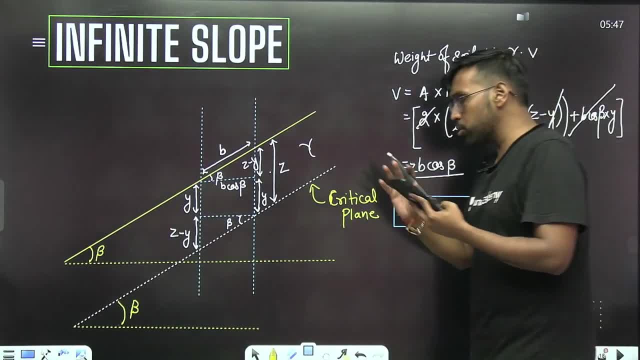 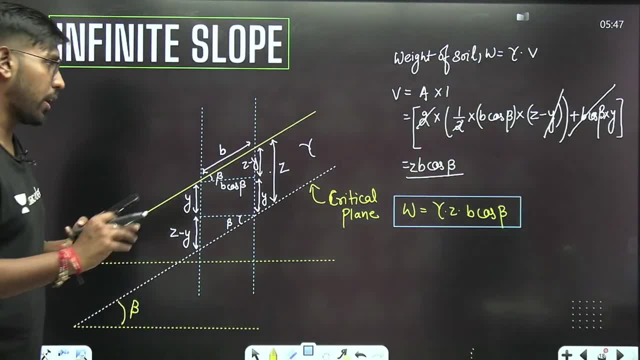 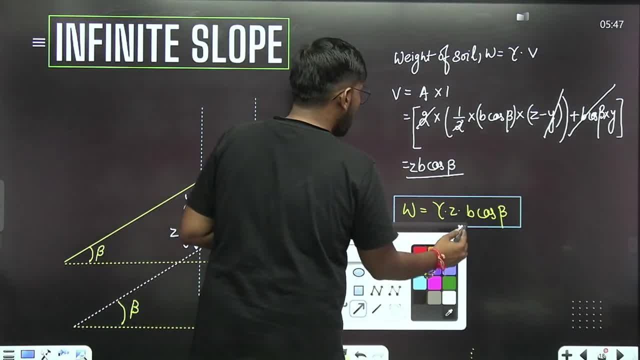 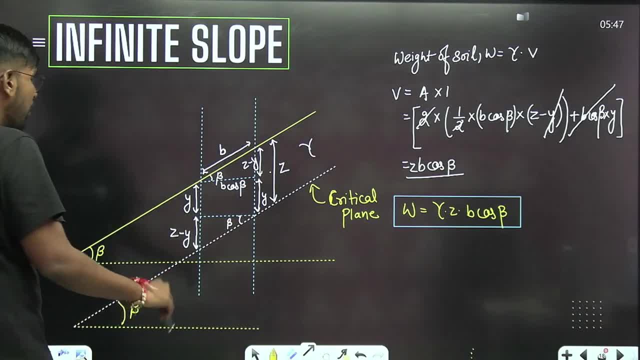 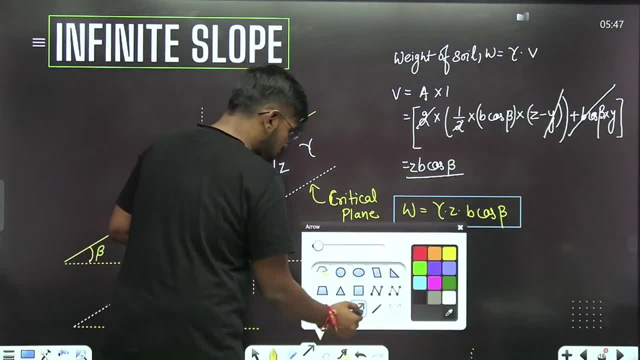 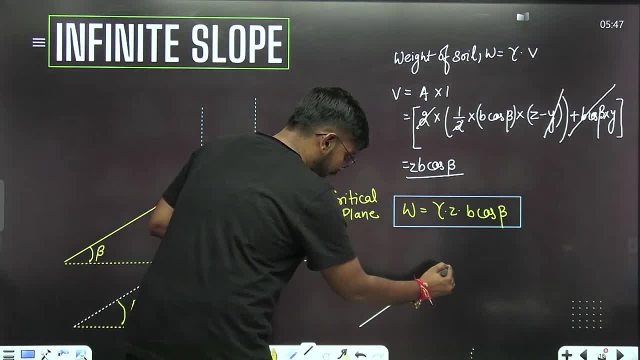 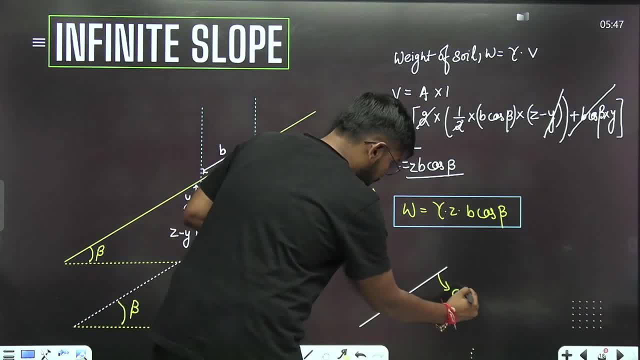 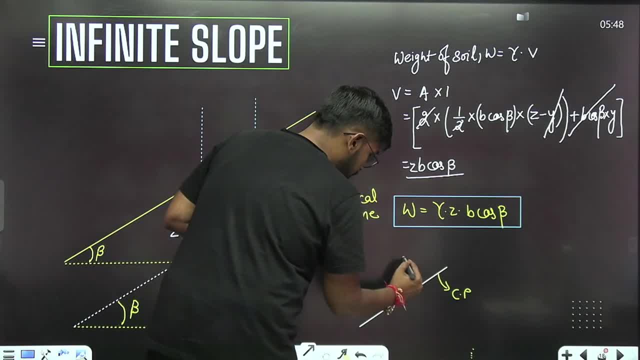 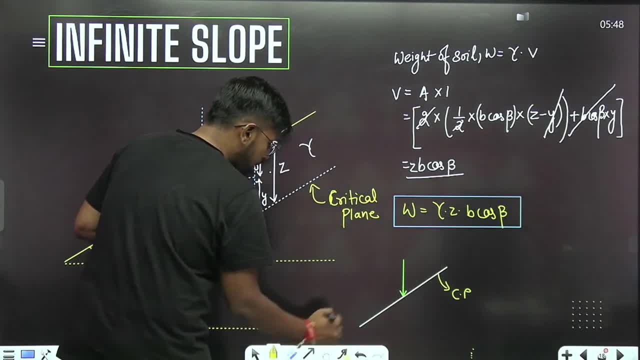 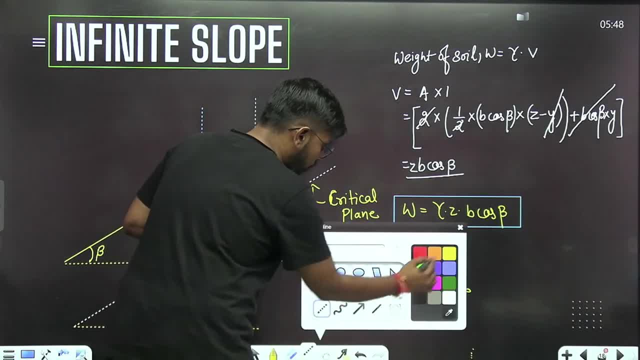 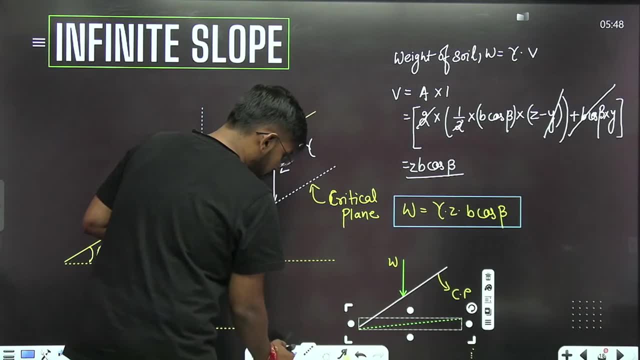 This is the weight of the soil over the width b on the critical plane which is pouring. this is the weight of the soil over the width b on the critical plane which is pouring down here. If the weight of soil over the width b on the critical plane is centered gagnantly, that 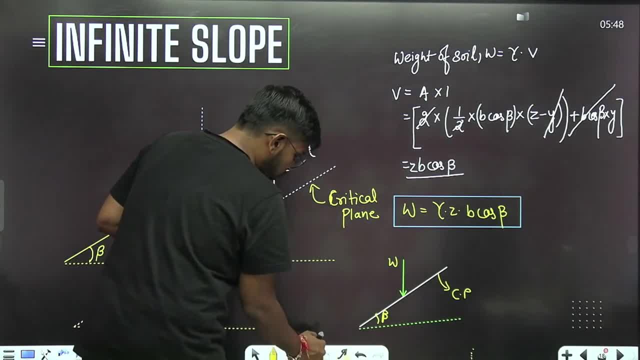 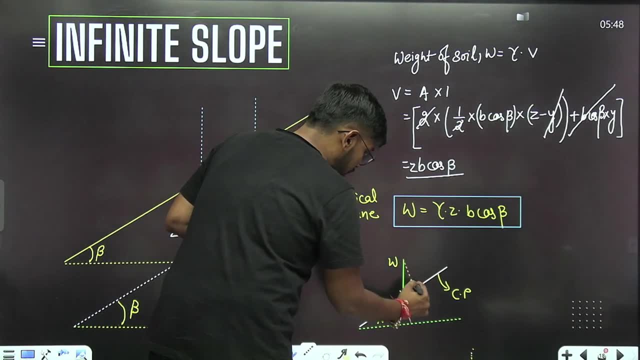 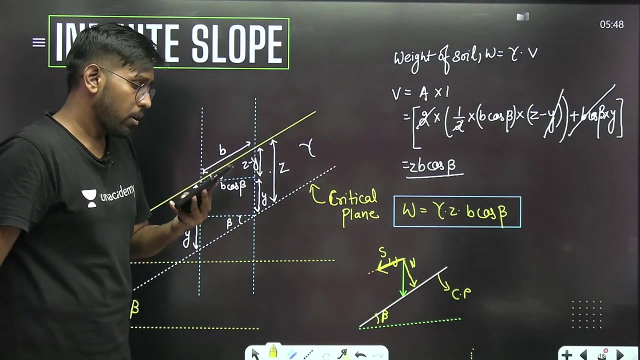 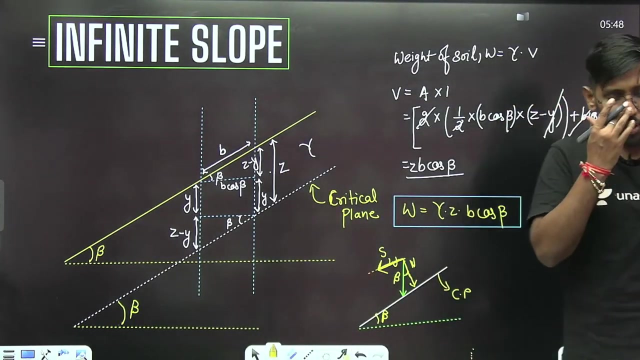 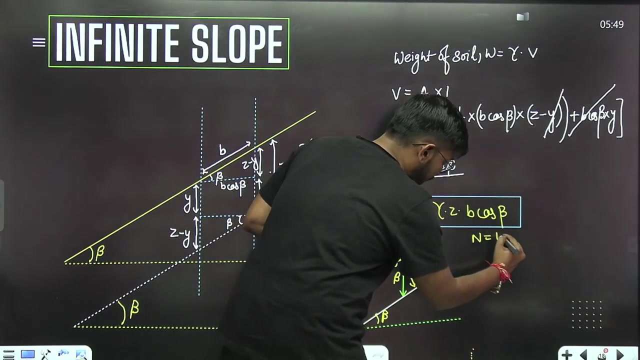 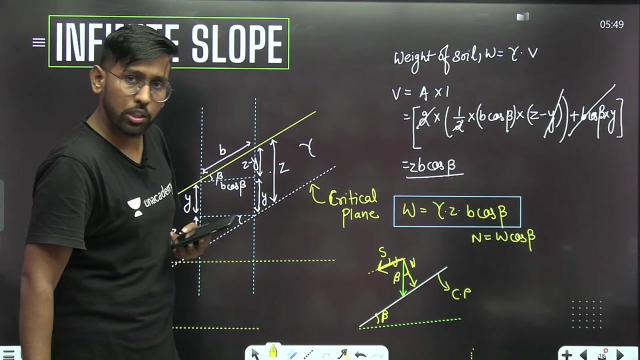 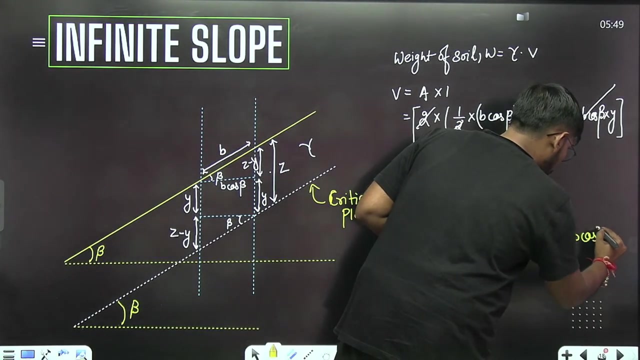 is, One component will be normal and the other component will be shear, So this angle will be beta. So what is normal force? W cos beta. Normal is nothing but W cos beta. That is what Gamma into z, into b cos square beta. 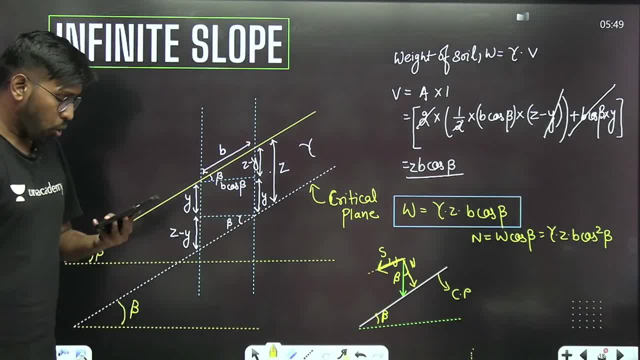 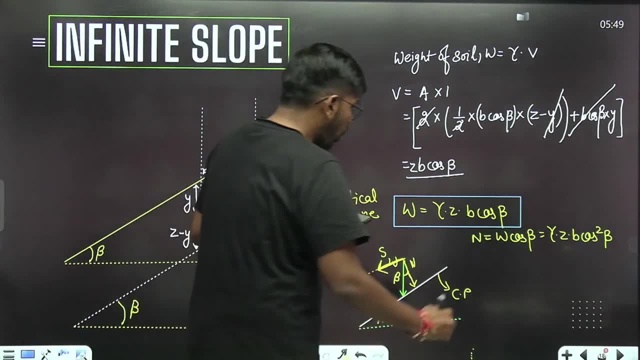 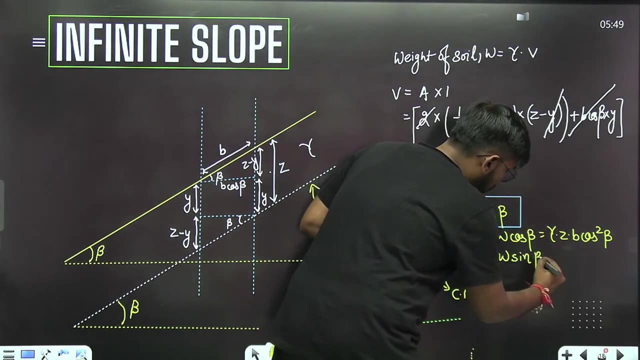 Gamma into z into b cos square beta. Tell me, yes or no. Gamma into z into b cos square beta. And if we talk about shear force, So shear force, What will be? shear force? W into sin beta. That is what. 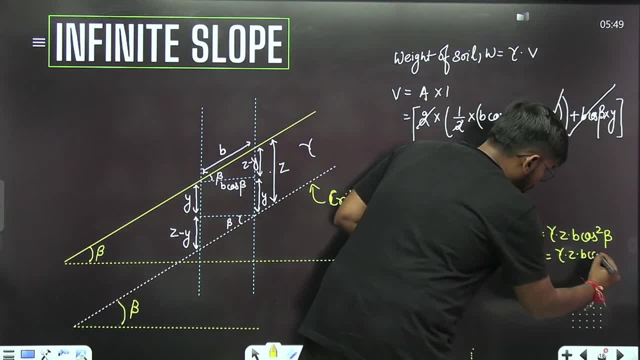 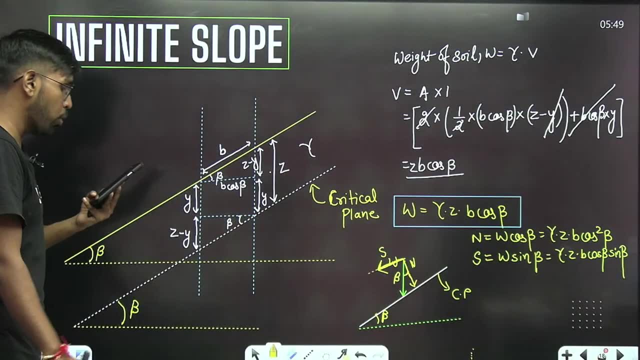 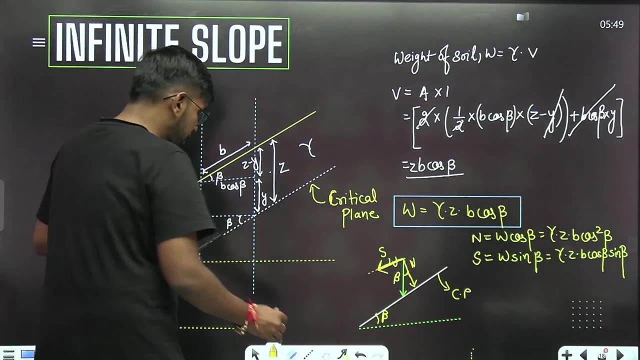 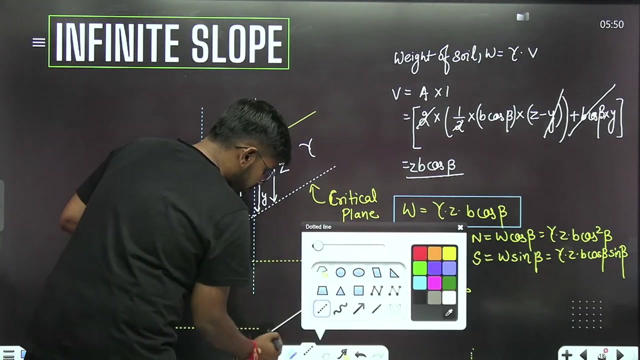 Gamma into z, into b, cos, beta, sin beta. If there is any doubt, we will say: Now, my friend, I want normal stress and shear stress. Now see here, This is my plane, This is plane of Drop. Let me learn something new, actually. 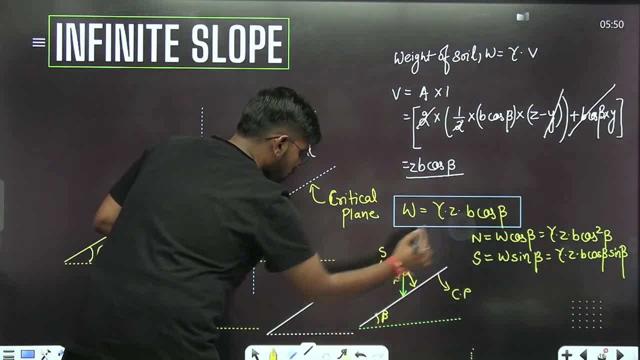 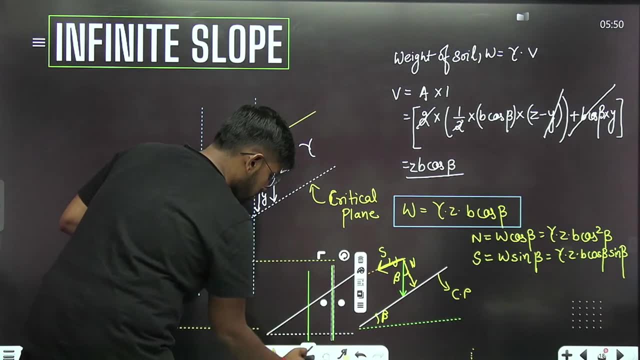 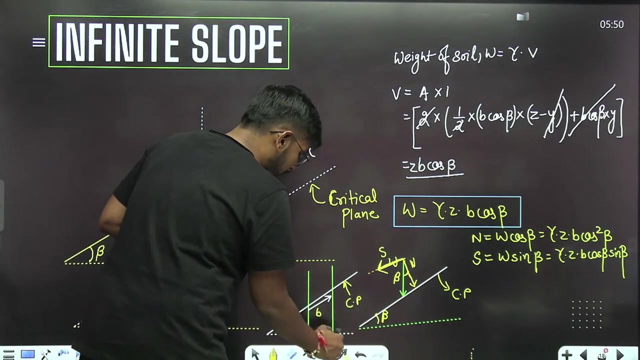 So if compared to the plane of Drop below, the edge of drop below, where is the North edge, You can see that the North edge can be seen this way: Wherever there is a paper in the point, Mars edge can be seen this way. 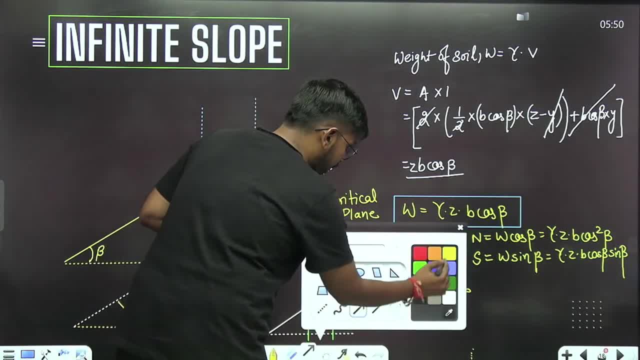 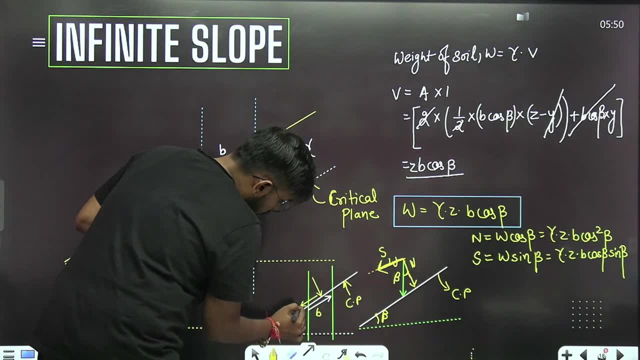 But the width here is 1 meter of 4 meter, 2 meter, So the depth is about 30 rm. okay, Now, what we are going to talk about is stress. So one stress we are seeing as normal. Second stress we are seeing as shear. 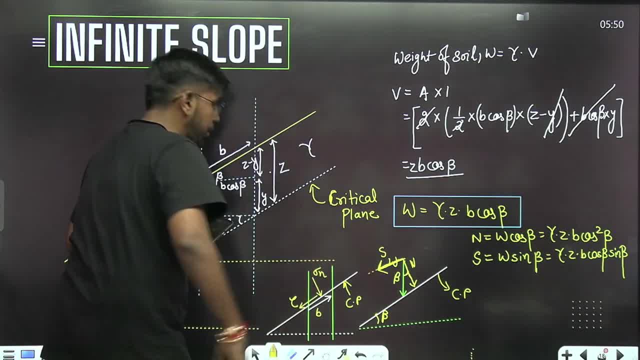 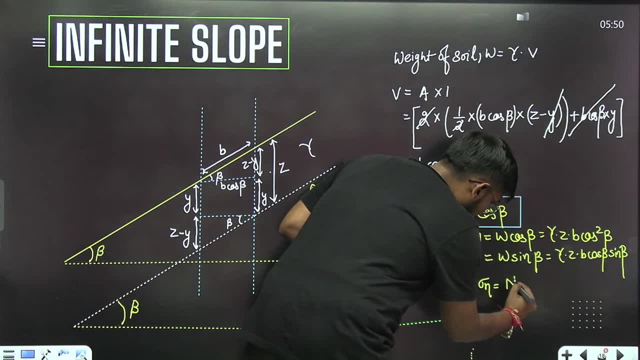 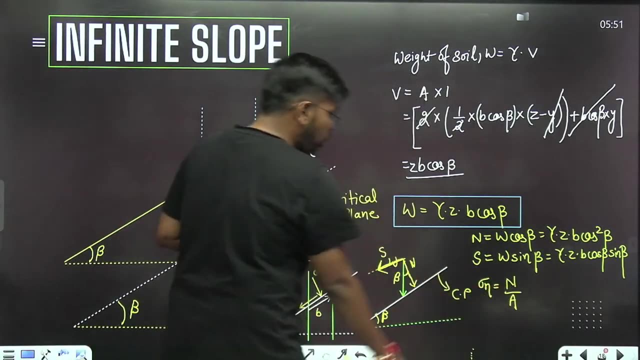 So this we are writing as normal And here we are writing as shear. So what is normal stress? What will be normal stress? Load upon area? Load upon area. Tell me, yes or no. What will be normal stress? What will be normal load upon area? 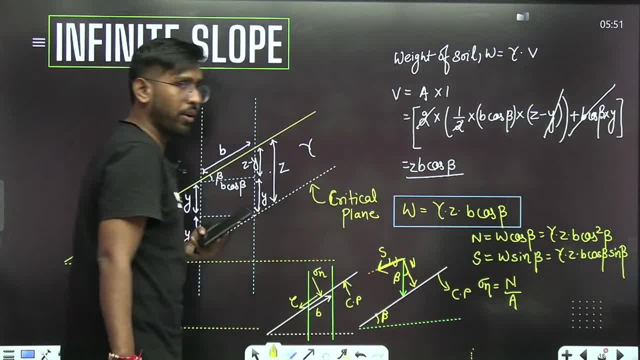 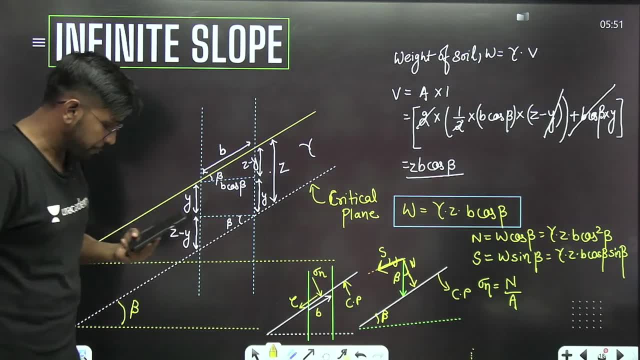 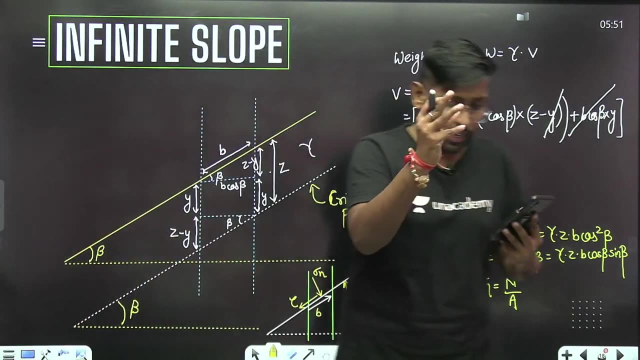 This will be normal stress. Normal stress is nothing but normal load upon area. Tell me yes or no, Yes or no. Tell me quickly. Normal load upon area. Now, what is the area? Who will tell me? How much area is it on? 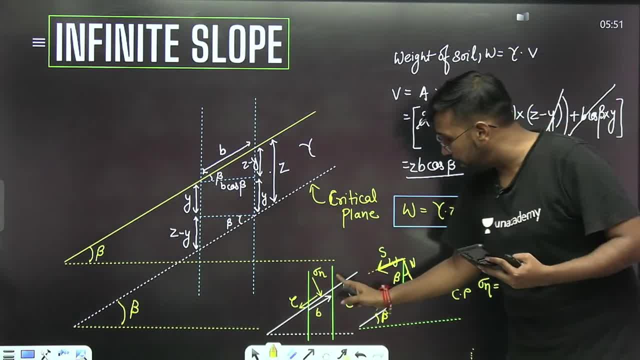 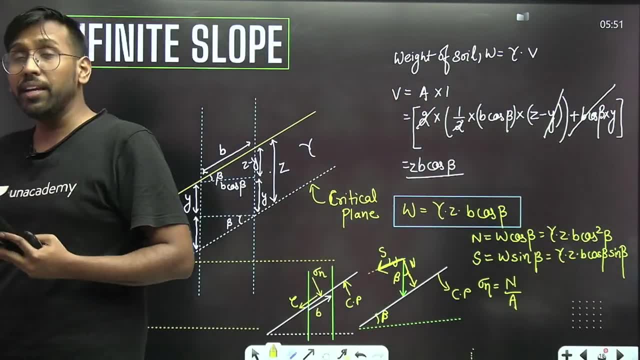 How much area is it on? This normal load is looking perpendicular and tangential. So tell me area, How much area? How much area is it on B x 1.. Very good, B x 1.. So what is normal? 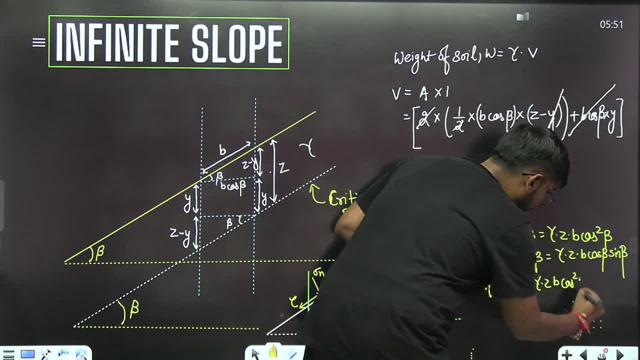 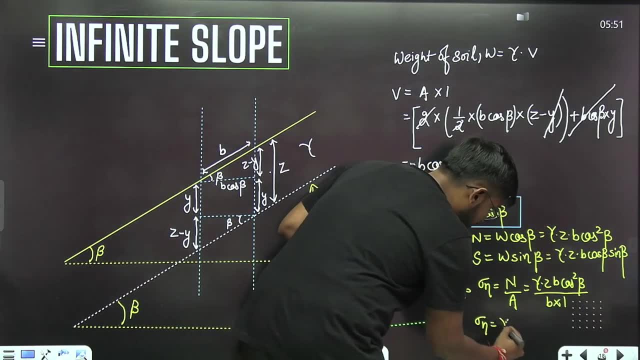 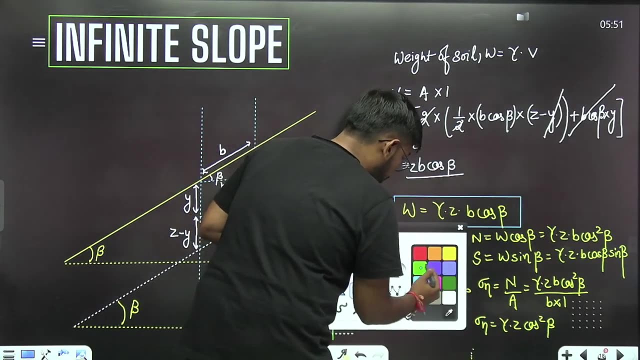 Gamma x, Z x B cos2beta divided by B x 1.. So from here, my friend, your sigma n becomes gamma z cos2beta. When you understand the concept, my friend, then happiness arises automatically in the mind. When you understand the concept, then happiness arises automatically in the mind. 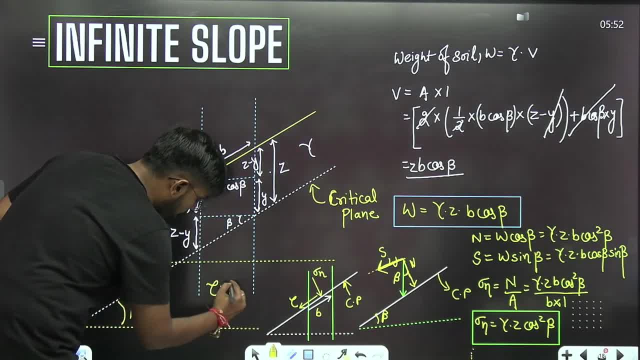 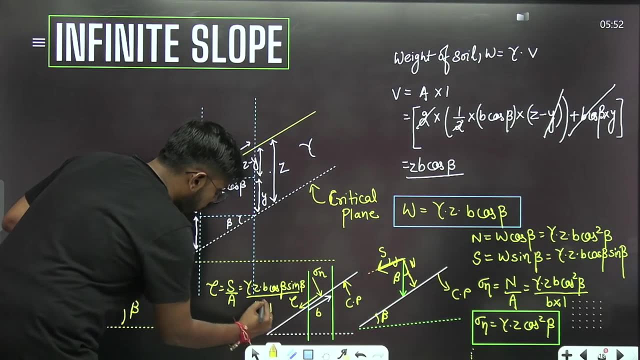 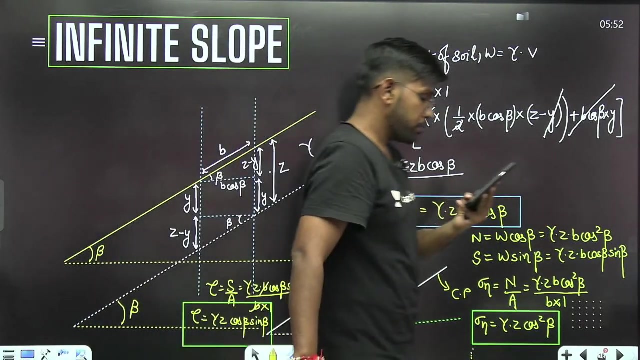 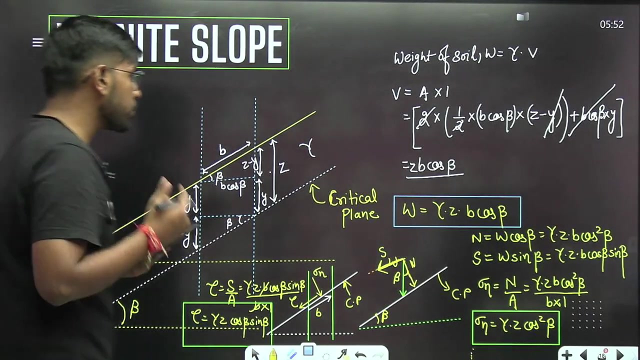 When you understand the concept, then happiness Pocket You won't get it. Is it clear? till here, Will you say, my friend, Any doubt in this? Any doubt in this? You had written direct in college. Okay, no problem, now understand. 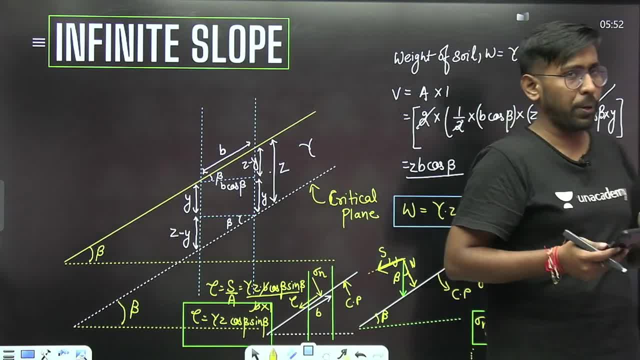 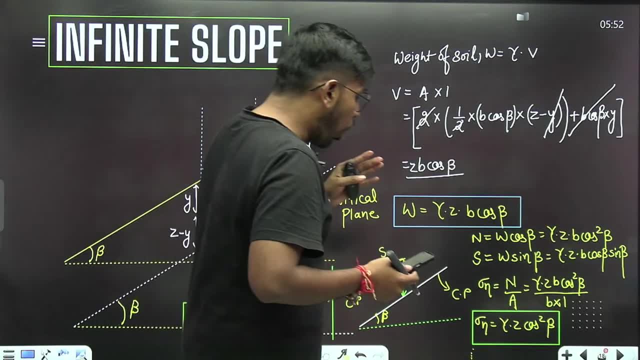 Any doubt till here. So, my friend, on an infinite slope, on an infinite slope, the normal stress that will come, that gamma, z cos square beta, and the shear stress that will come, that is gamma, into z cos beta, sin beta. Now, what is gamma? 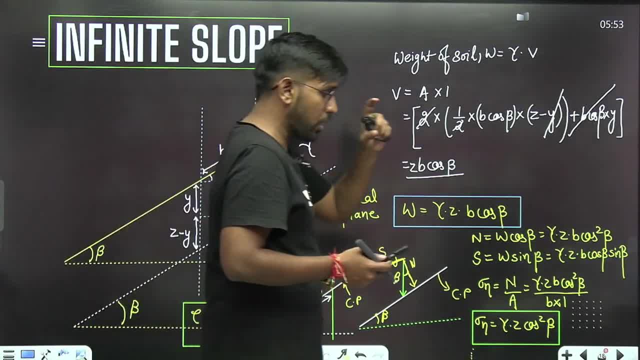 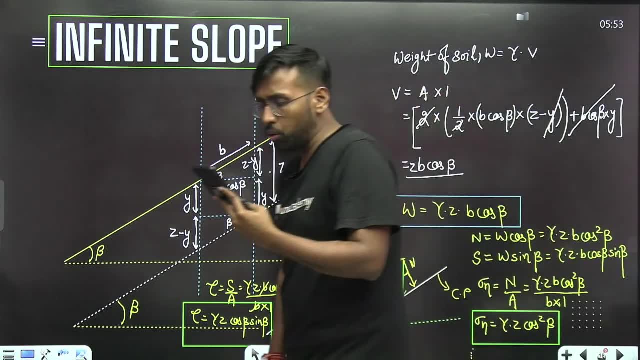 This is the unit weight. that is the unit weight of soil throughout the depth of z. This is the unit weight throughout the depth of z. There should be no doubt till here. If you liked it, then give red, yellow, green, blue. 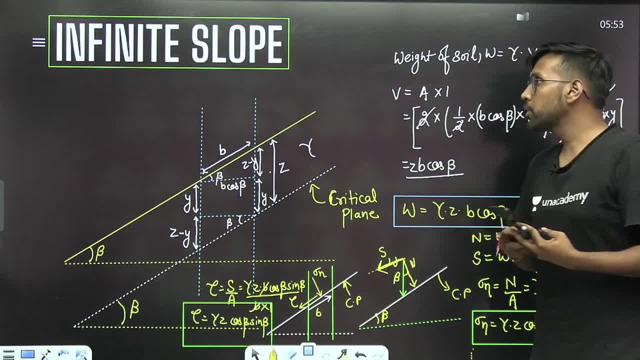 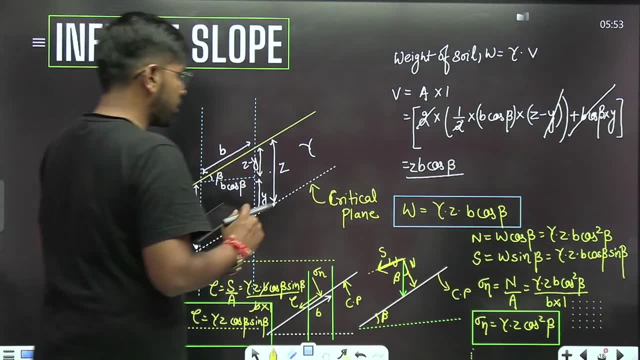 If you liked it, then give red, yellow, green, blue to the comment section. Okay, so now we have not talked about whether it is a cohesionless soil or a cohesive soil. This is written for both of us, yes or no? 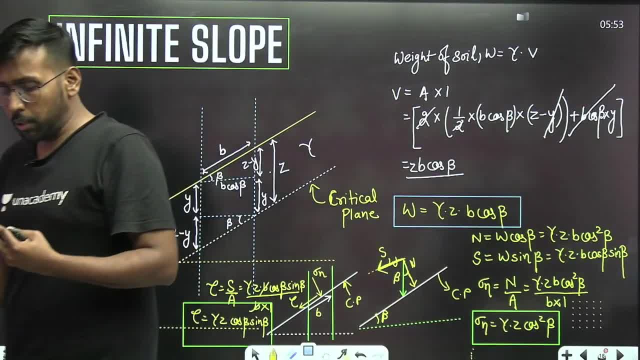 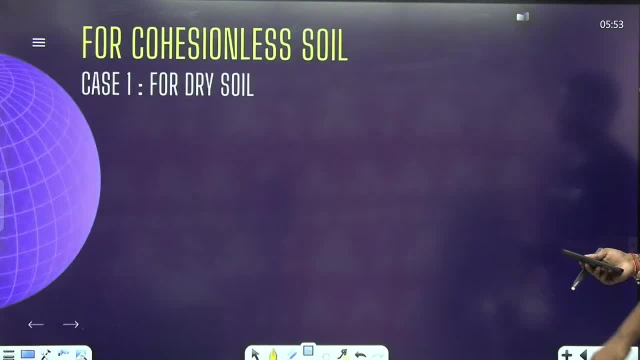 This is written for both of us. Okay, then, Okay then, Right. So now, my dear friend, we are going to talk about cohesionless soil. We are going to talk about cohesionless soil. Okay, We are going to talk about cohesionless soil. 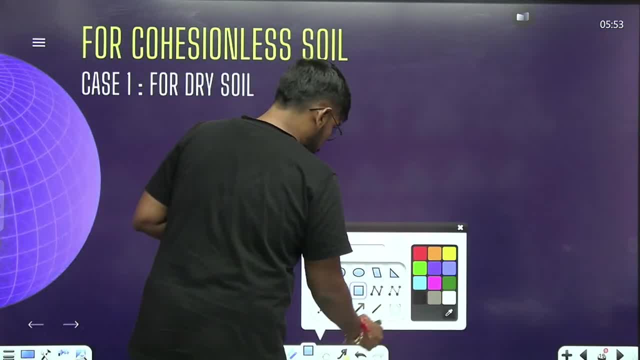 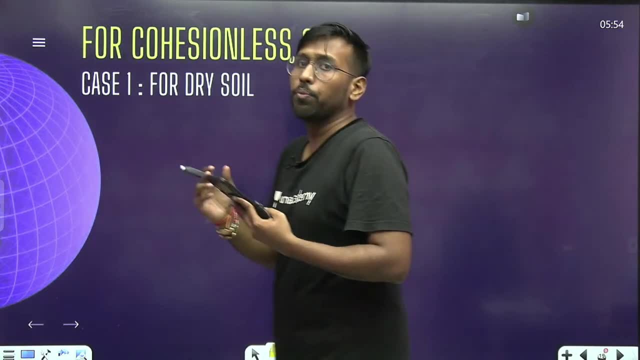 So look, understand this carefully: The soil will fail due to the soil will fail due to the soil will fail due to soil will fail due to soil will fail due to shear. So, if the soil will fail due to shear, 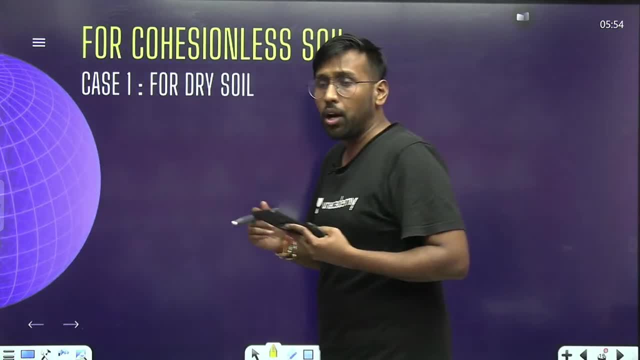 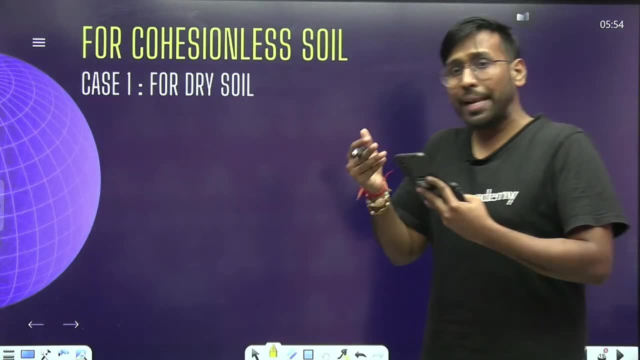 if we want to save any plane, then we have to save it due to shear. And how will it be safe in shear? How will it be safe in shear When the applied shear stress will be less than the maximum shear stress, That is, the shear strength of the soil? 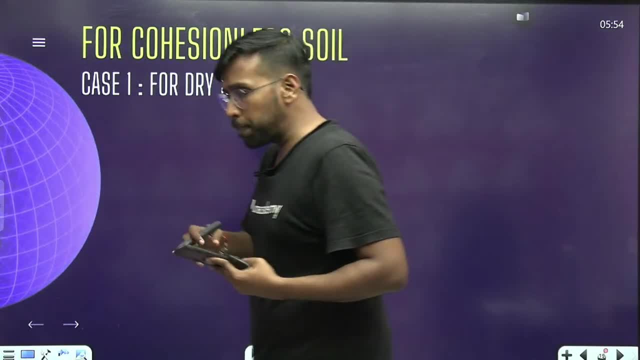 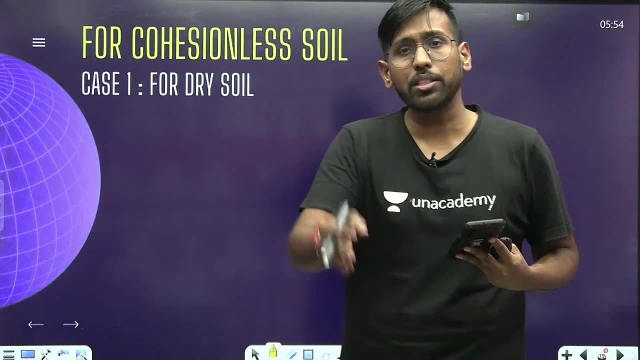 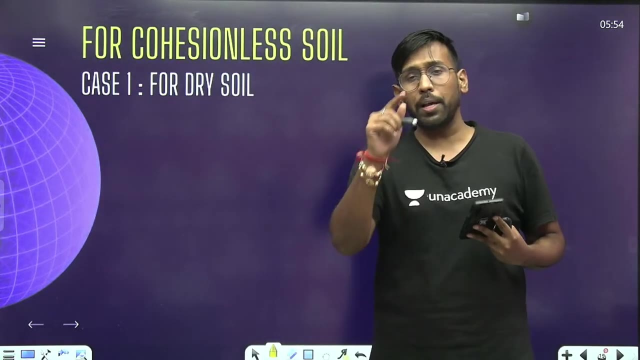 Only then it will be safe. right Now the plane you are talking about. The shear on the field is maximum shear, or the shear allowed on the field, or when the shear strength of the soil is less, then only that plane will be safe. So, my friends, if we want to make it safe, if we want to save the critical plane, then we will talk about the factor of safety. 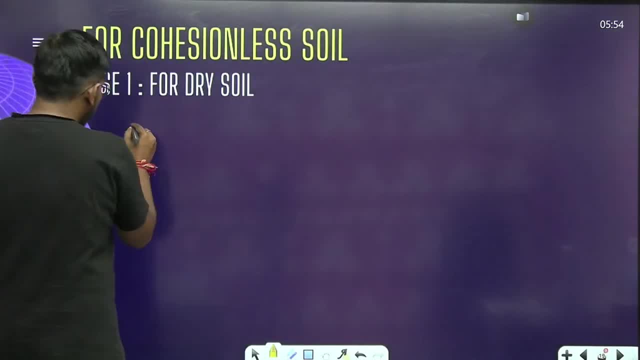 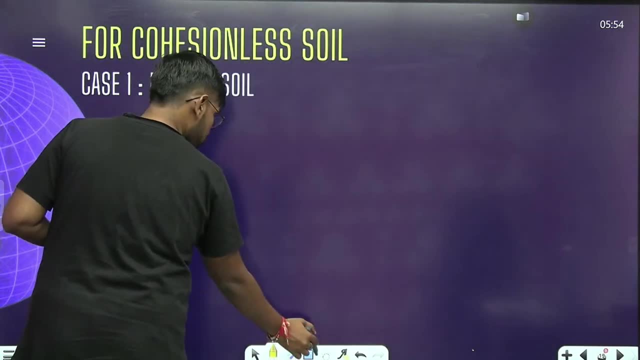 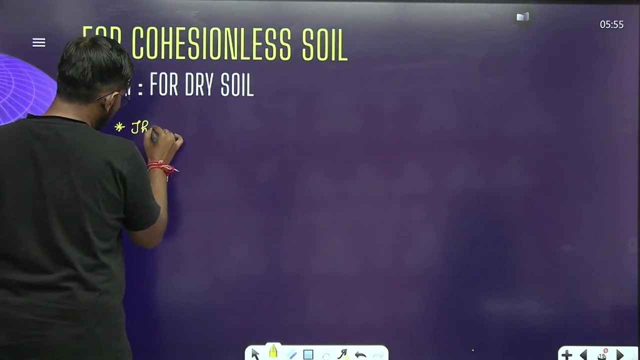 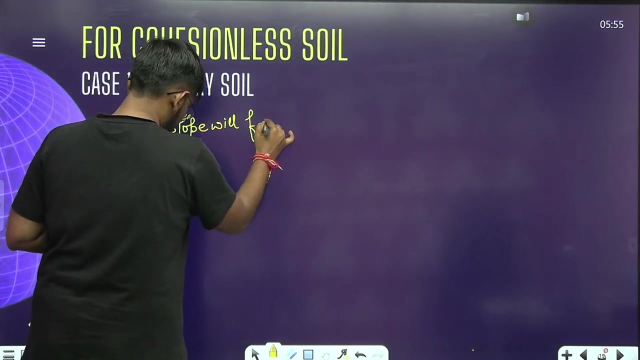 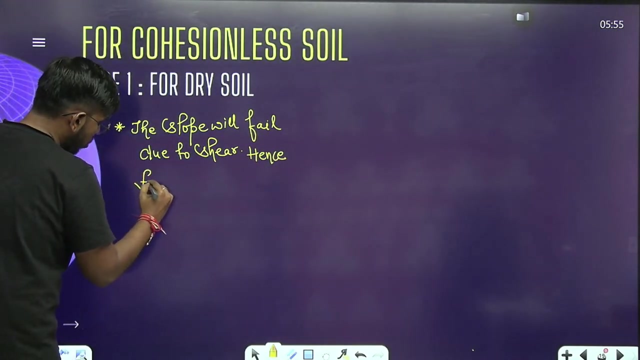 We are going to talk about the factor of safety. So, my friends, here we will write some points first, and then we will come to dry soil. The slope will fail due to shear. Hence, Hence, Hence For the, For the, For the safety. 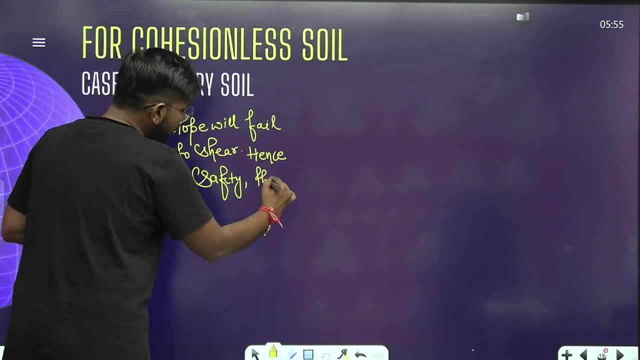 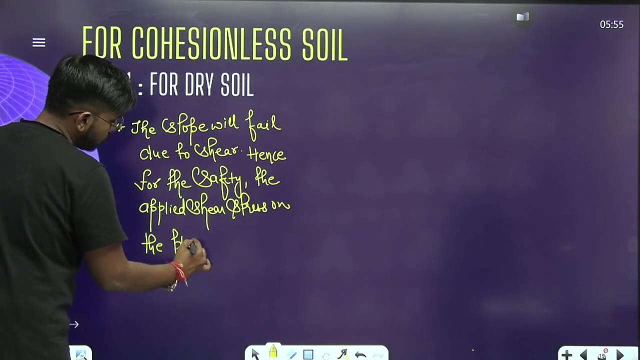 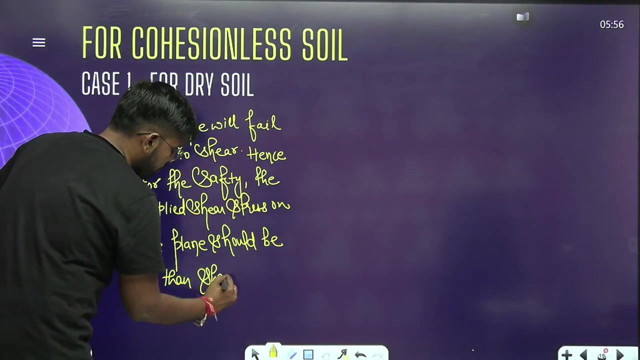 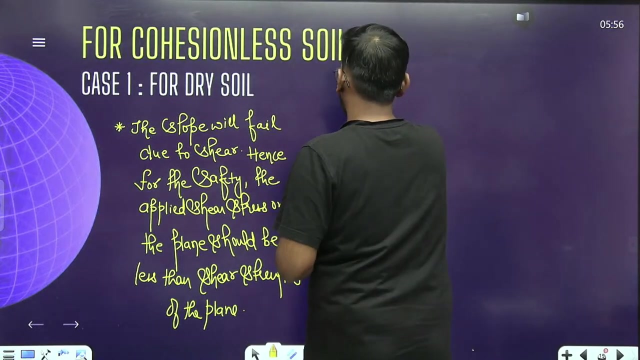 For the safety, The applied shear, The applied shear stress On the plane Should be: Should be less than less than shear strength: shear strength of the plane, of the plane. ok, is this point clear to everyone? is this point clear to everyone? now, my friends, if we talk about 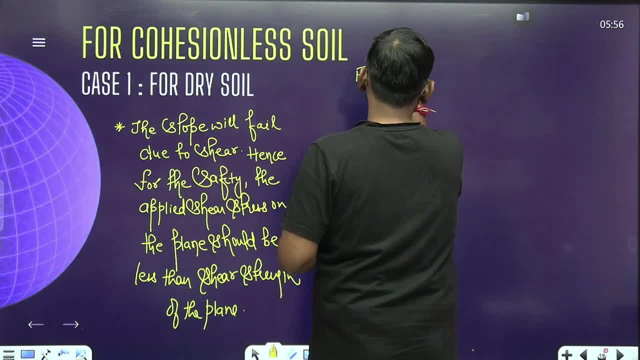 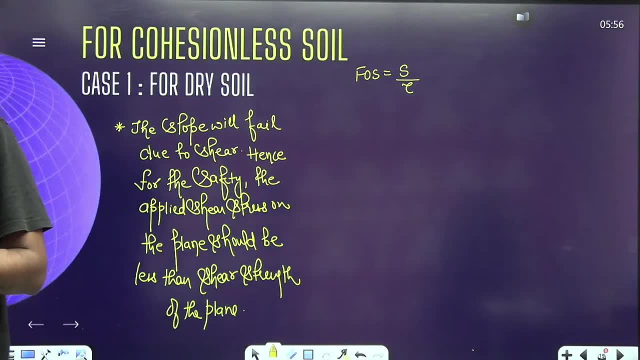 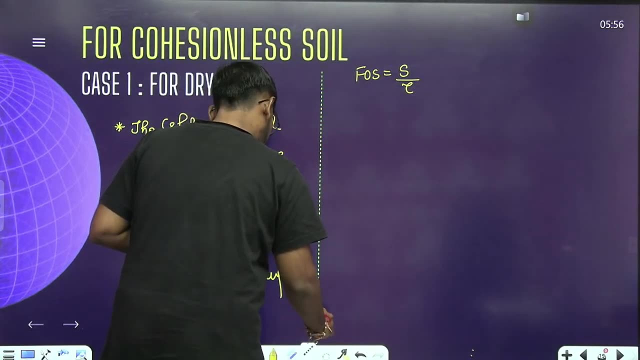 factor of safety, then what will we write? factor of safety, shear stress, shear strength of the soil by the applied shear stress. so if we are defining factor of safety, then what will we write? shear strength of the soil upon shear stress. no doubt till here. no doubt till here, my friends. 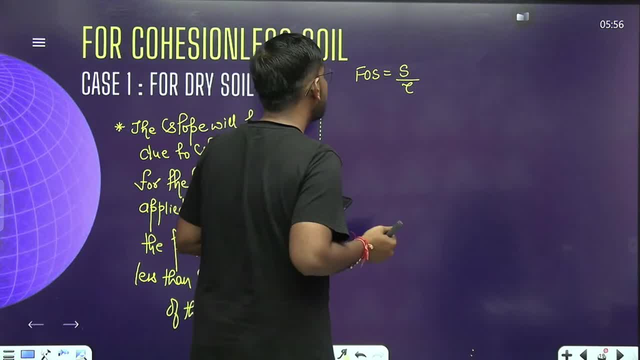 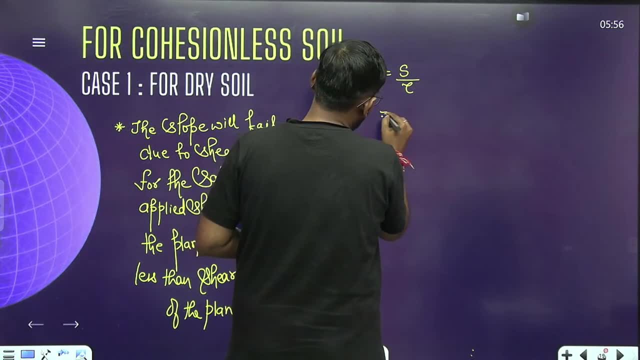 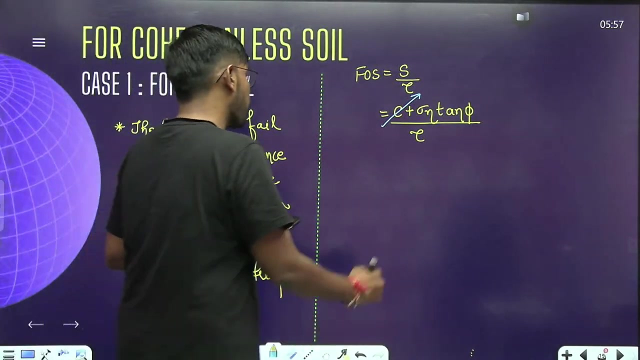 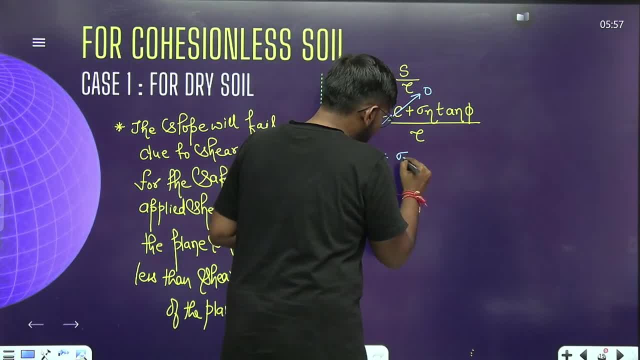 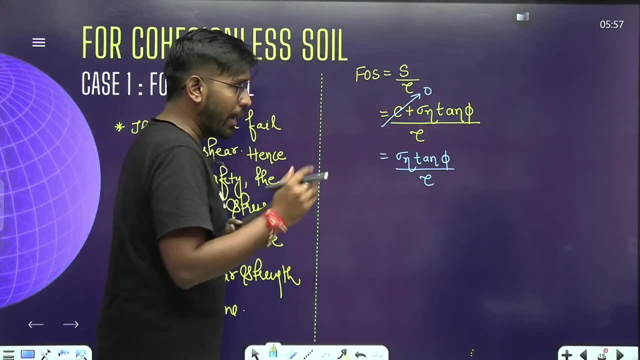 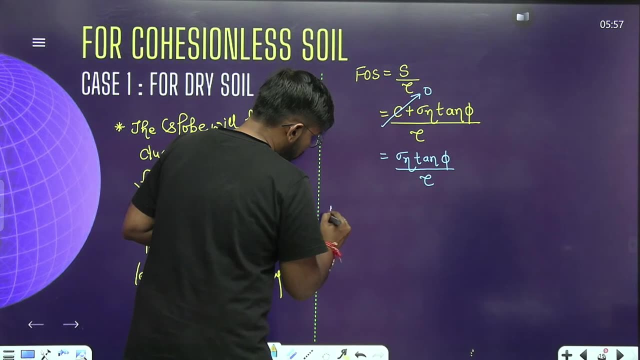 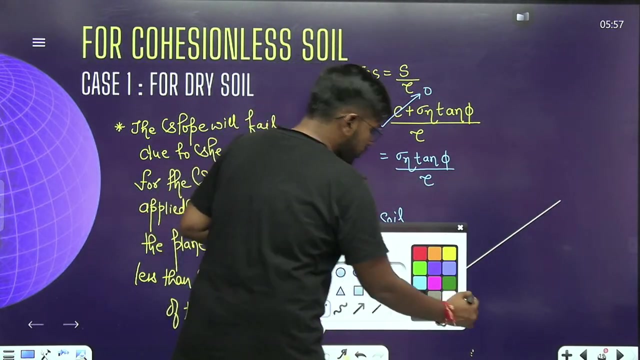 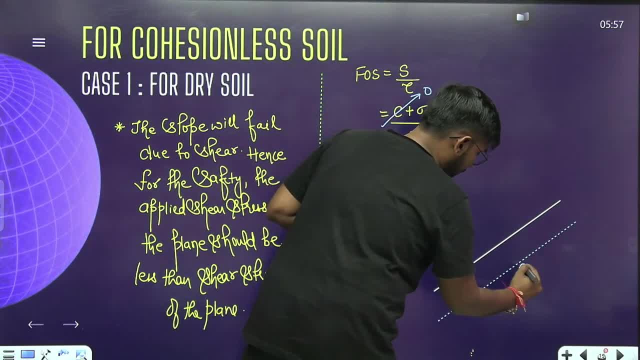 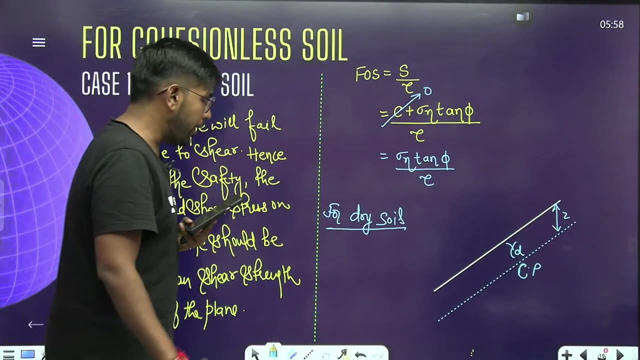 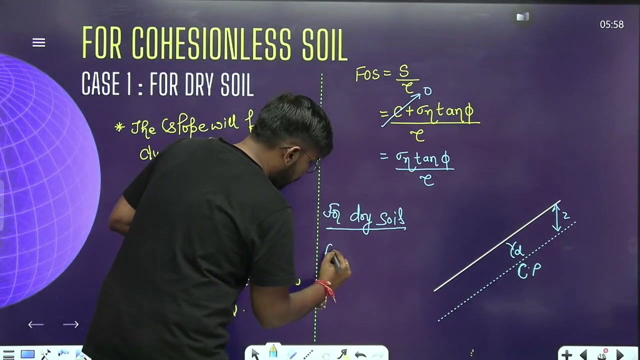 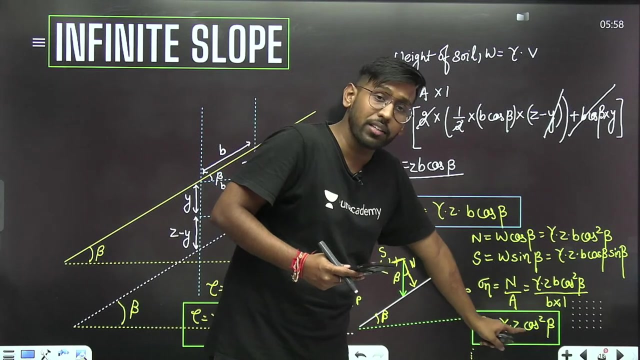 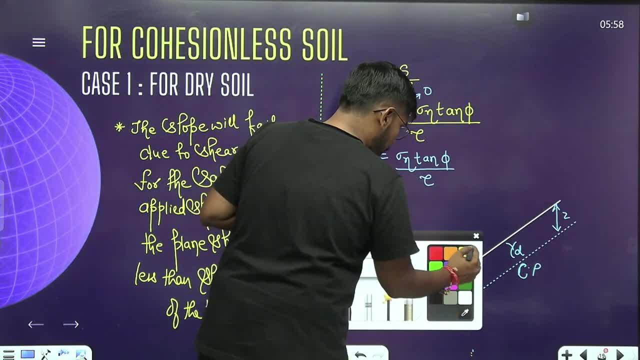 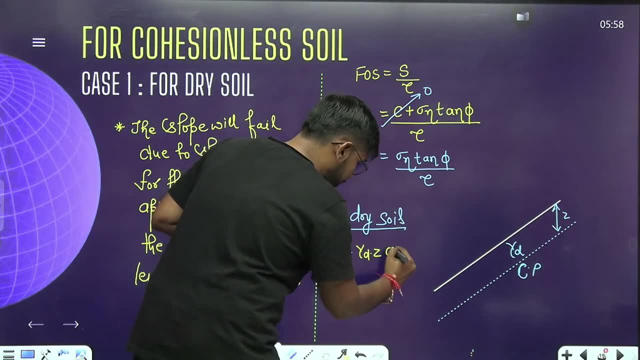 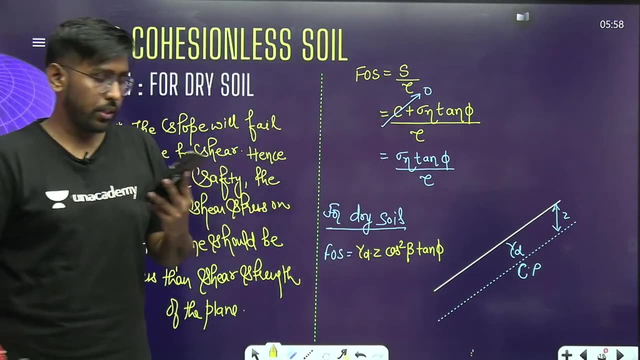 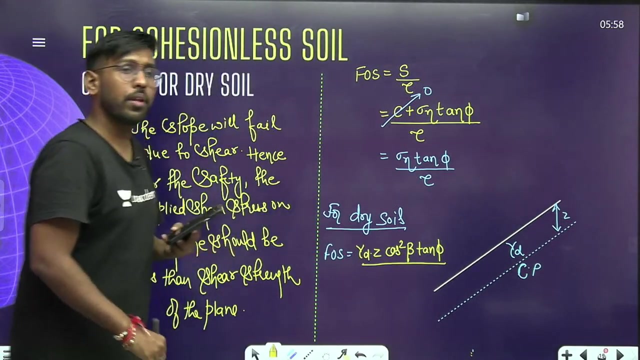 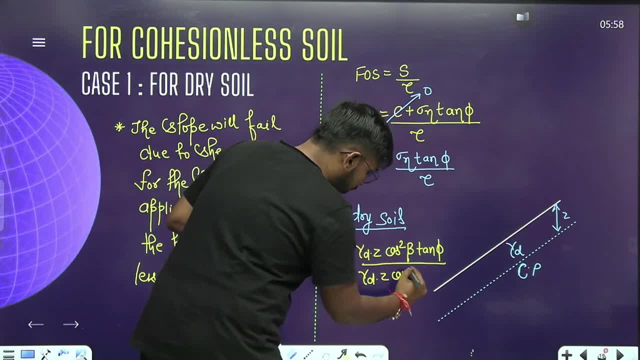 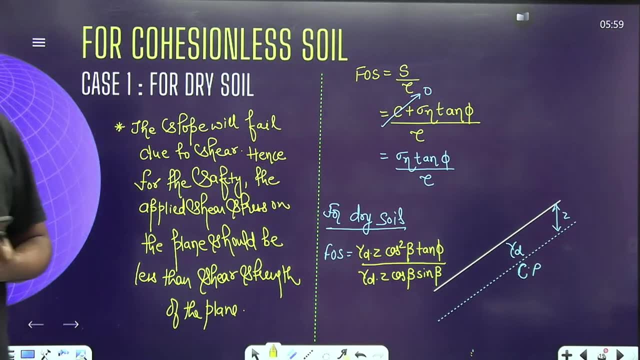 Gamma D into Z Cos beta, sin beta. Yes or no? Tell me yes or no. You can ask me any part which you don't understand. You can ask me any part which you don't understand. There is no part which I haven't explained. 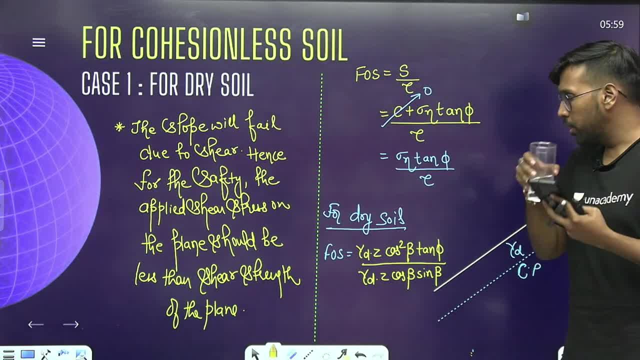 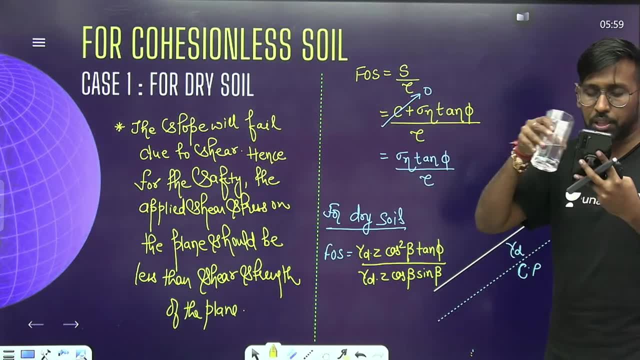 Every part I have explained in a great detail. Every part I have explained in a great detail. Why is this the formula of shear stress? Why is this the formula of normal? This is the formula of shear strength of the soil. I have explained everything. 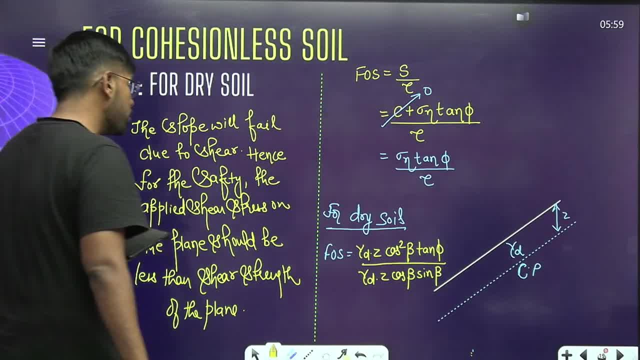 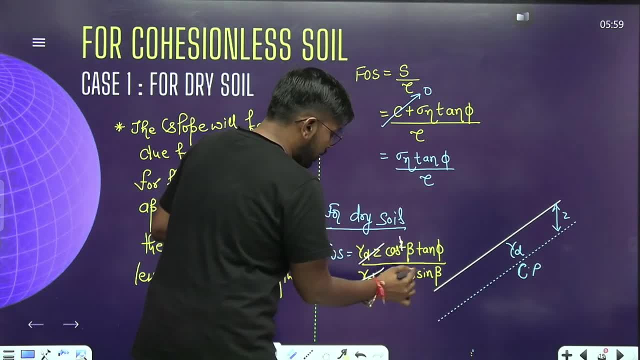 Yes, Now, my friend, Gamma D into Z, Gamma D into Z. This is gone. One cos beta is blown. What happened to sin by cos? What happened to sin by cos Tan beta? What happened to factor of safety Tan phi by tan beta? 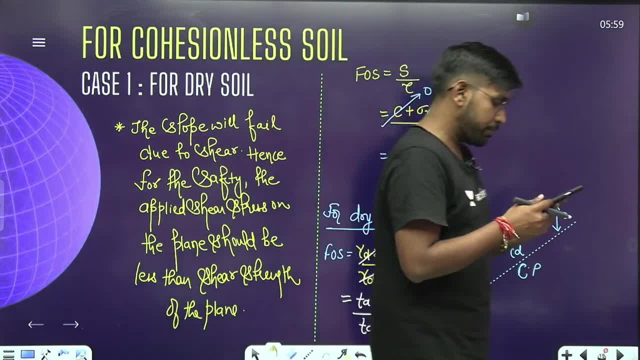 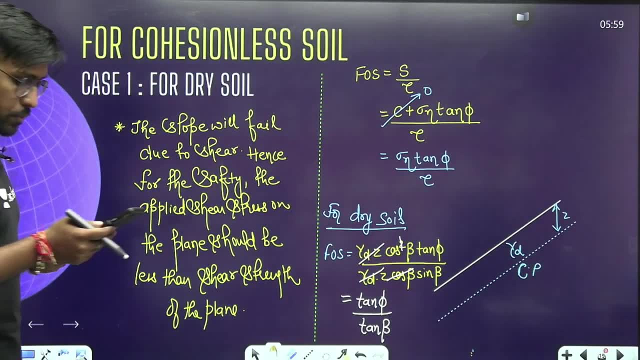 What happened to factor of safety? Tan phi by tan beta. pactrrof safety is tan phi by tan beta. Any doubt in this? Any doubt in this? Tan phi by tan beta, Any doubt in this? What do you say, my friend? 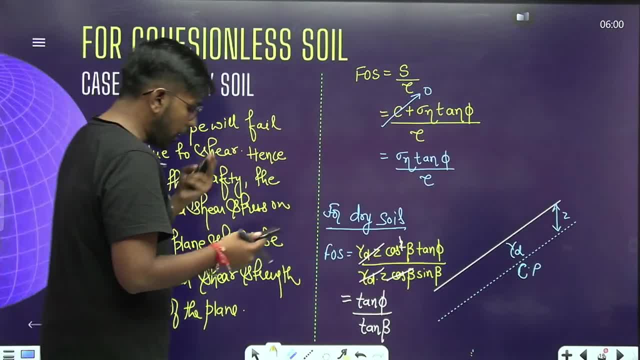 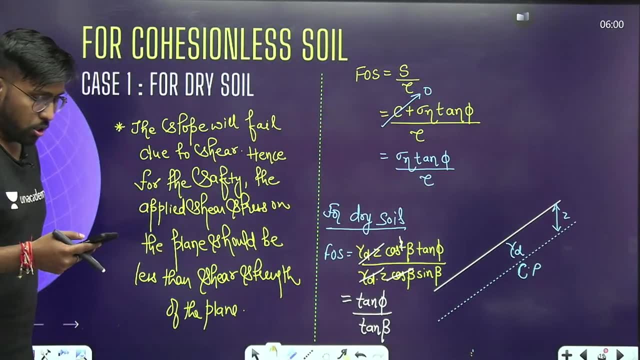 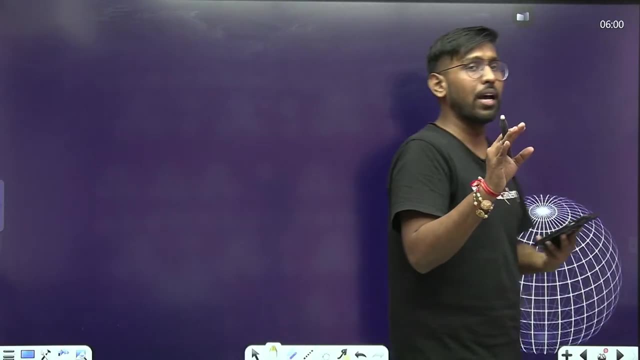 is this point clear to all? is this point clear to all? Do you all understand this point? Yes, Bro, you see you have like and share our video. Like and share the video if you have liked it. yes, now see, my friend, you have a factor of safety. tan pi by tan beta. 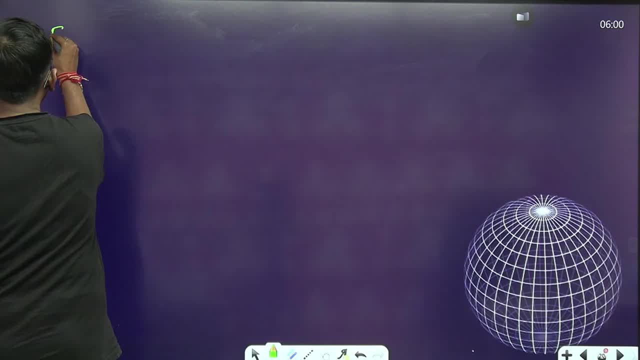 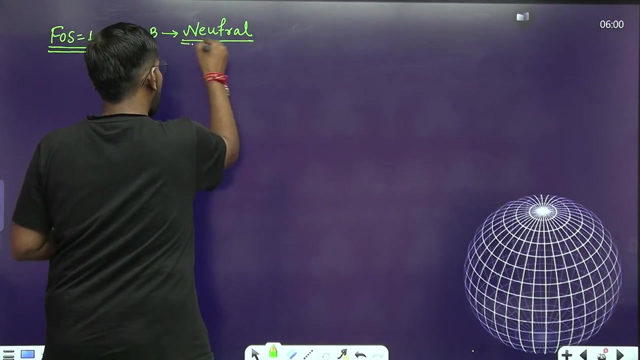 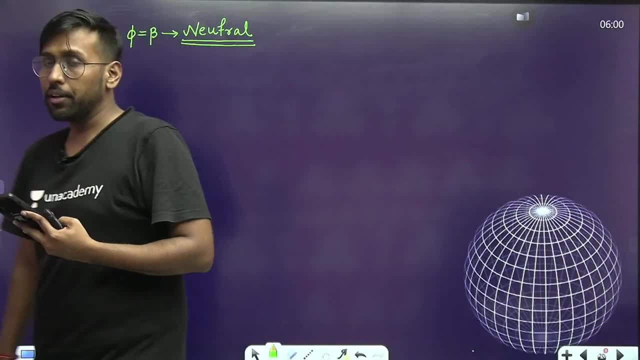 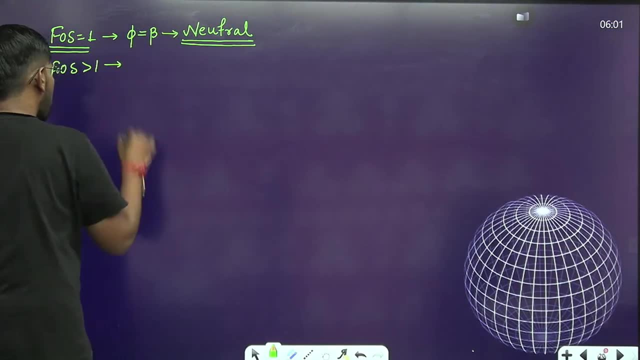 If you have given extra effort, then what will you do? You will fail right. So 5 is equal to beta. If the factor of safety- Sorry, If the factor of safety- is greater than 1, then 5 will be greater than beta. If it is greater than 5 beta, then what will happen? 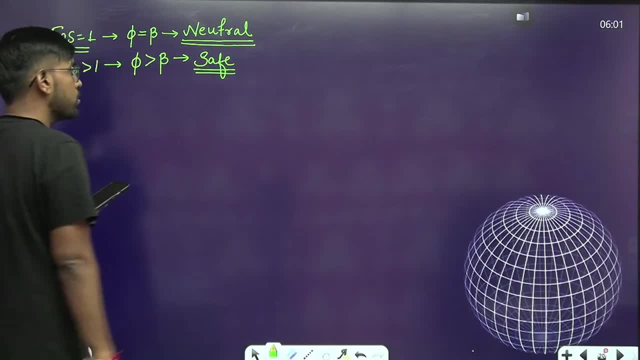 Safe condition. What condition is this Safe condition? This condition is the safe condition. Next, my friend, Factor of safety: less than 1, What will happen in this case? Pi less than beta? Will your structure be fine? Will your structure be fine? Will your structure be fine? 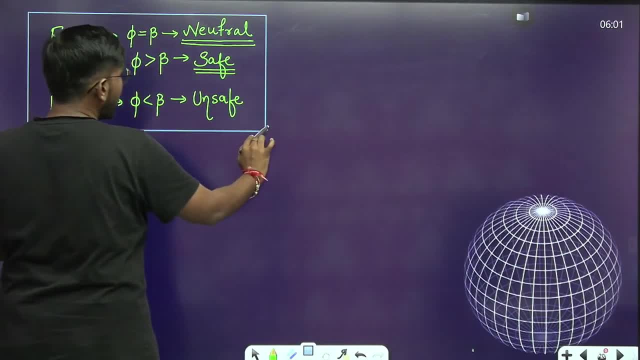 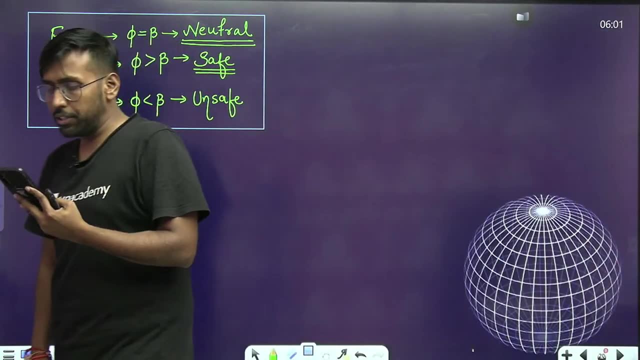 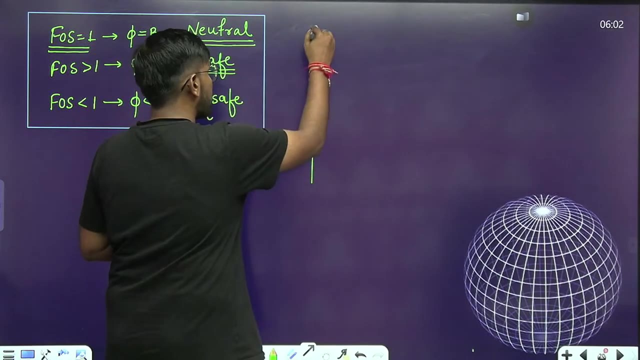 Tell me. This is an imaginary condition. right, Your structure will not be fine. you will provide here, the soil will fall. Yes, it's an unsafe condition. Ok, very good. Now, my dear friend. Now this is explained in the form of a graph. This is explained in the form of a graph. 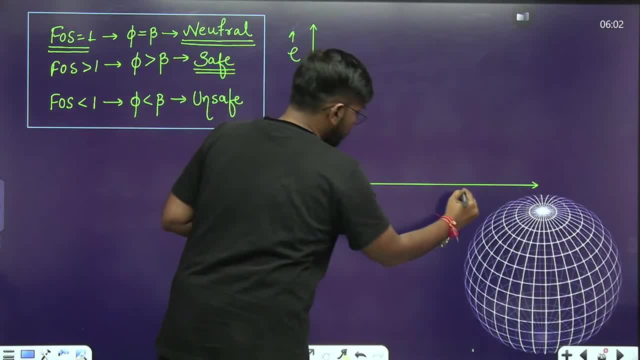 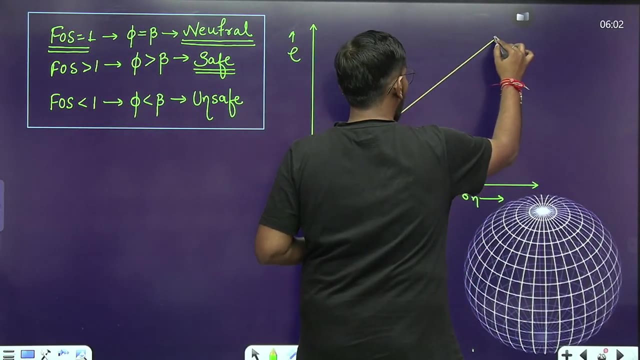 Suppose here your tau is at y-axis, At x-axis is your normal. So if we make more failure envelop for cohesionless soil, So more failure envelop for cohesionless soil. Everyone knows, For the cohesionless soil this will be more failure envelop, Yes or no? This angle is 5. 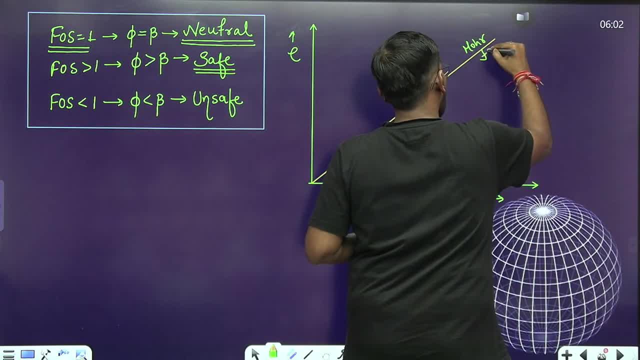 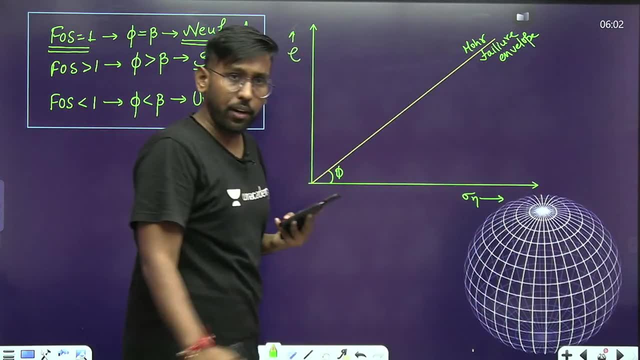 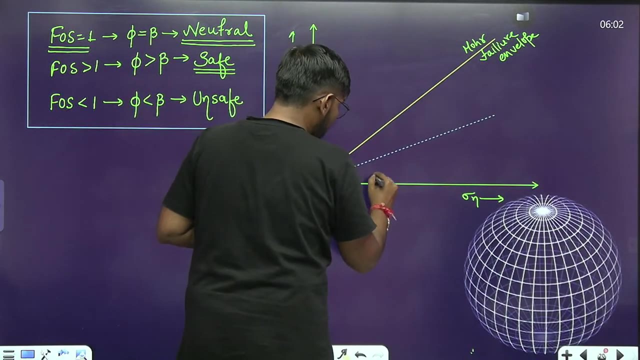 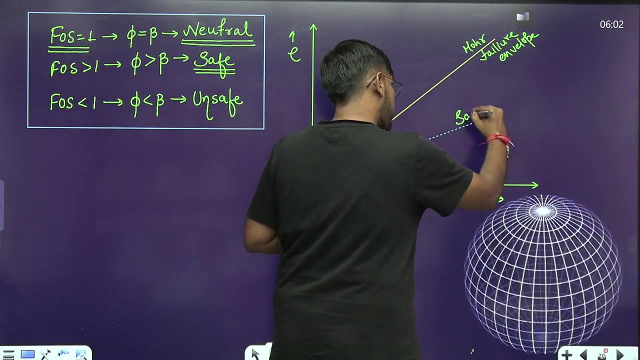 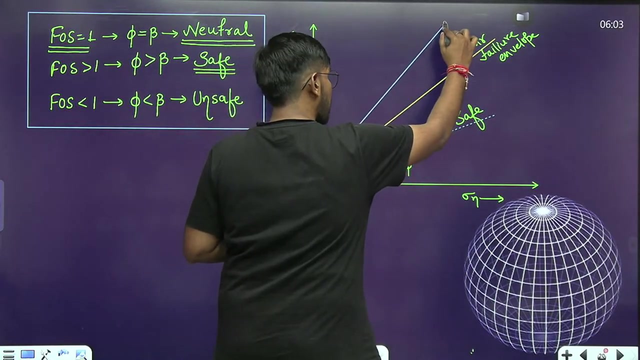 This is your more failure envelop, Right? So, my dear friend, We have three conditions. What are the conditions? First condition: When beta less than 5. So this slope you are giving, What did you tell Safe? Ok, For beta equal to 5 It is unsafe. And for beta greater than 5, 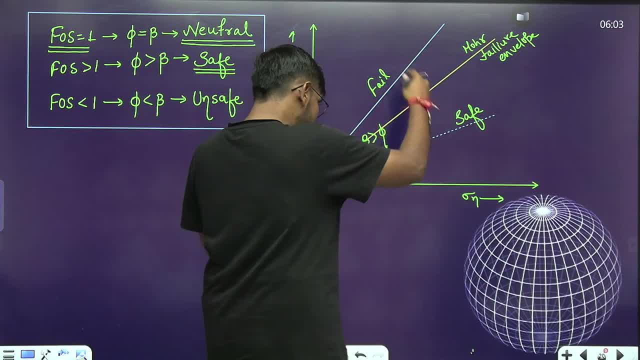 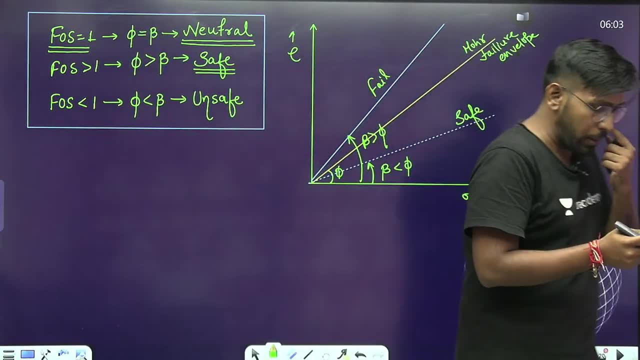 It will be failure condition. Earlier, did you understand all these curves? Earlier, did you understand all these curves? What are you making, sir? I don't understand anything. We used to take ruts. Earlier, what did you do with all these curves? We used to take ruts. 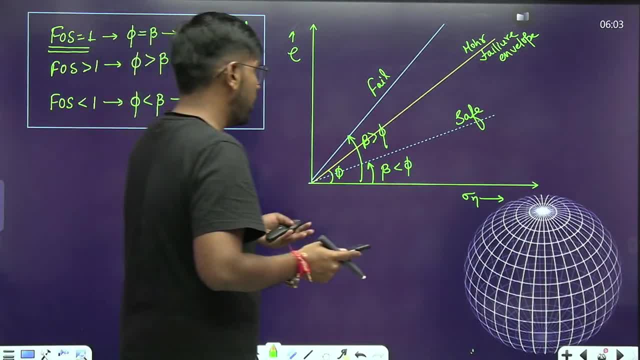 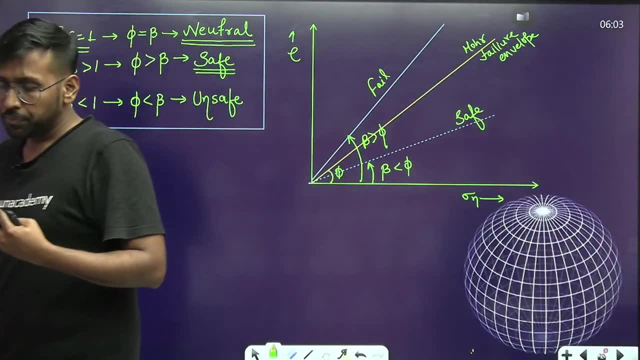 Sir, what are you doing, Sir? I don't understand anything. Sir, I don't feel the air. We used to take ruts. What will we do? If you don't understand, we will take ruts. Is it clear to all now? 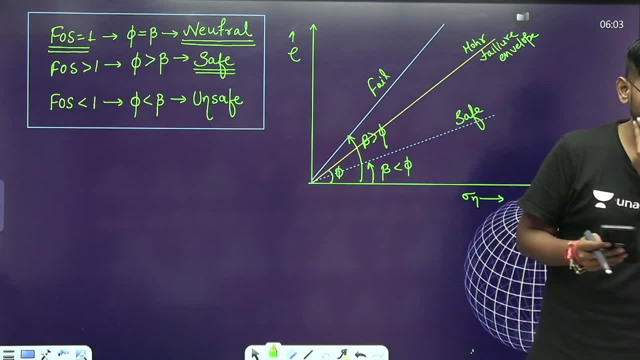 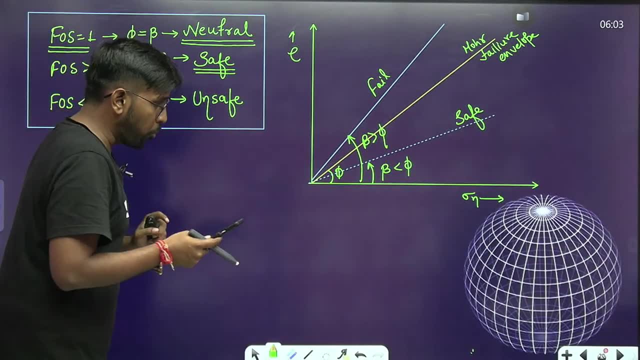 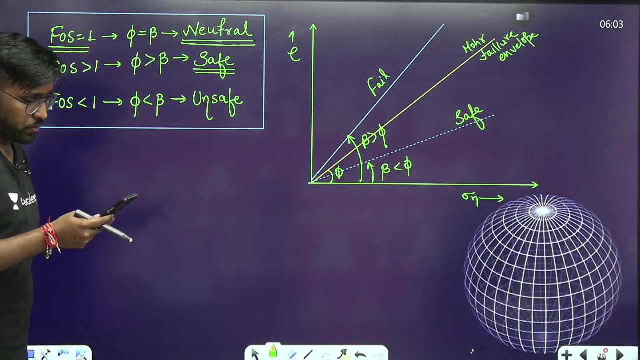 Is it clear to all? Is it clear to everyone? There is something: Everything is very simple. It is a concept to understand. If you understand, then everything is easy. Is it clear? till here? Speak, Speak. Any doubt in this? Any doubt in this? Any doubt in this? 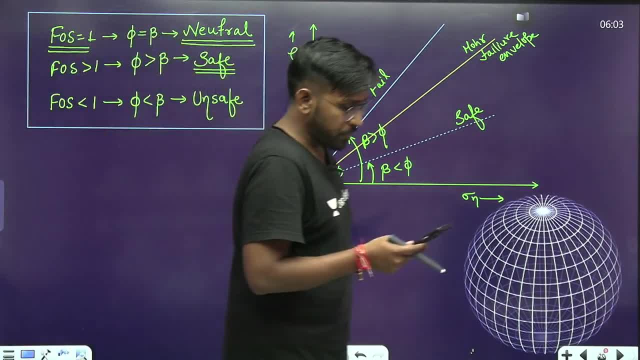 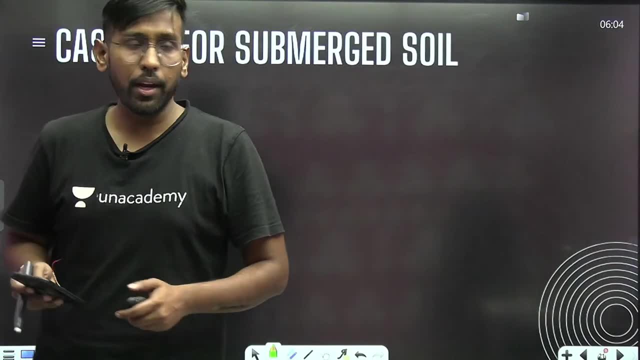 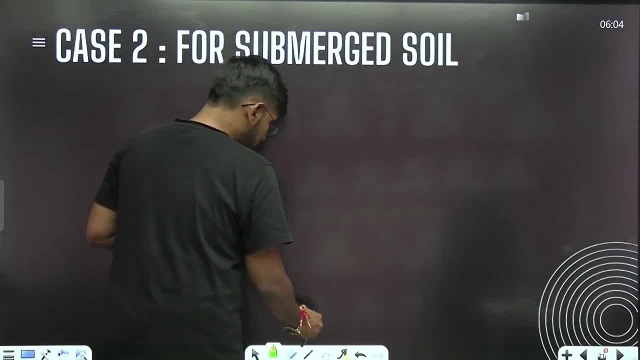 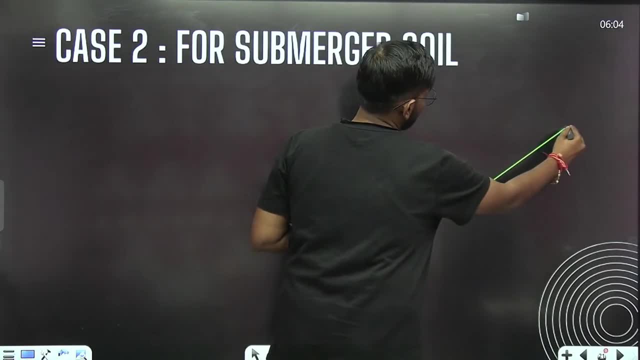 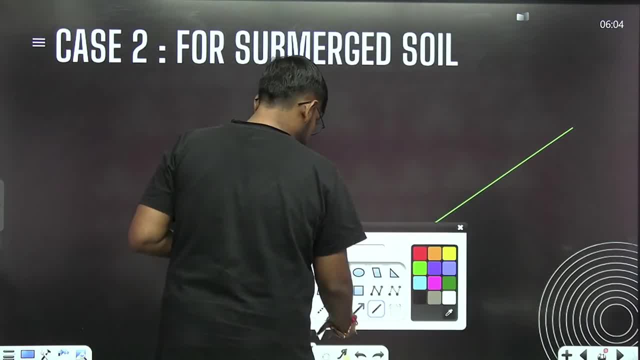 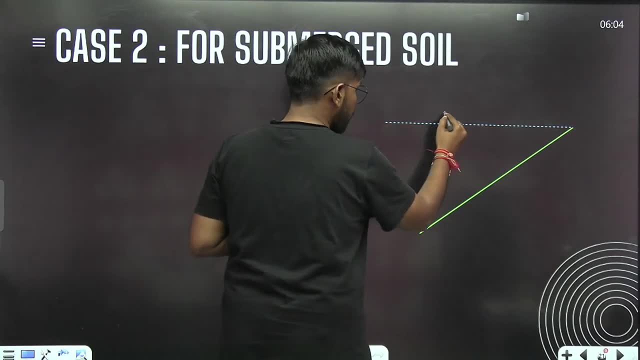 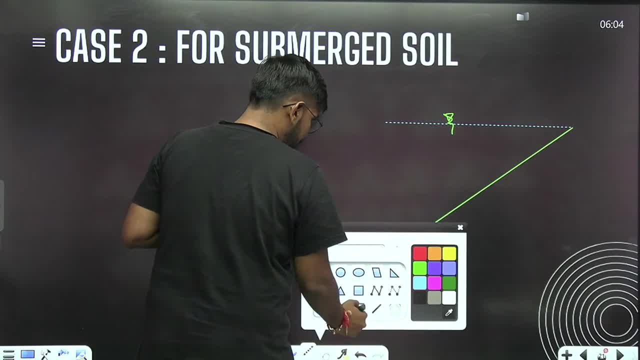 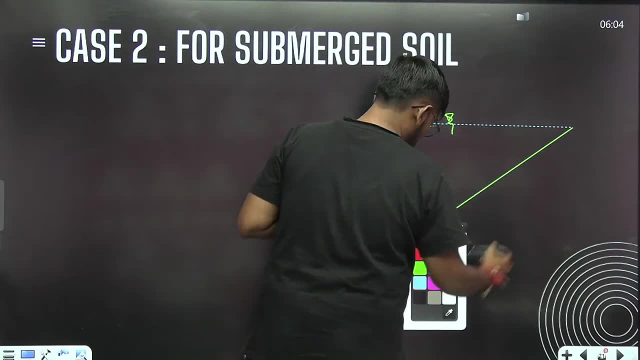 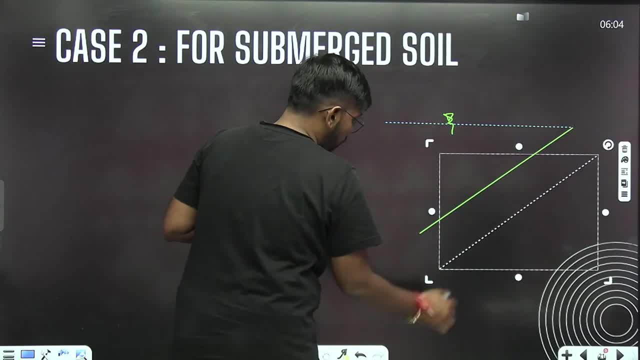 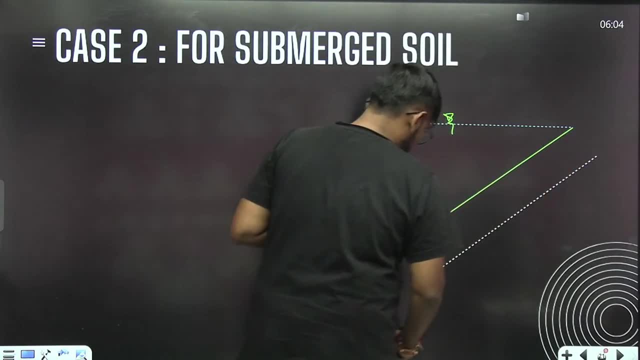 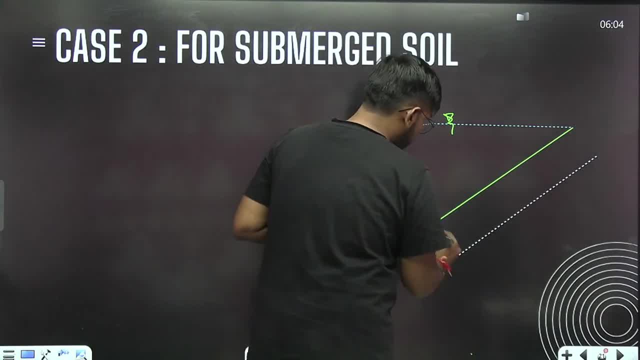 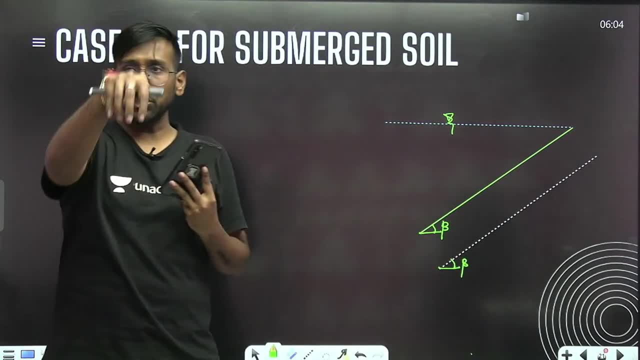 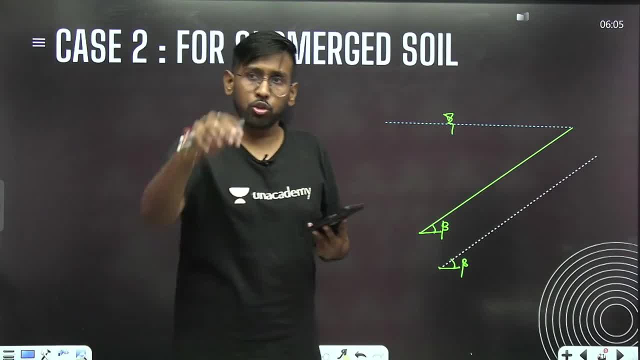 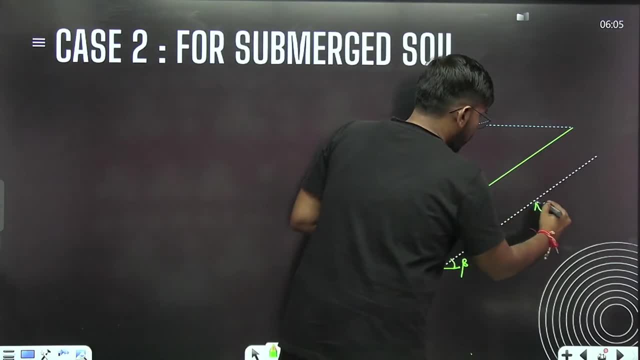 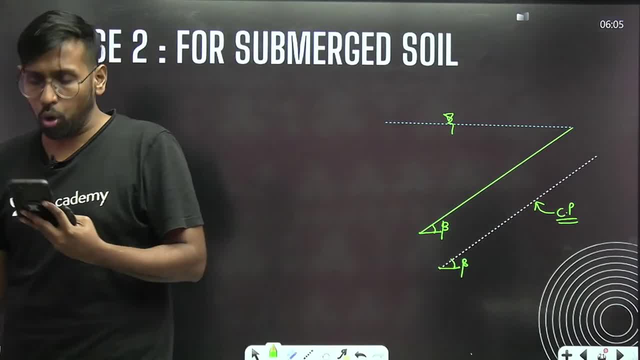 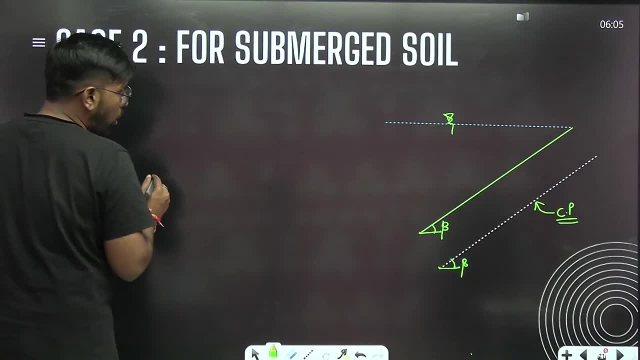 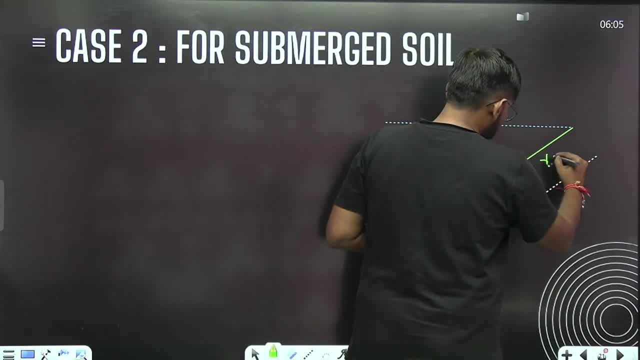 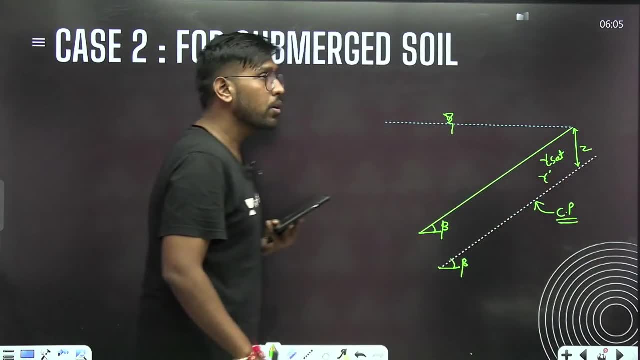 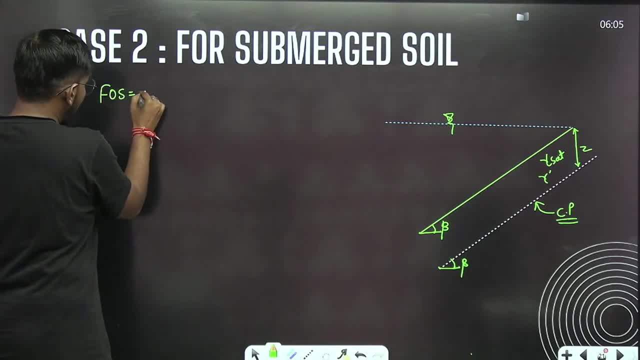 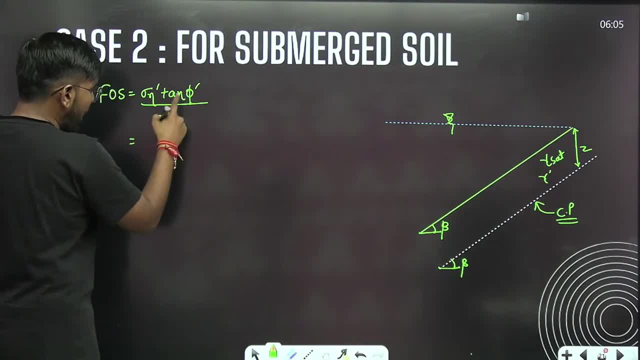 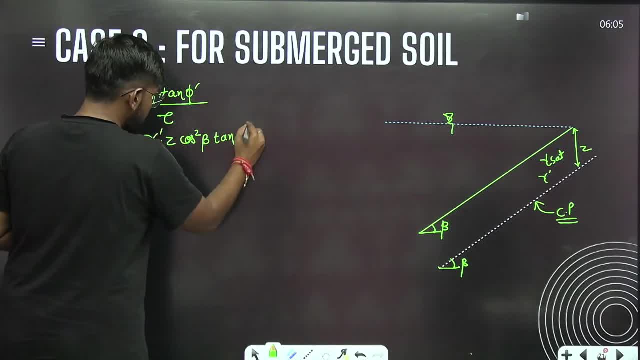 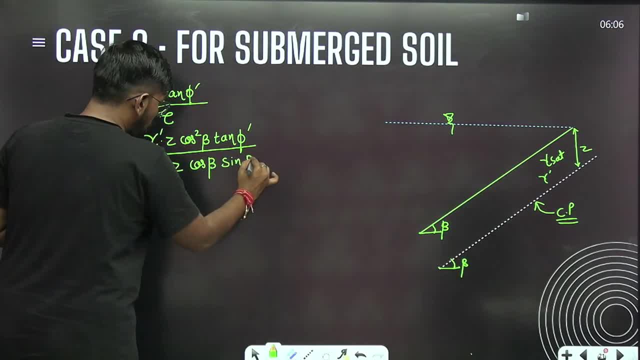 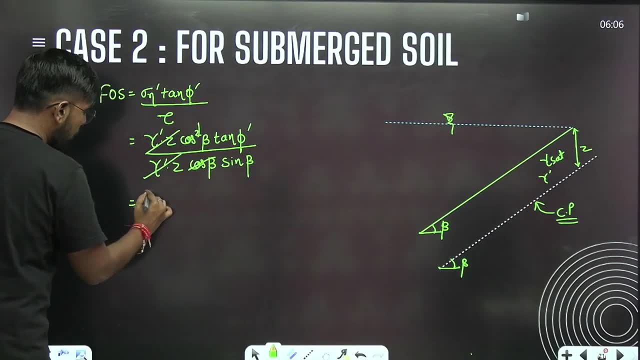 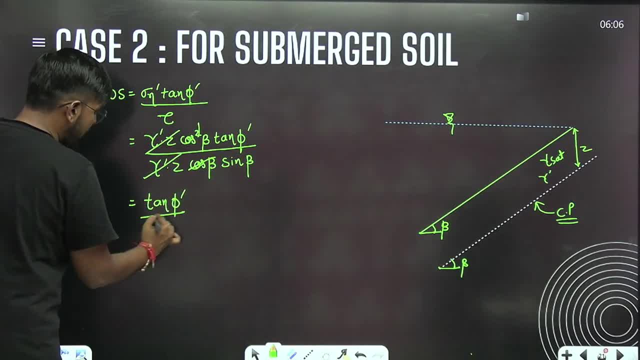 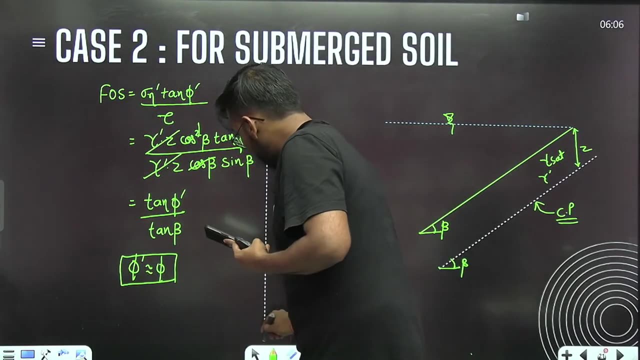 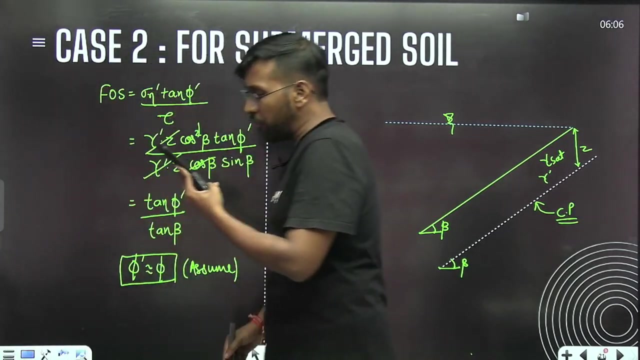 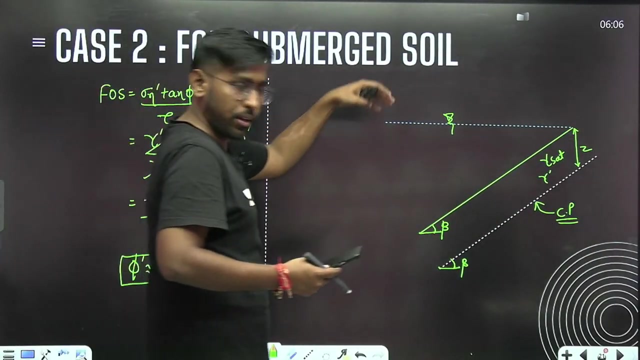 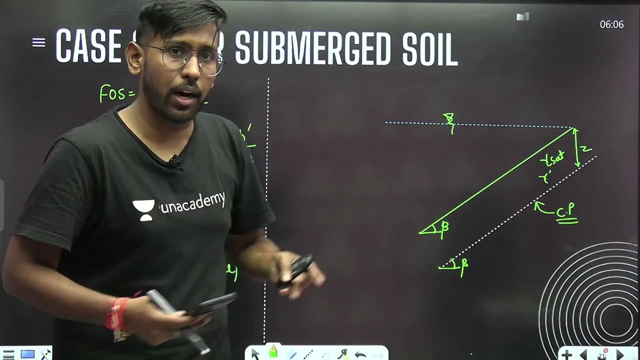 So your answer here is tan phi dash by tan beta. We are assuming phi dash and phi are nearly equal. So can we say that the factor of safety? Who will take the pressure and whose pressure will be applied? Will the pressure of neutral pressure be applied? No, the pressure of neutral pressure will not be applied. 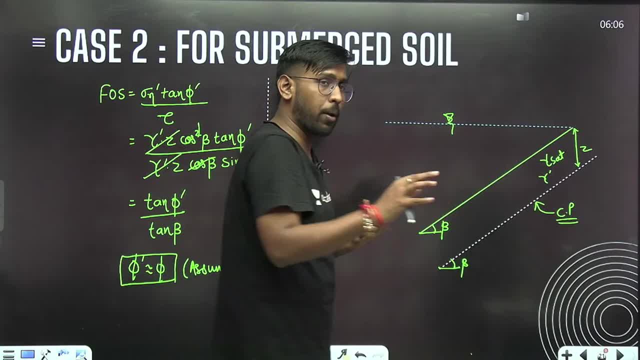 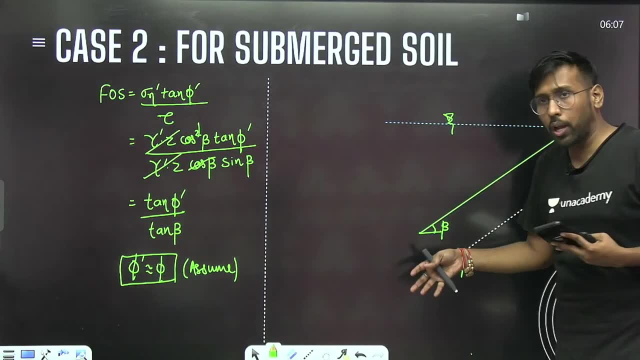 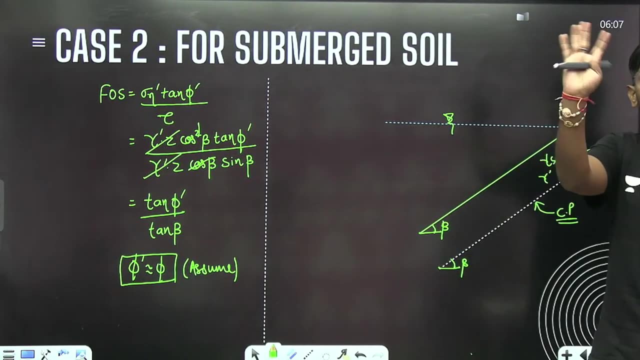 If the water will flow, then the pressure will be applied. If the pressure is equal everywhere, Then the force will not be applied. the flow will not be there. If the soil is submerged, we will assume that there is no flow of the soil, And if there is no flow of the soil, then there will be no pressure. 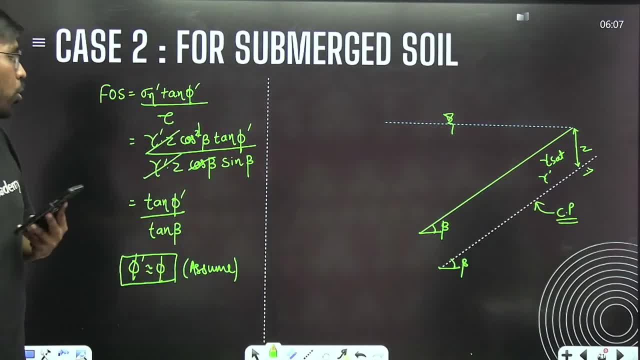 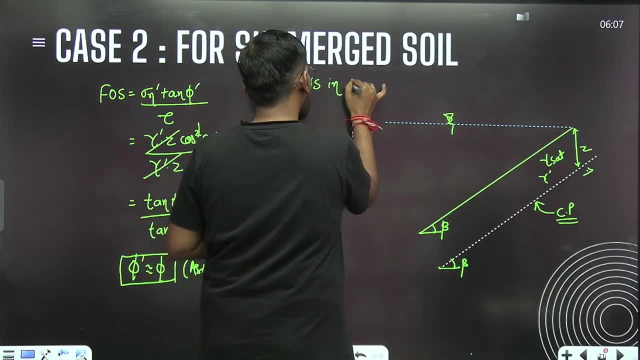 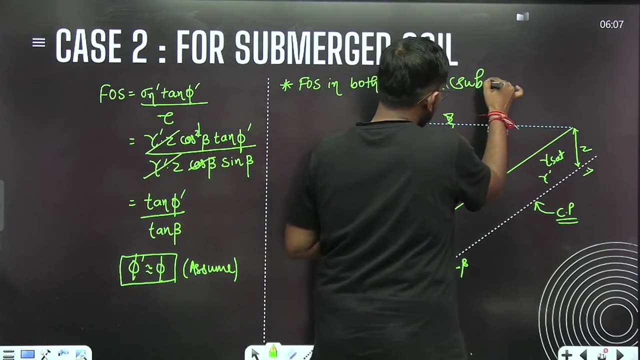 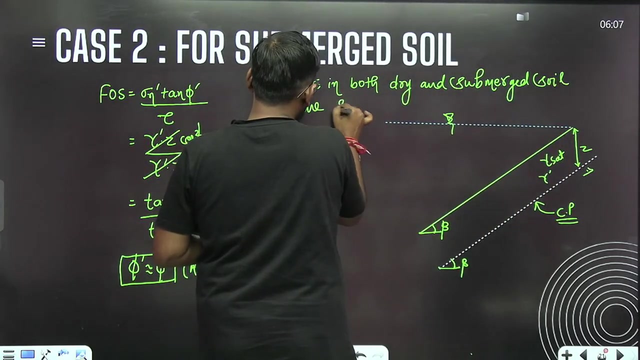 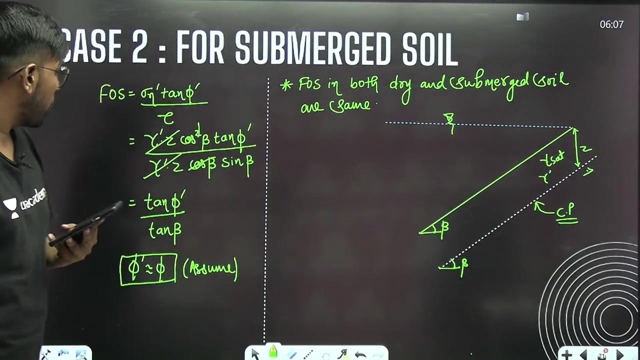 Is it clear. There will be no pore water pressure. So what we are saying here is that the factor of safety In both dry and submerged soil Soil are same. Both dry and submerged soil are same. What will happen in both, my friends? What will happen in both. It will be equal. 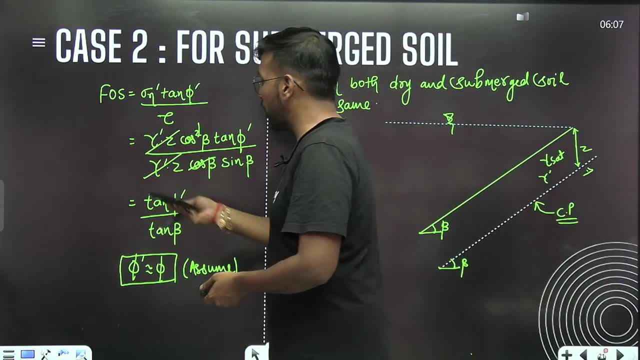 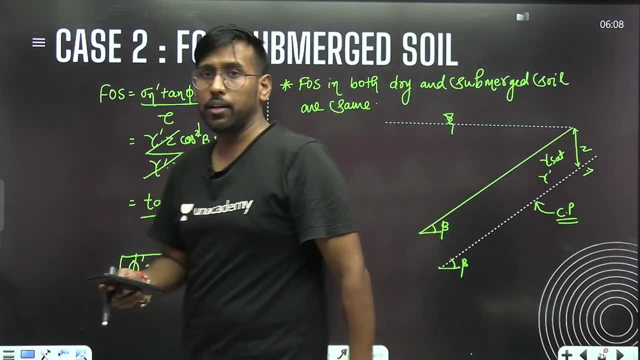 What beta, brother? Who are these phi and phi dash saying? If it is equal, then the matter is different. To compare, these phi are written for dry. These two are written to compare. We are not equating the beta. Is it clear? till here, Yes, 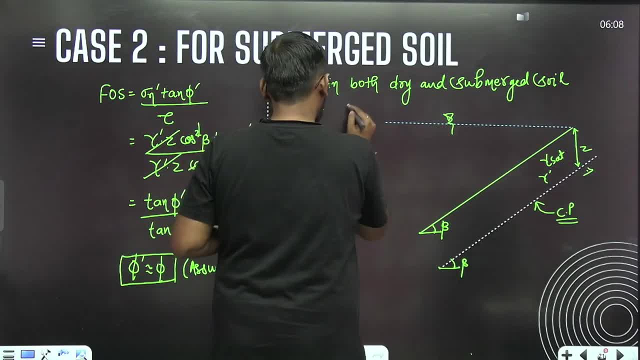 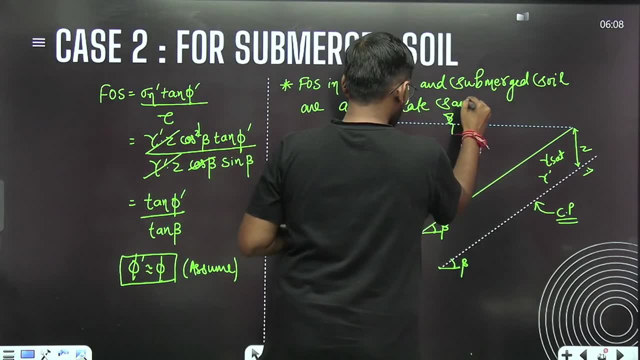 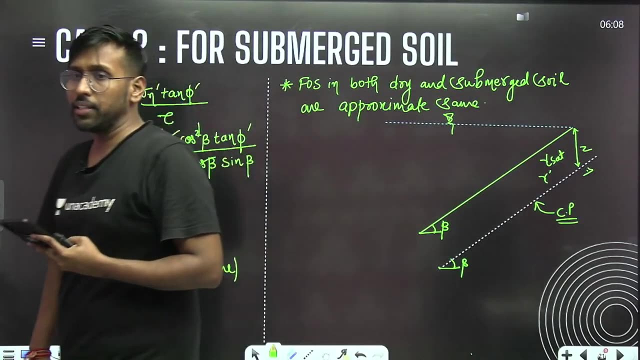 Write here: are approximately same. Otherwise you will say: sir, it is not same, Are approximately same. Ok, So that is your case no.2. Does anyone have any doubt till here? Does anyone have any doubt till case no.2?? Does anyone have any doubt till case no.2?? 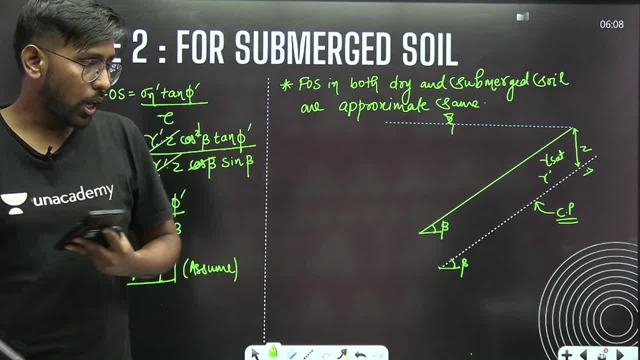 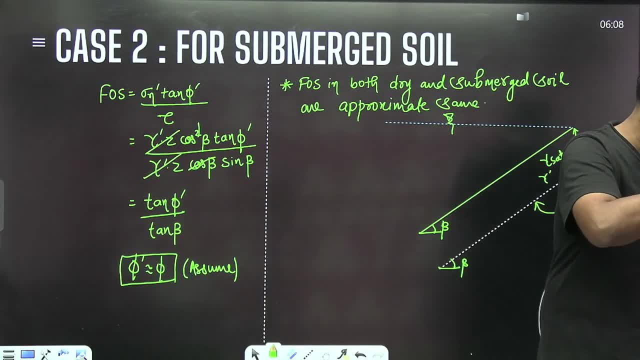 Does anyone have any doubt till case no.2?? Because now we are going to have fun. We are going to do the part Which is the most liked topic of GATE. Now we are going to do the topic Which is the most liked topic of GATE. 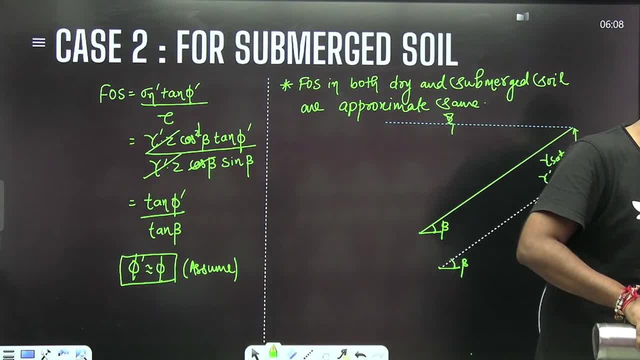 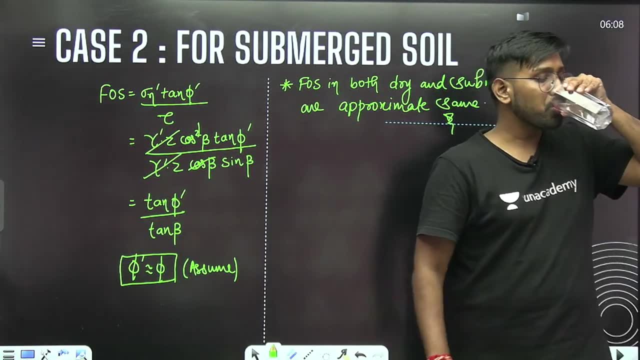 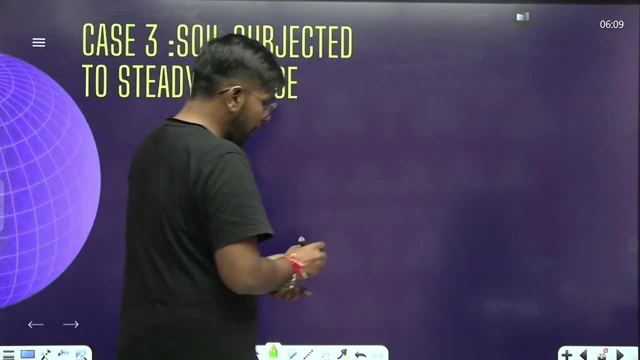 The topic that is asked the most in GATE, Which is the most liked topic of GATE, Which is the most liked topic of GATE, GATE, GATE, Mere dhost Chali Mere dost. Now we are going to talk about soil subjected to steady seepage. 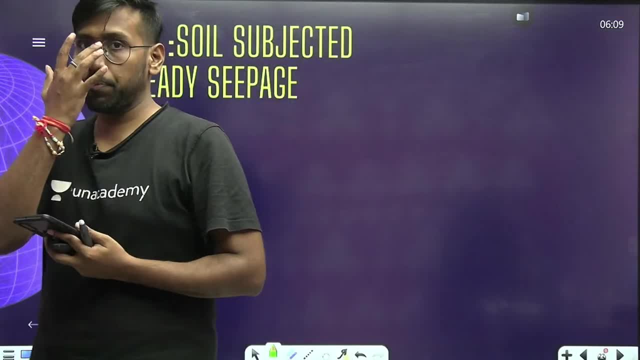 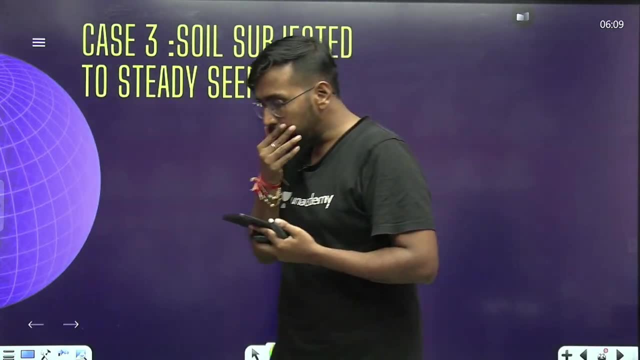 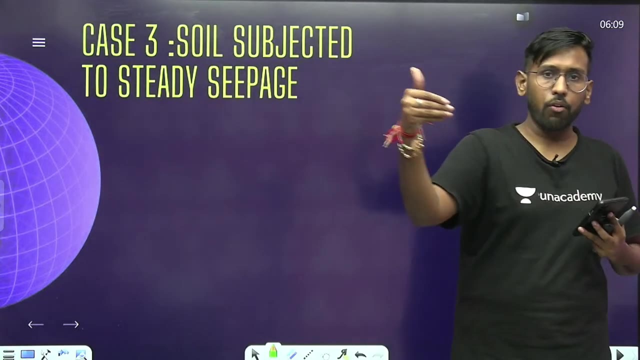 If we don't consider soil submerged. soil is not submerged. Soil is not submerged. Soil is not in a submerged state. If it is not submerged, then what will happen? Water will flow along the slope due to its weight. There will be difference of the pressure. pore water pressure. 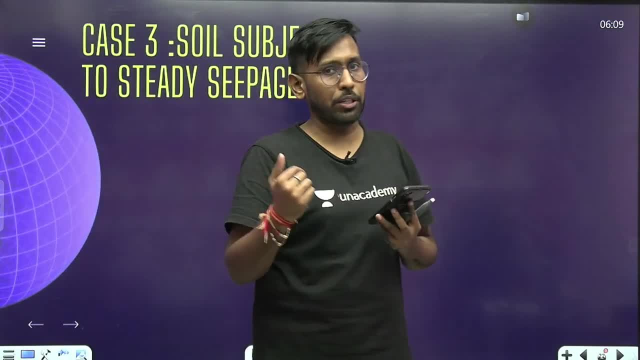 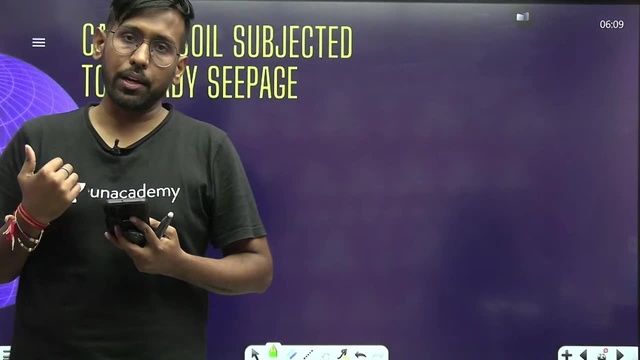 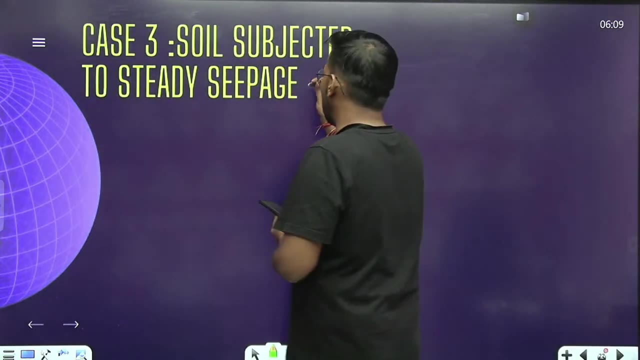 Pore pressure will be different, There will be difference in pressure And due to difference in pressure, the flow will be seen in the water. The water will flow through the soil, along the layer. So you can see this thing. So the next reason is for soil subjected to steady seepage or 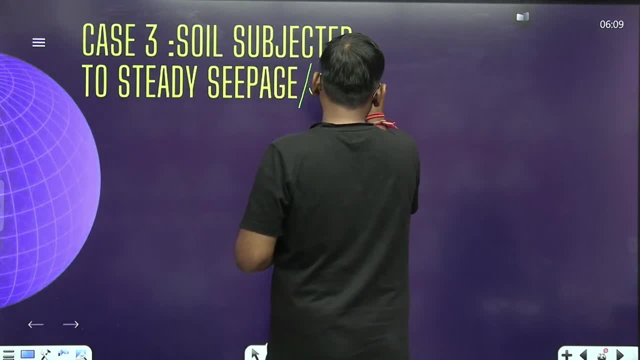 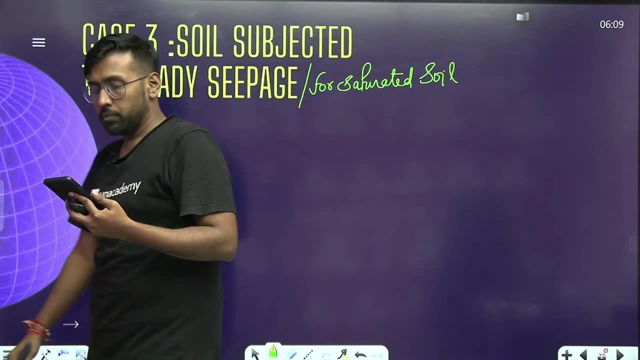 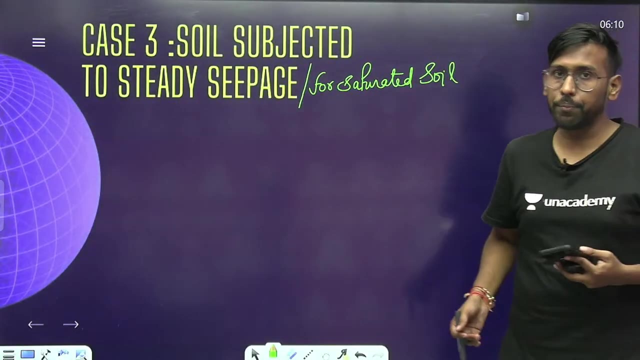 here. you must have seen many cases For saturated soil. Now we are talking about cohesionless, Everything is happening for cohesionless, Everything is happening for cohesionless, And this is an interesting topic. This is an interesting topic, So listen very carefully. 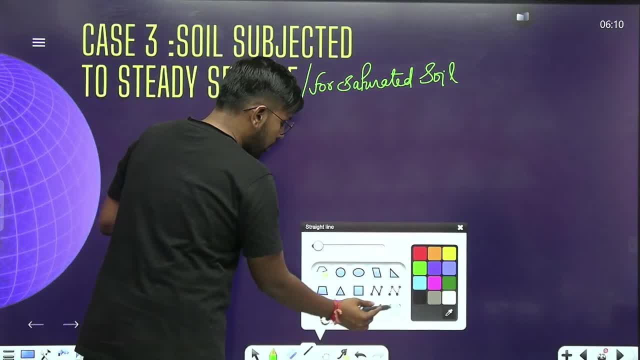 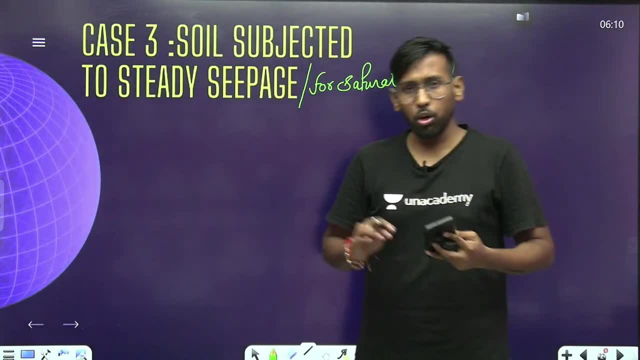 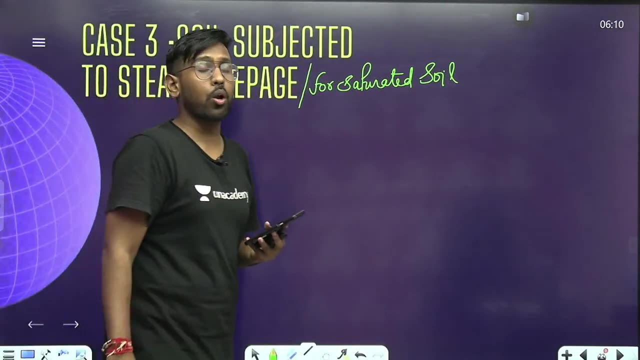 Listen very carefully, My friends. what will happen here? Water will flow In the submerged soil. the flow was not there Because there was no head difference. What is here? There will be head difference. Here. you are going to observe the head difference. 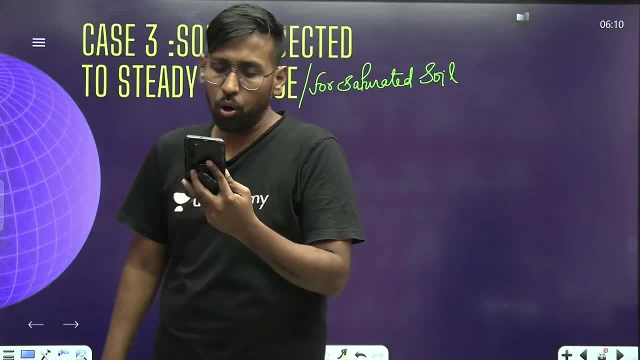 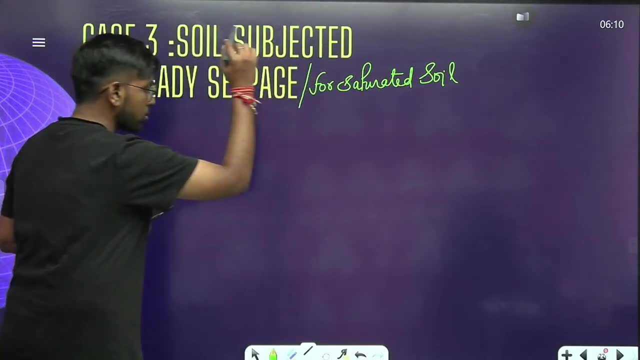 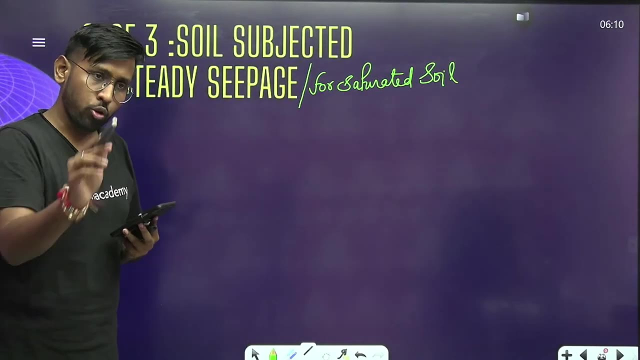 Because of which the flow will be seen, Because of which the flow will be seen. So you will understand this thing very carefully, My friends. I am going to tell you this thing. I have not told you this till today, And it will not be found in any book. 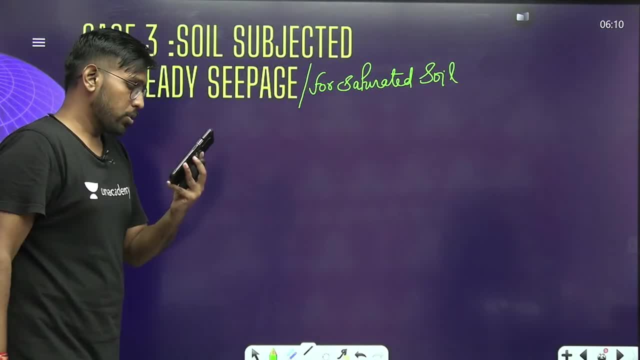 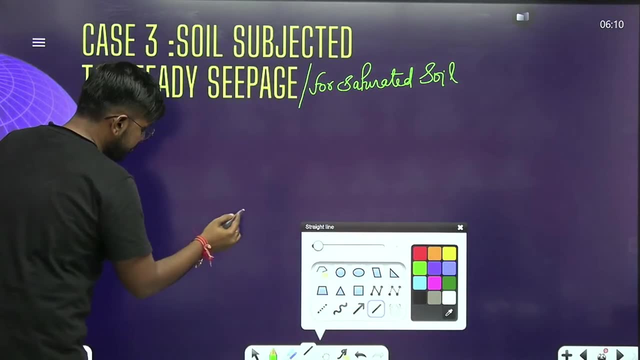 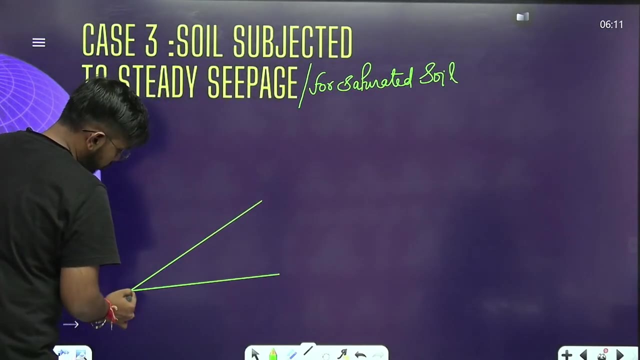 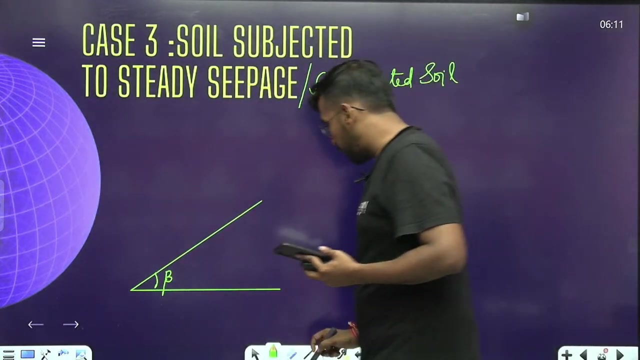 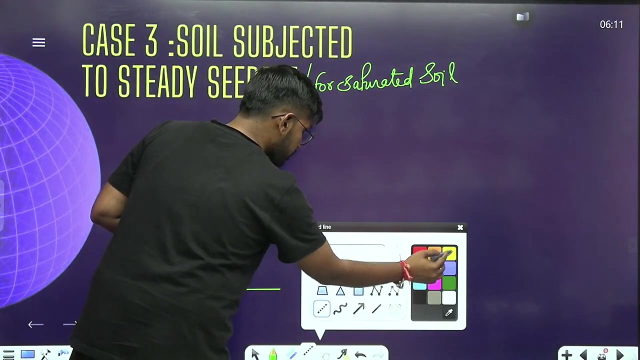 So please keep your focus here. Only then you will understand. Okay, Please maintain your focus here, Look here. So this is the slope beta. What is this slope Beta? The slope is beta. Now, my dear friend. Now, my dear friend. 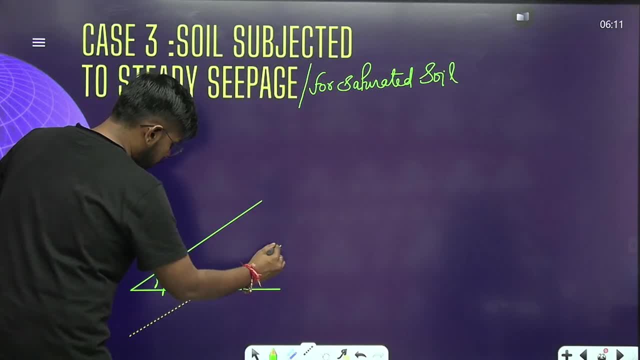 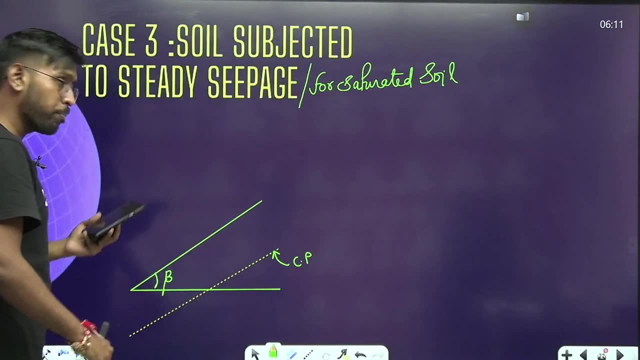 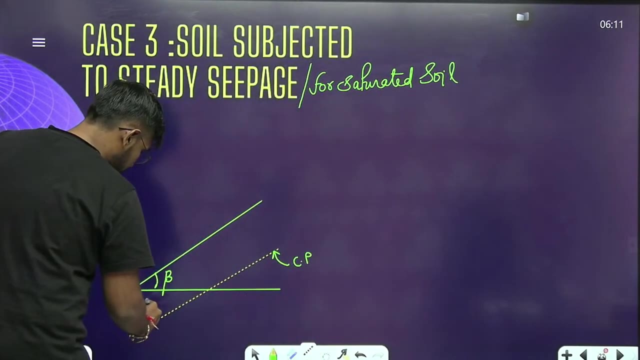 Okay, Let us say This is your failure plane Or critical plane. This is the critical plane, My dear friend. My dear friend, Let us say: This is the water table. This is your water table. Okay, This is your water table. 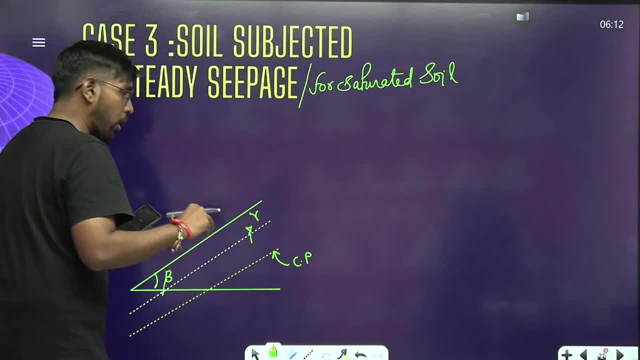 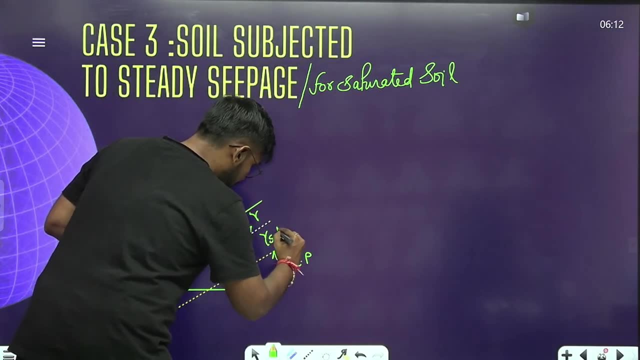 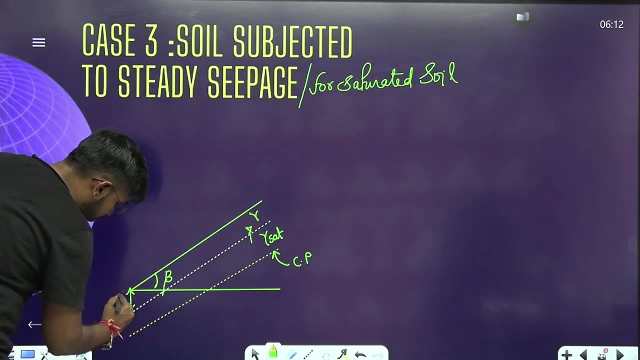 Right Now, On this, the weight density can be in soil, dry condition or in moist condition. Below this, the weight density is gamma psi. Okay, Below this, the weight density is gamma psi. So now, my dear friend, We are saying this height is z. 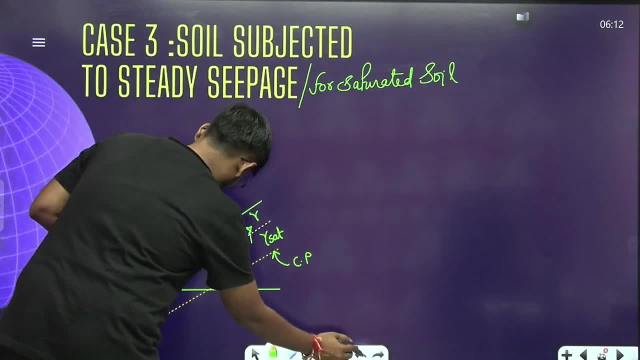 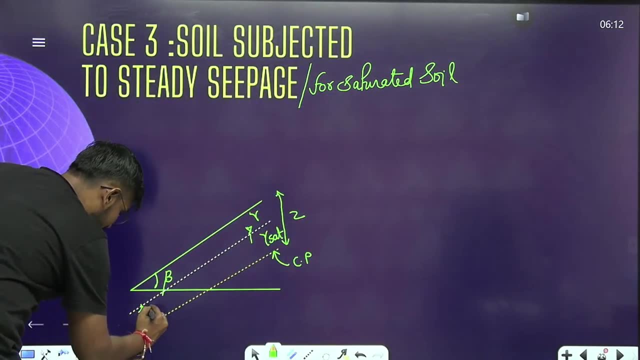 And we are saying the other height, Or If we say that the total depth is z, Okay, This height is h. So the remaining height, The remaining height, That will be what z minus h. Any doubt till here? Any doubt till here? 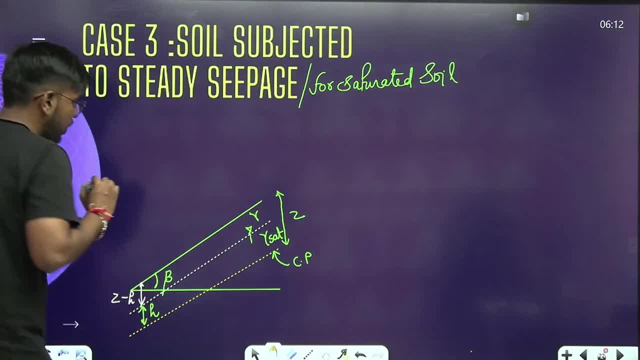 Tell me, my dear friend. So here We will do total stress analysis. The analysis of the pore water pressure will be different, The analysis of the total pressure will be different. How will it happen? Why will it happen? I am also telling you this: 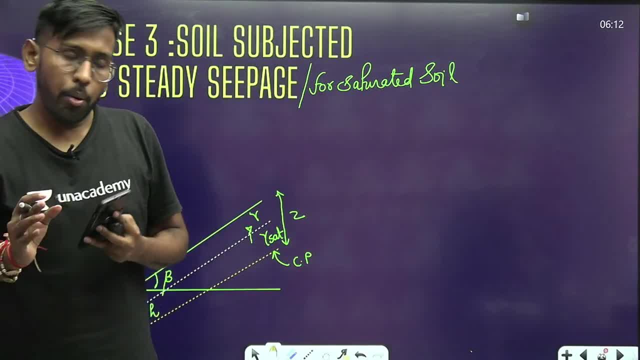 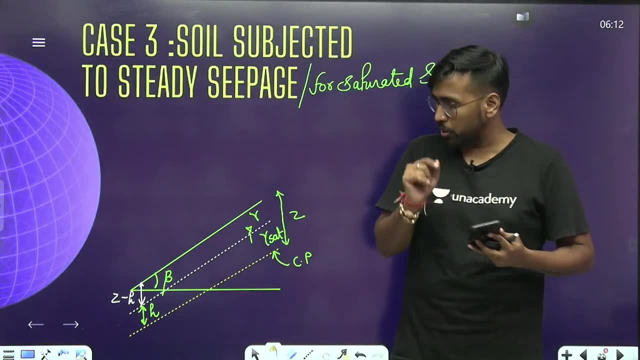 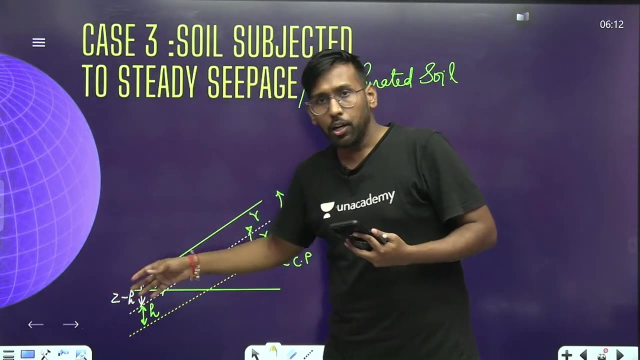 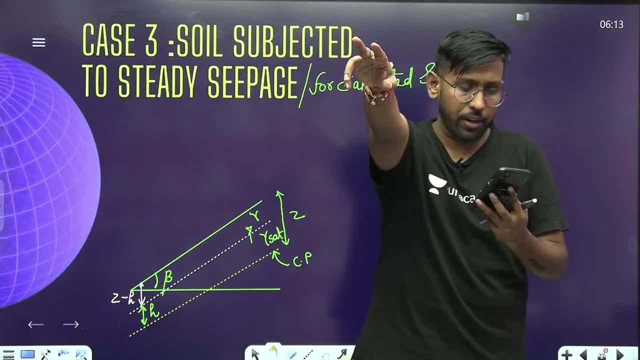 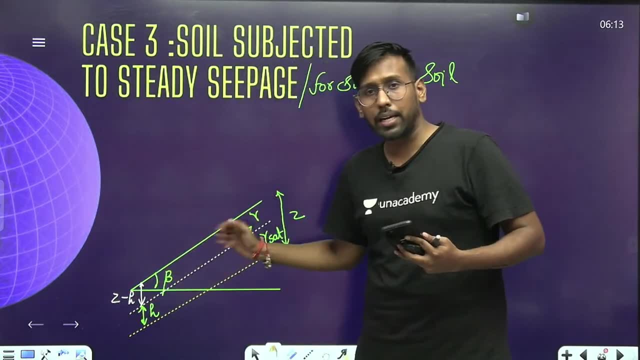 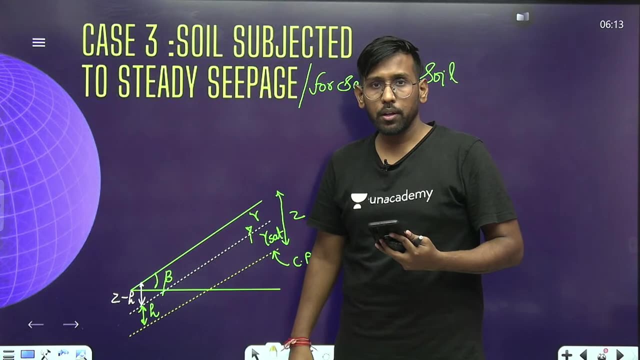 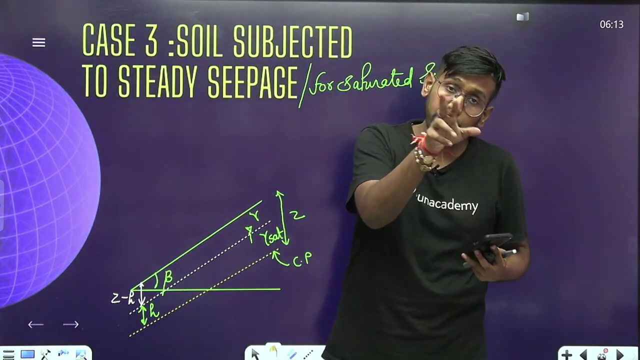 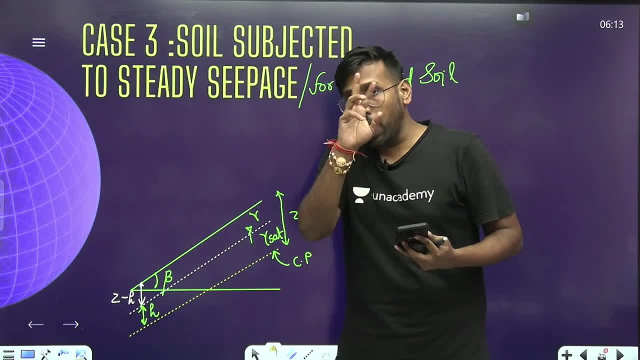 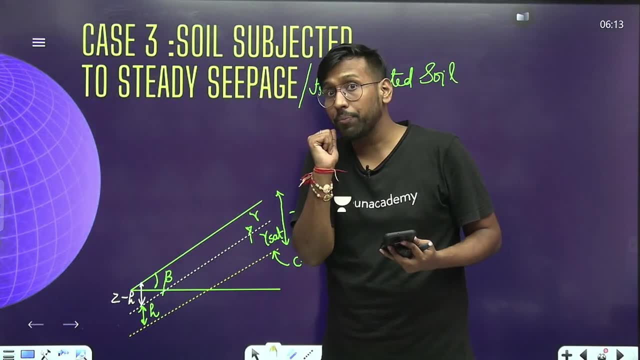 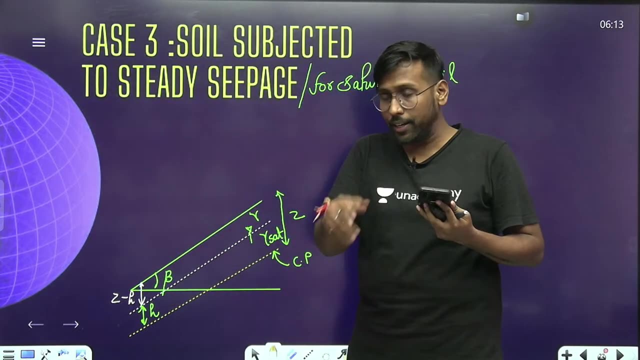 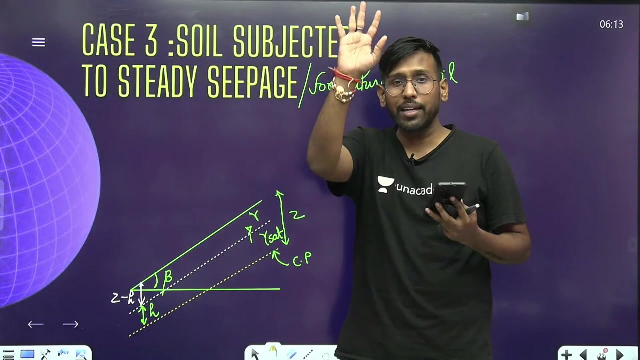 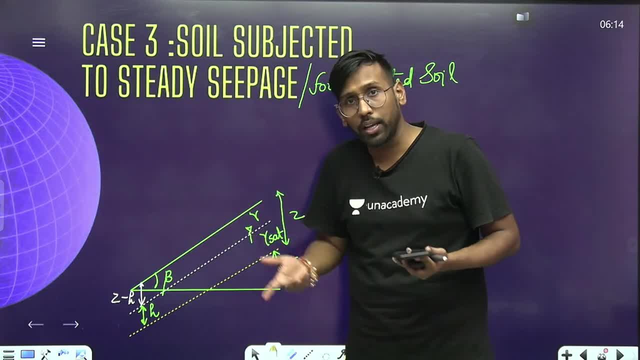 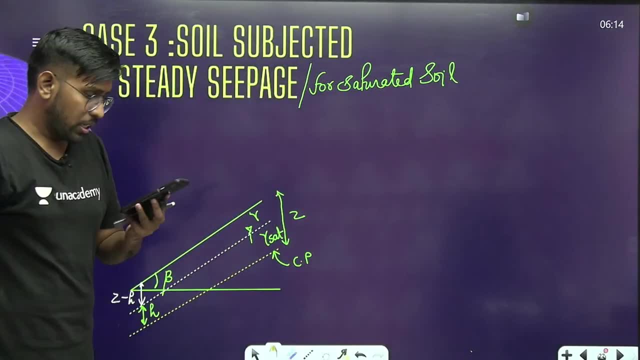 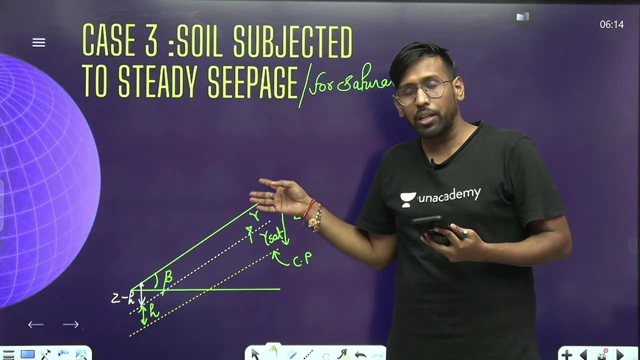 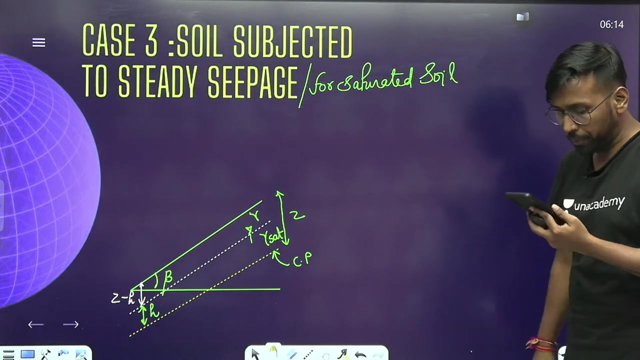 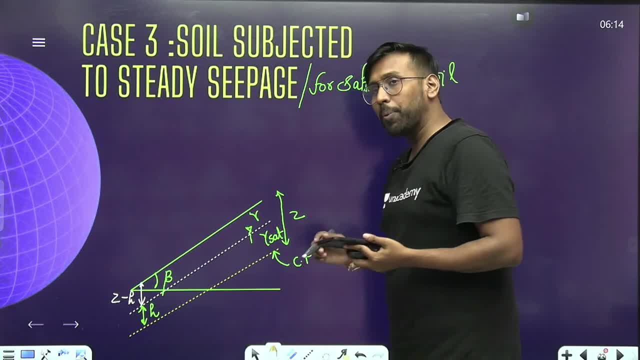 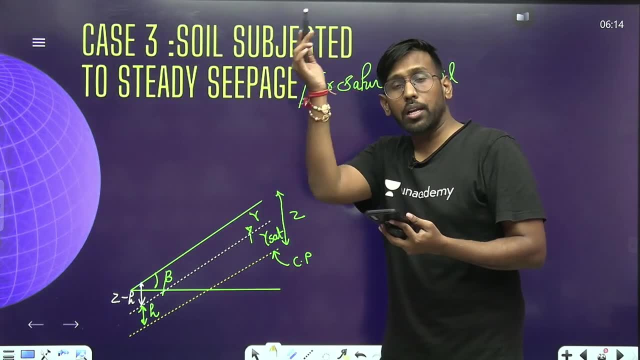 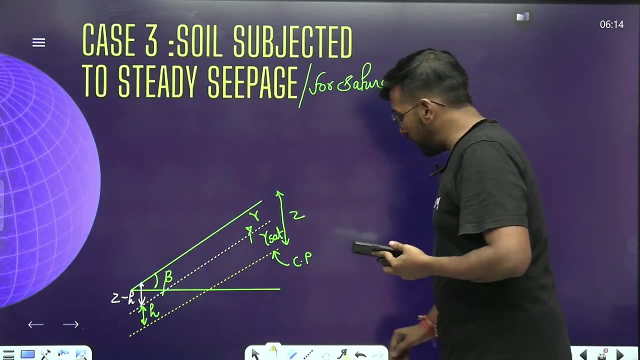 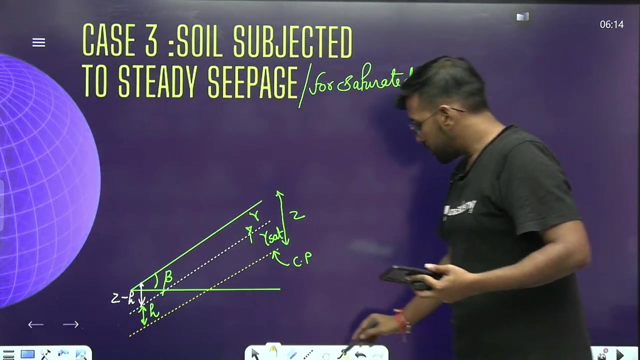 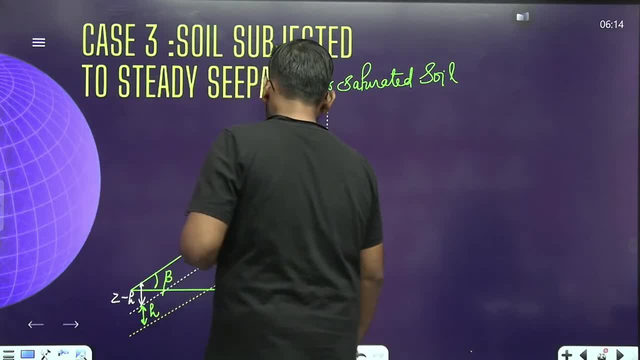 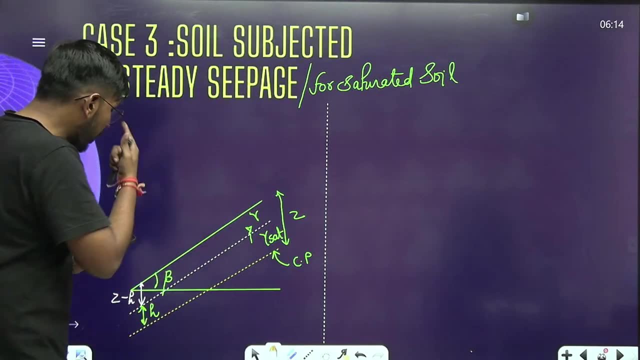 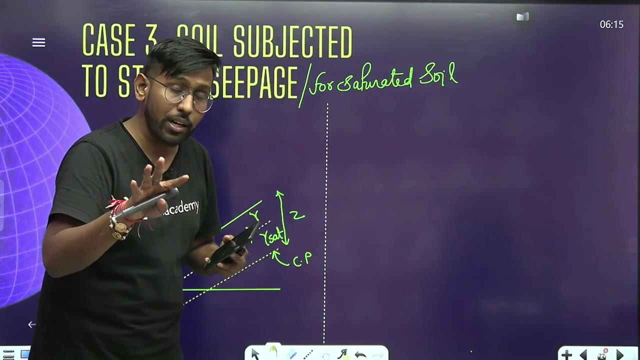 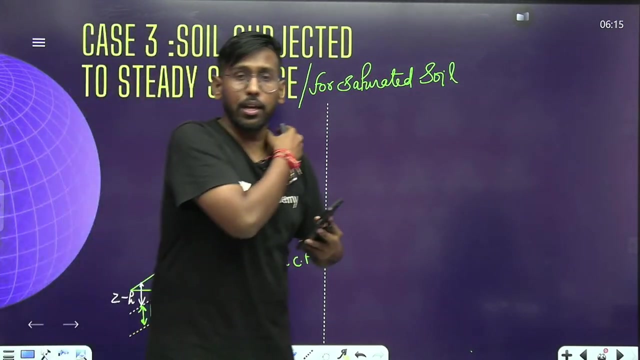 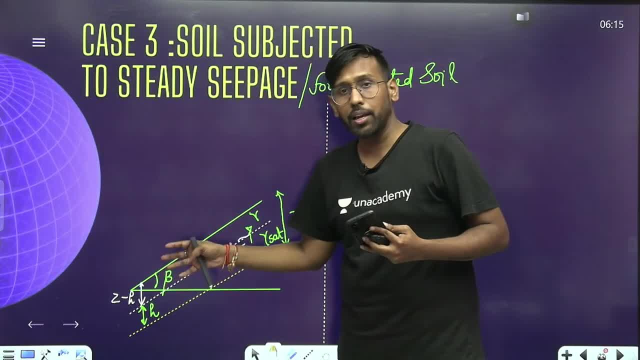 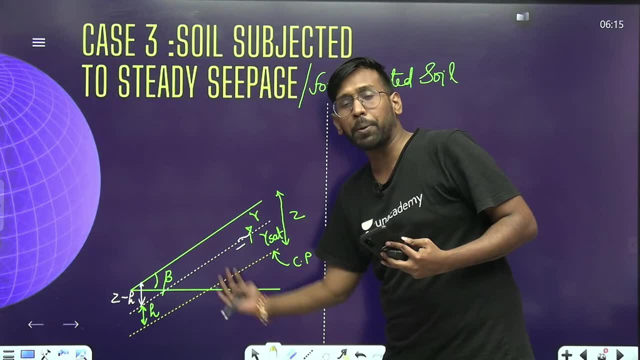 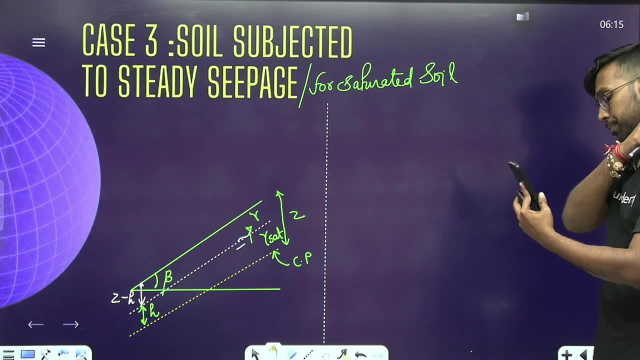 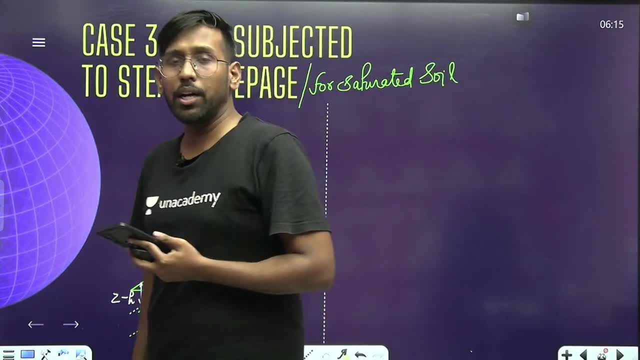 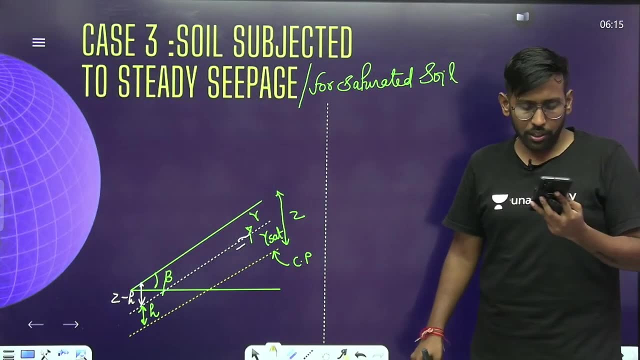 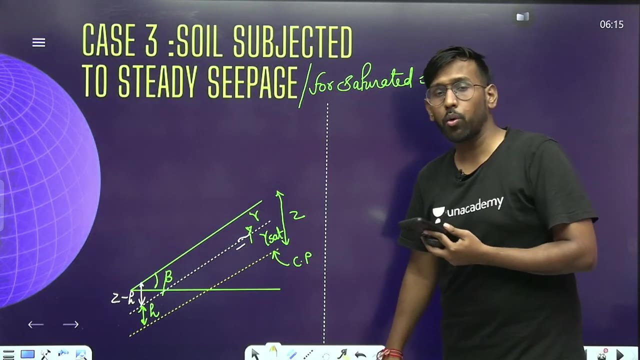 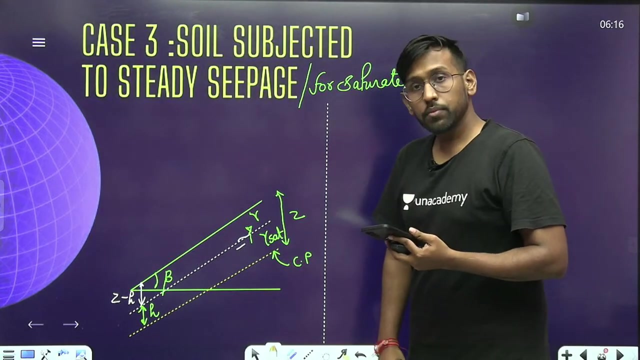 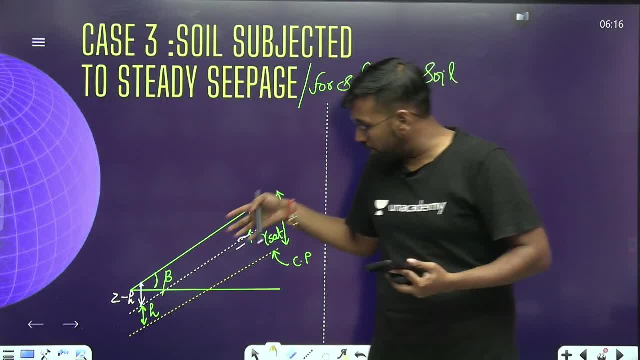 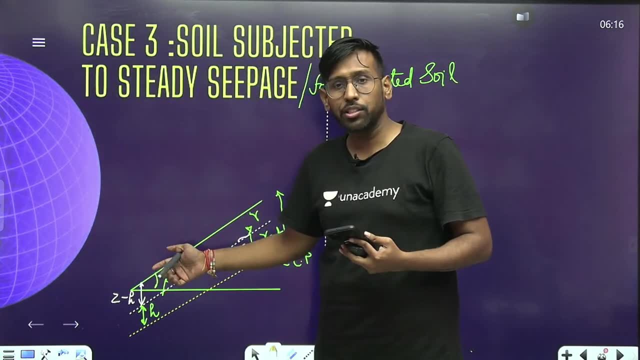 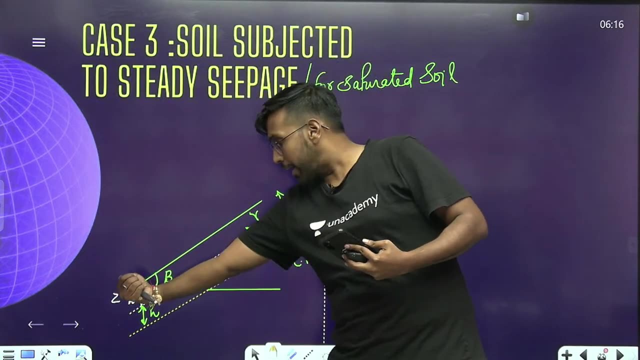 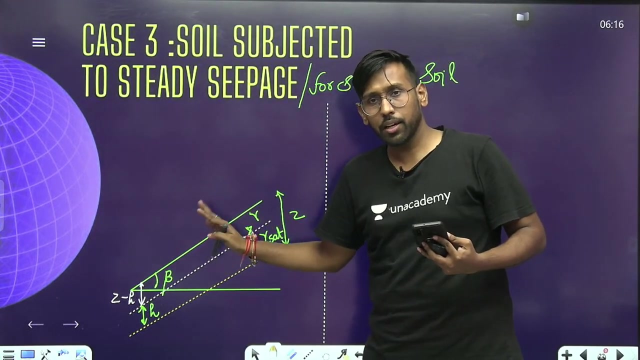 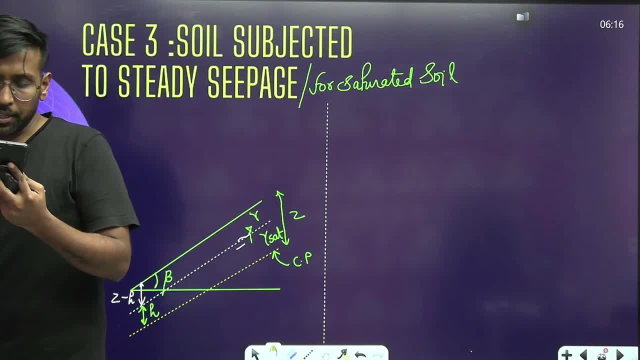 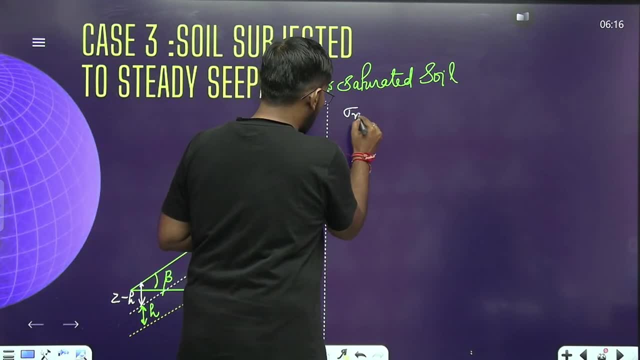 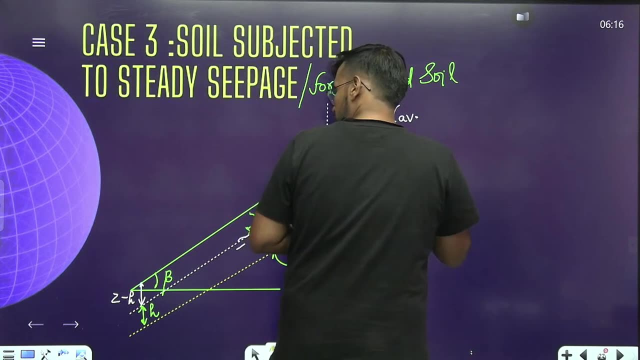 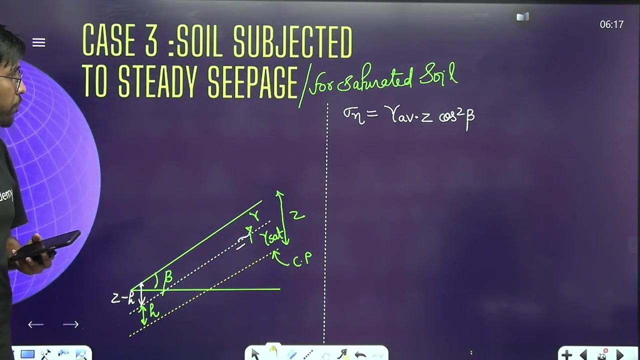 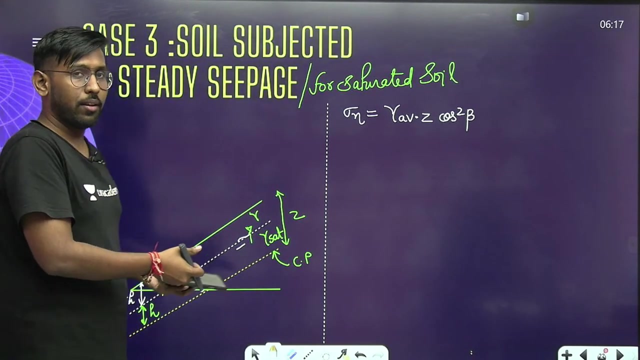 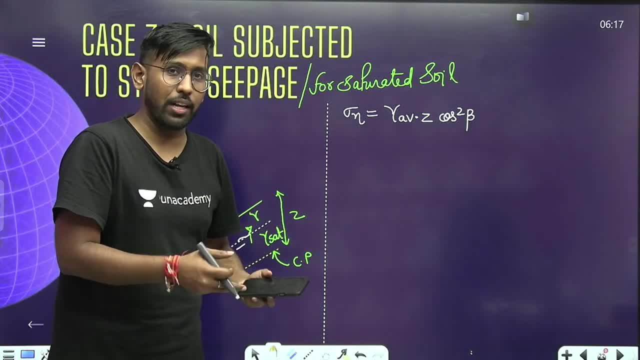 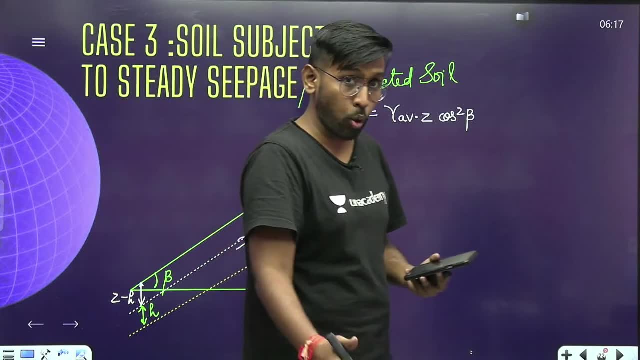 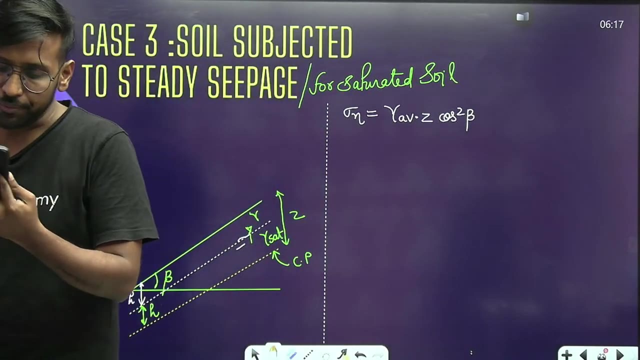 Now we are saying that we will take the total, We will not take the effective part, We are taking the weight component. That's why we are saying that we will do total stress analysis. If there was no flow, then we would have done effective. Ok, Yes, we are saying on failure plane. 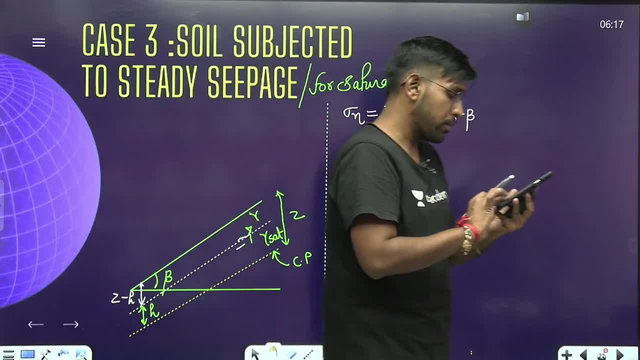 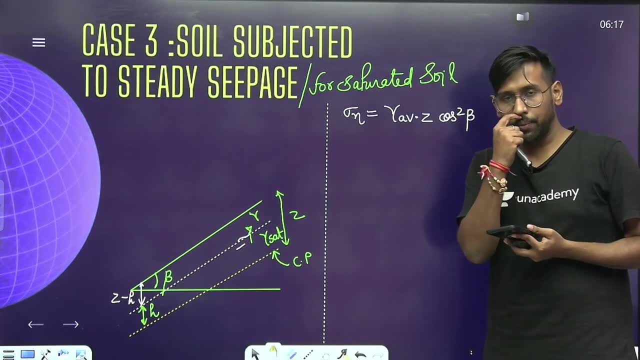 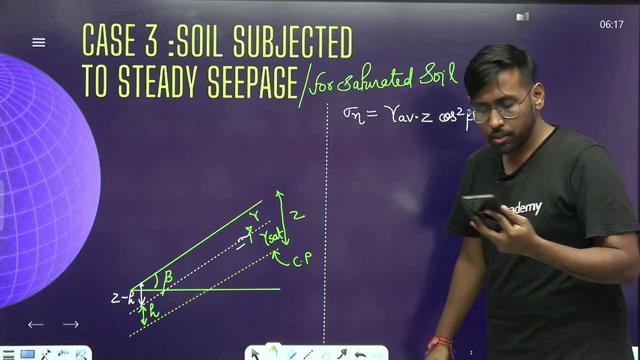 This is your critical plane, or failure plane, Which you are analyzing. Clear Naveen bhai is asking for old. My nature is like this. we teach like this. Ok, Now you will write useless things. Increase the light, Decrease this and that. First look at the screen. 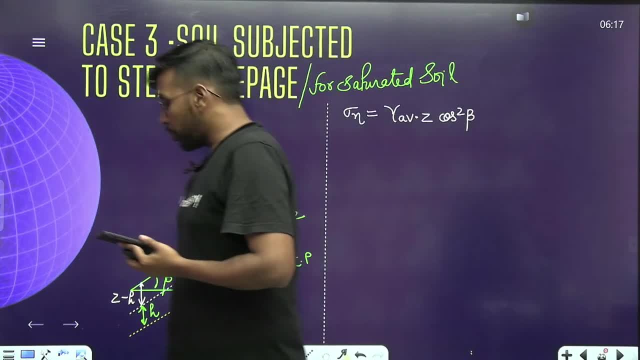 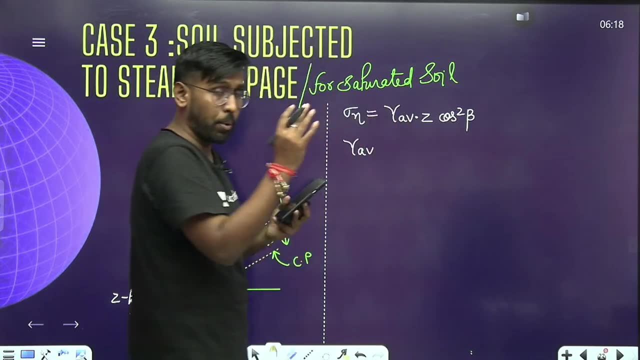 Ok, Let's see here, Come on, What will be written as gamma average. What will be gamma average, Gamma average- That is the total. We are talking about the total kit. We are talking about the total kit. So what will be written as gamma average, Gamma average. 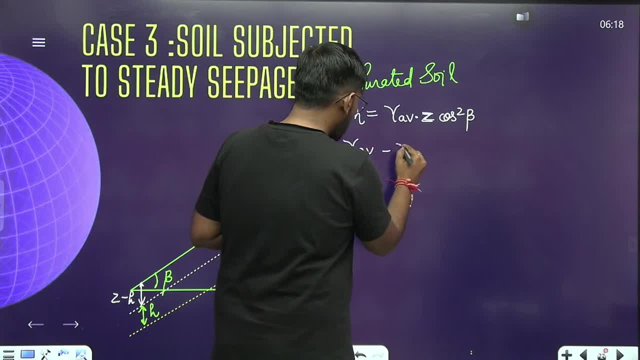 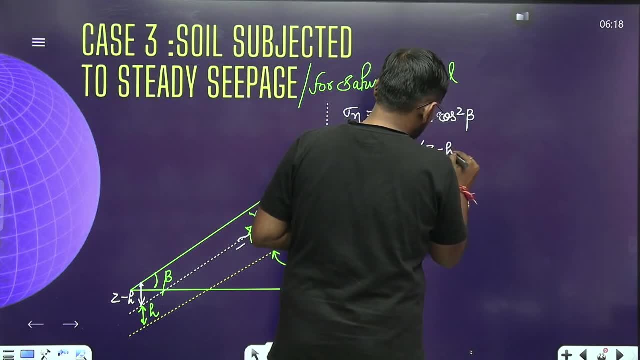 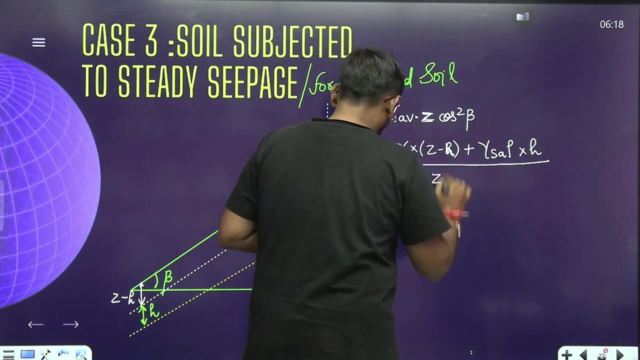 What will be written as gamma average Gamma into? How will you write normal average Gamma into Z minus H. Z minus H Plus Gamma sat Into H Whole divided by Z. Any doubt in this? Any doubt in this? This is how we write the average. 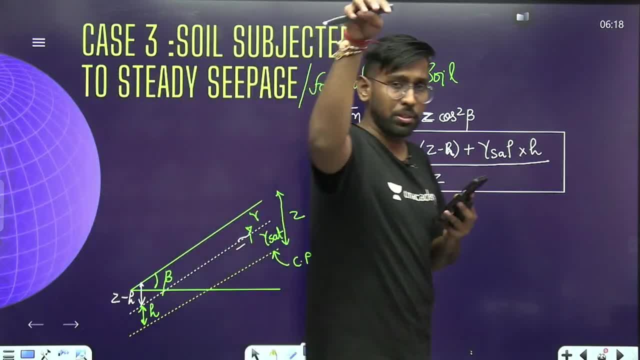 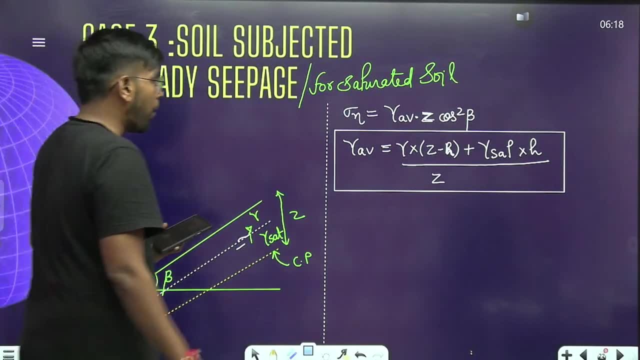 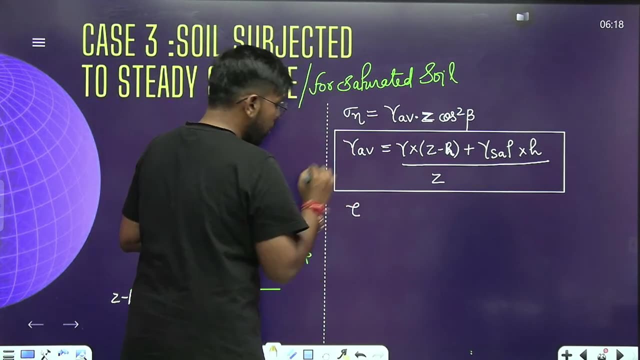 Because you are talking about the full depth Z. Now you have to tell the total stress for the full depth Z You are going to use the average, Ok, Gamma average- into Z cos square beta. That is your value of Sigma normal. What will be the shear? What will be the shear? 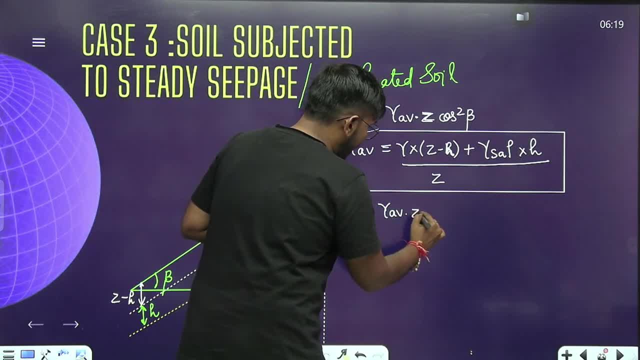 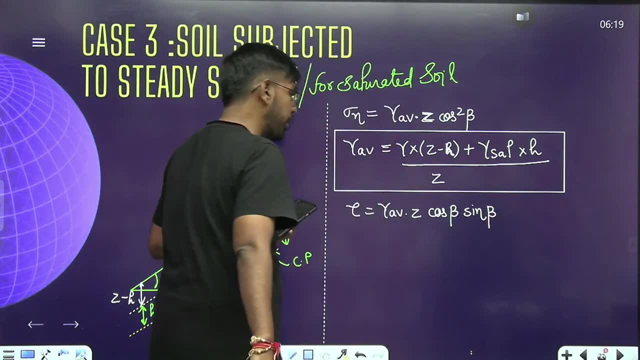 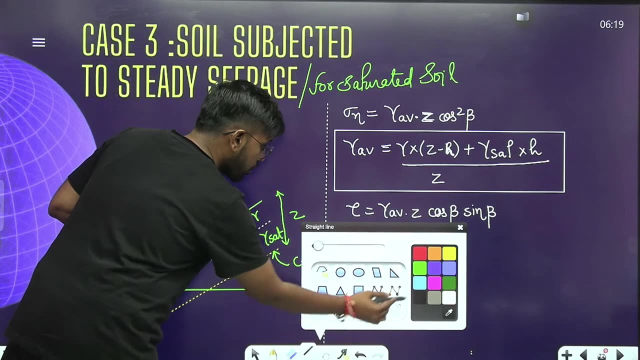 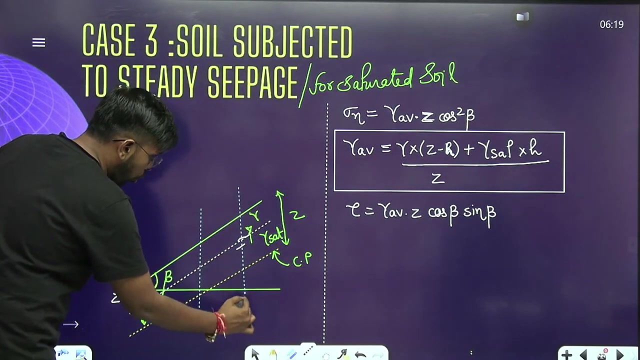 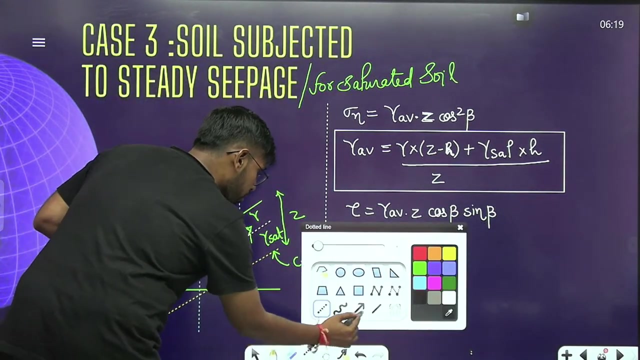 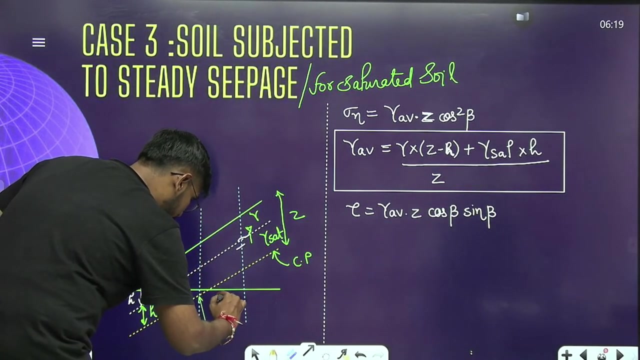 Gamma average Into Z, Into cos beta, Sin beta, Cos, beta, Sin beta. Ok, Clear Now, my friend, You will understand the thing carefully. Assume The analysis you have done, That you have done on width D. Ok, Now, my friend, here, Here You are told The pressure, which seems normal. 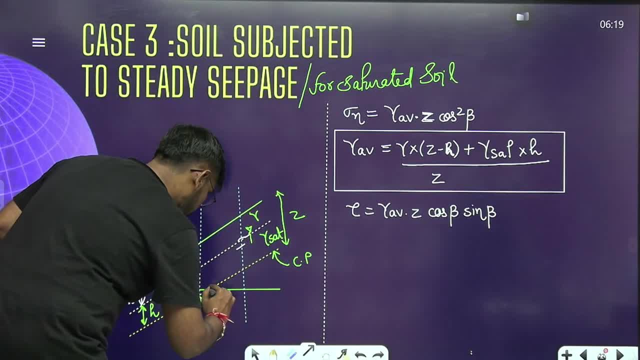 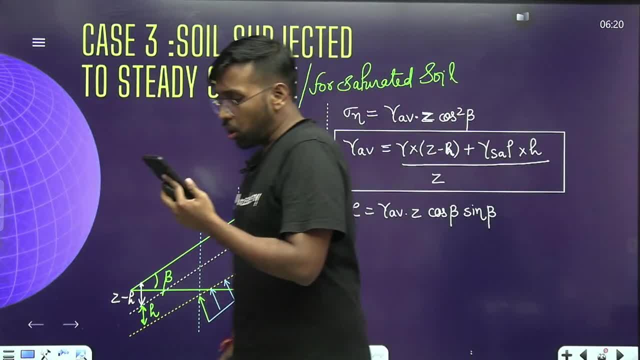 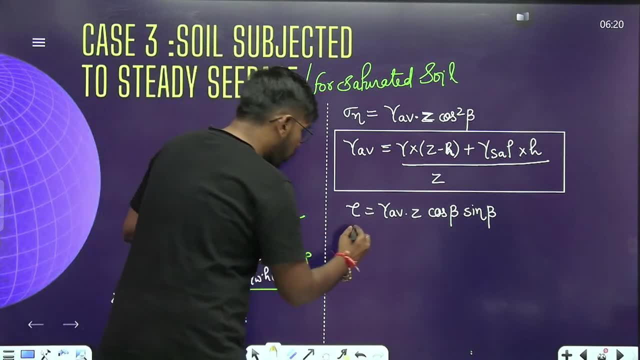 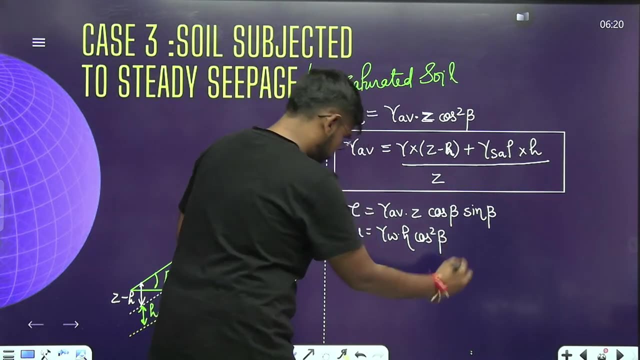 This pressure? This is Gamma W into H, Cos square beta. You write this, my friend, Yes or no? Pressure to the top, To the top: Gamma W into H, Cos square beta. How many people want to understand this thing, Sir? how did this come? 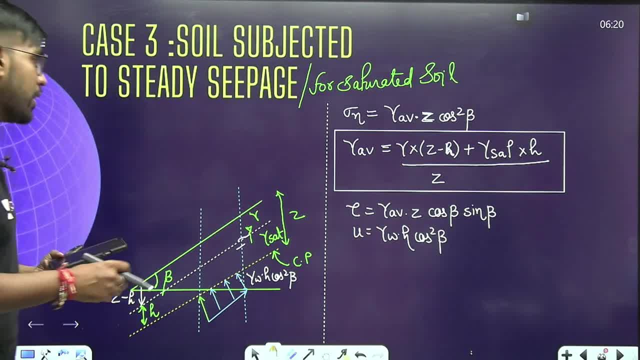 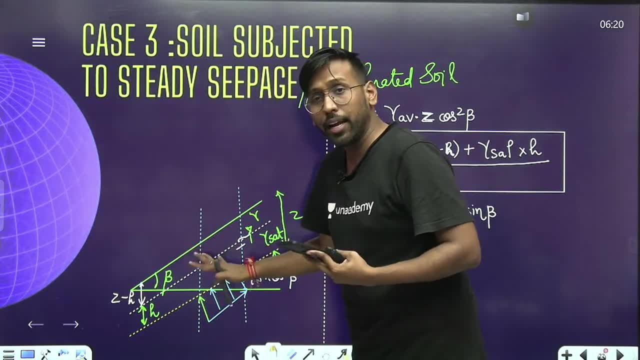 How many people want to understand this thing, Sir? how did this cos square beta come? How did you write Gamma W into H? cos square beta H is the height of the water table. The pressure seems. It's not Gamma W into H, But Gamma W into H cos square beta. 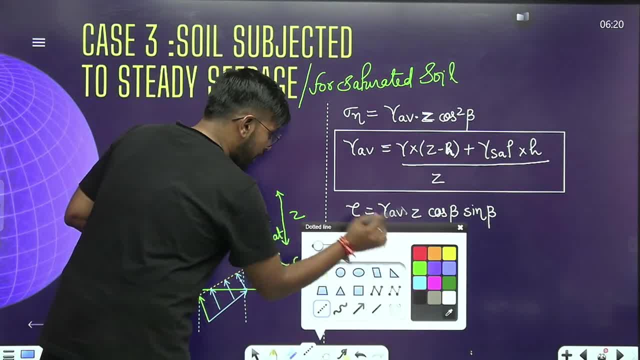 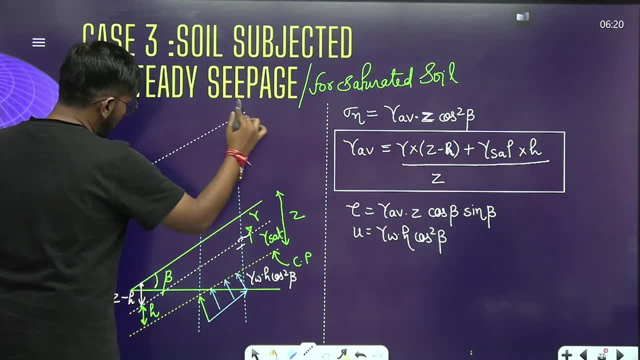 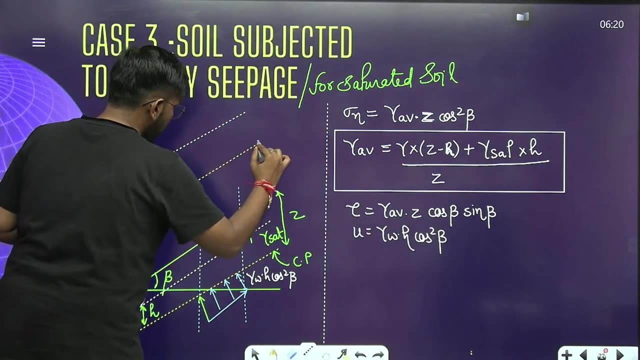 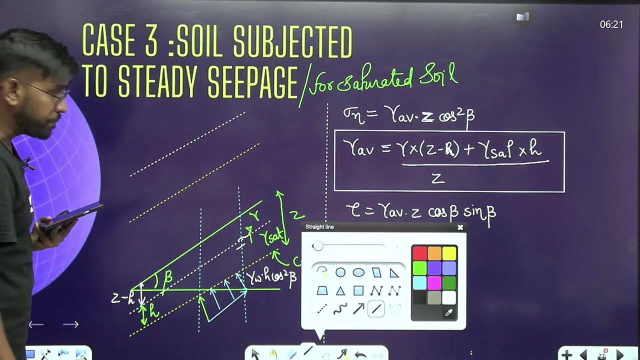 Ok, If you want to learn, Then you have to be patient. If you want to learn, Then you have to be patient. Yes or no? If you want to learn, You need to be patient, You don't have to be impatient. See here, See here, My friends, What is this height? 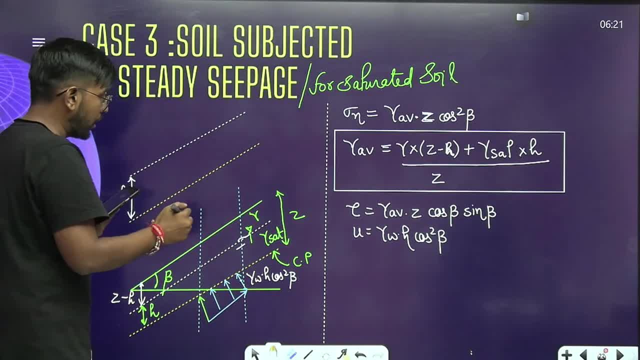 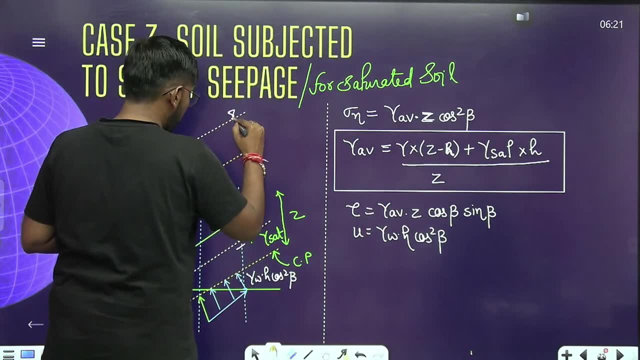 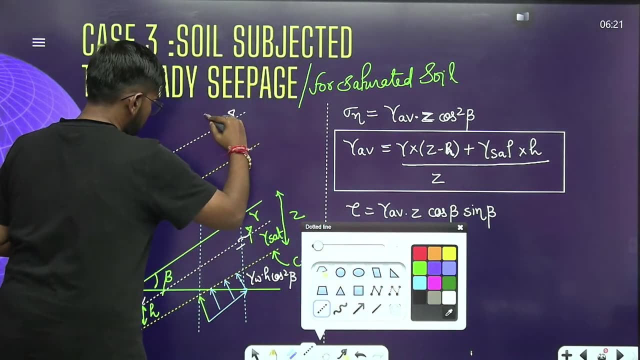 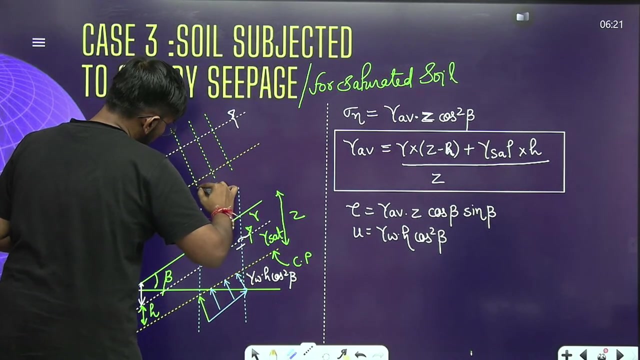 This height is H- Vertical- Vertical. you can see. Ok, Now, my friends, This is your water table. This is your water table. Now, my friends, If I make a flow net, If I draw the flow net, So this is your equipotential line- It will be perpendicular to the flow line. 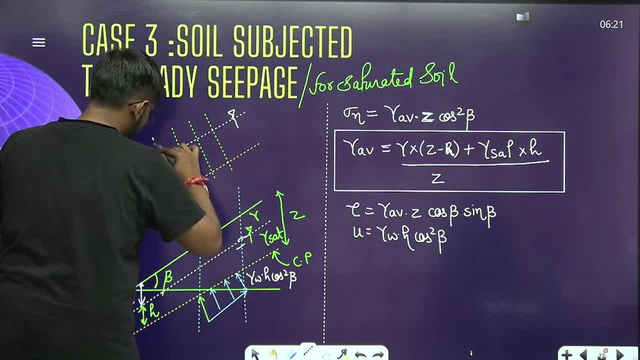 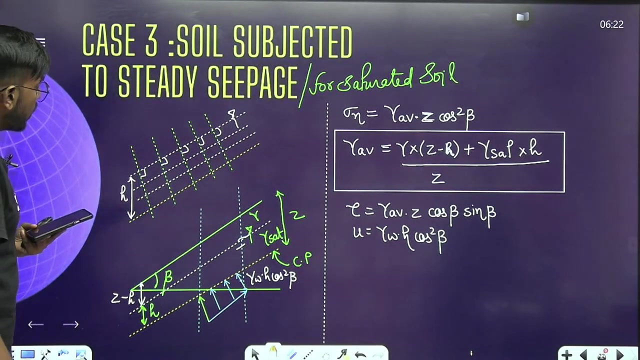 Which is your equipotential line? Which is your equipotential line? It will be perpendicular to the flow line, Yes or no? These are the flow lines. These are the flow lines. Ok, Right, So what is the white one? What is the white one? 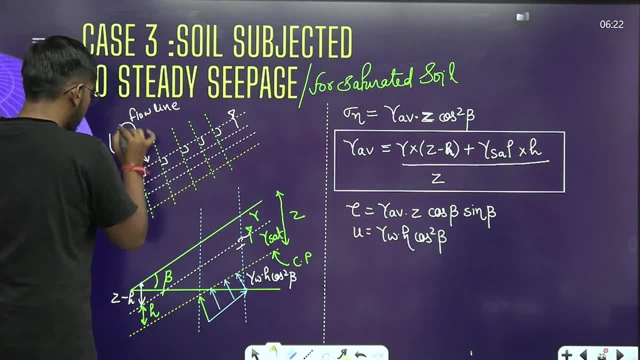 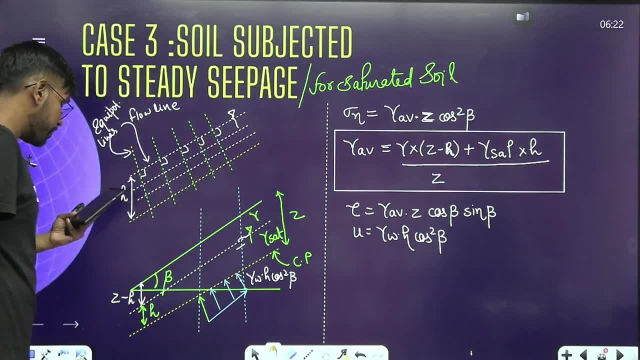 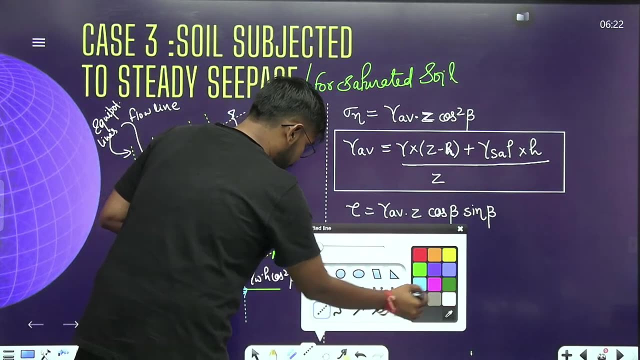 These are flow lines. And what is the green one? These are equipotential lines, Equipotential lines. Ok, till here, Players, till here. Now you will understand the thing carefully, My friends. If we put a piezometer On this bottom, If we put a piezometer, 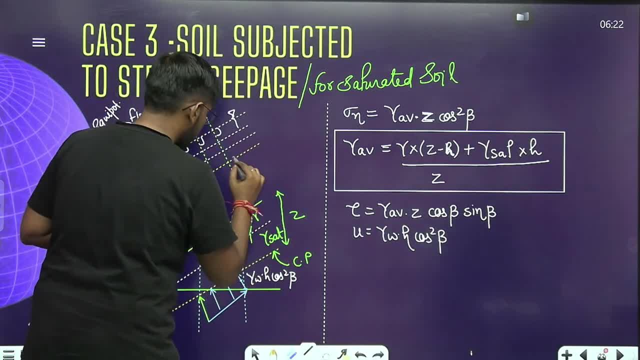 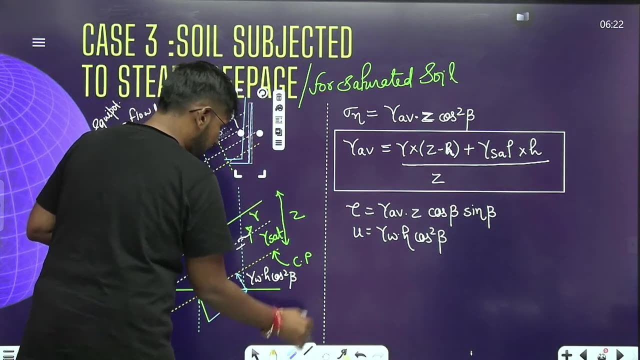 On this bottom. It will be fun. It will be fun On this bottom. If we put a piezometer On this bottom, Then how much water level will rise? How much water level will rise? How much water level will rise If we put a piezometer? 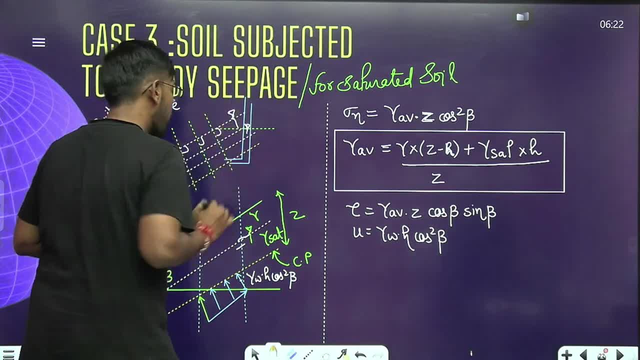 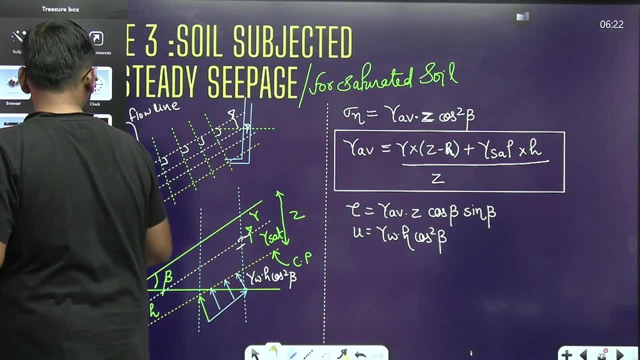 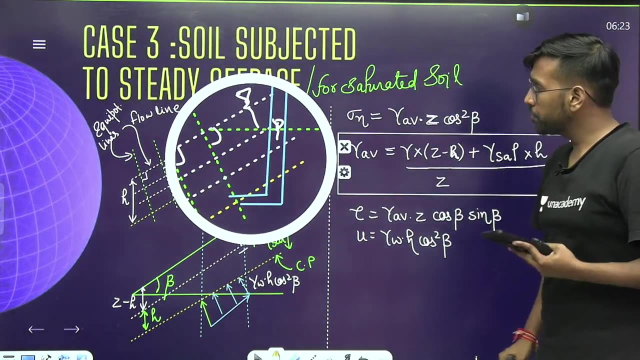 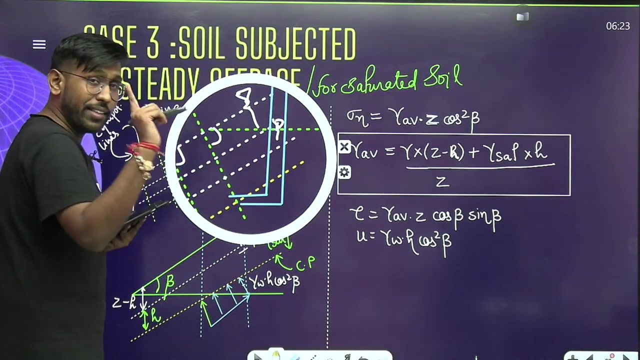 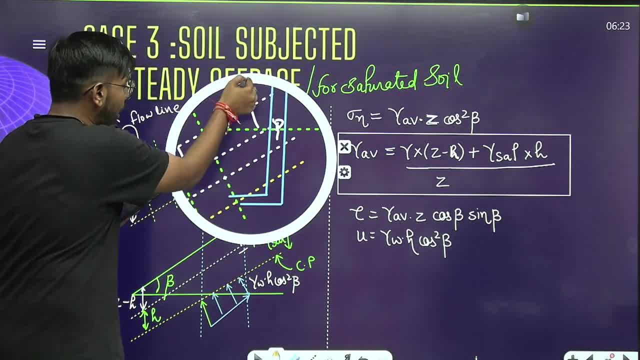 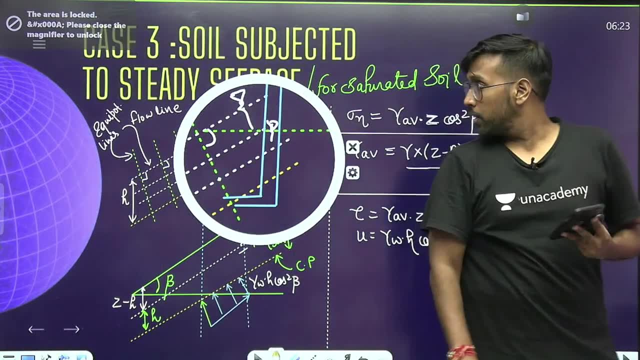 Where did the H-height go? This was the H-height. This was the H-height. It didn't rise till the H-height. How much did it rise? It was less than that. Did you understand this? Did you understand this? It is not rising. Look here. 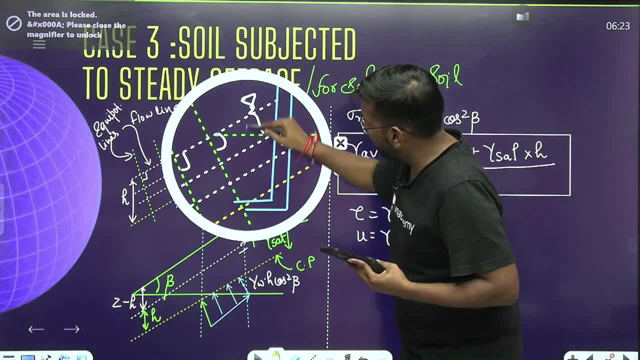 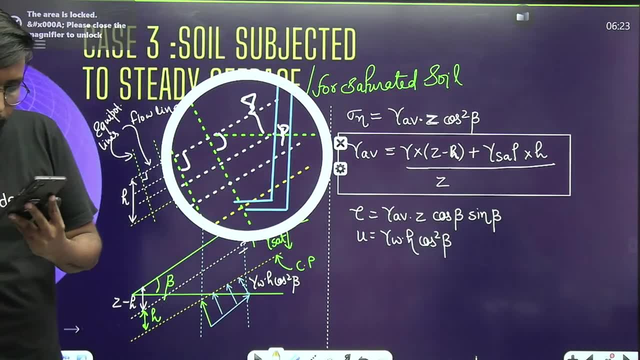 How much is the H-height From here to here? If this was the full rise, Then only it would be H-height. There is no H-height here. It is less than H-height. It is less than H-height. Did you get the feeling? Did you get the feeling from inside? 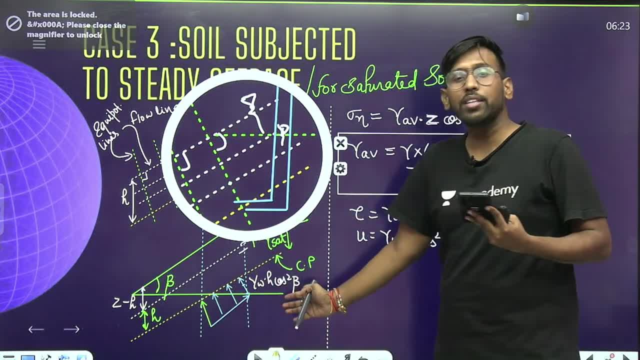 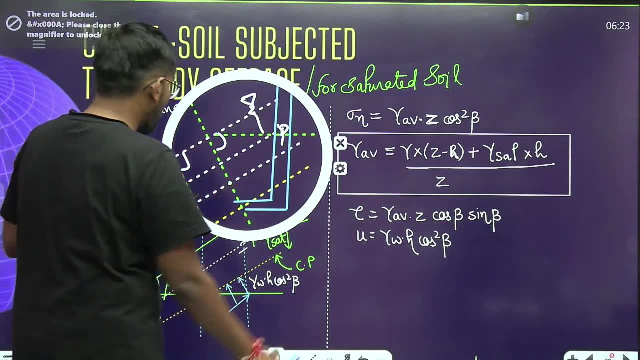 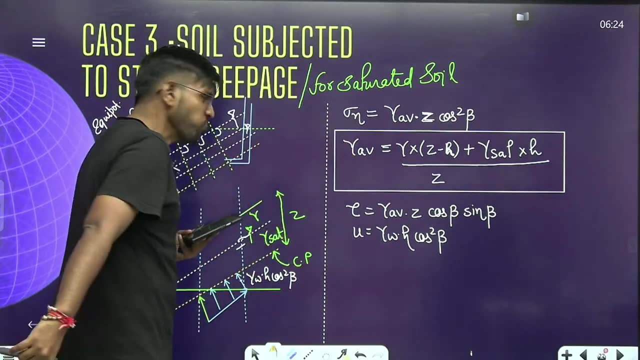 If the H-height had risen, Then it would have been Gamma W into H, It would not have been cos square. beta, Yes, Then it would have been Gamma W into H, It would not have been H-square. Come on Now you will see My friends. So this height. 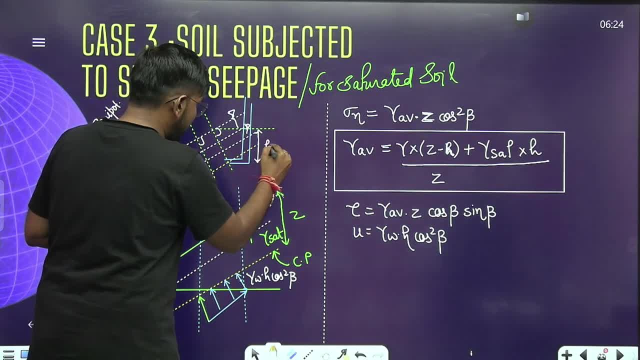 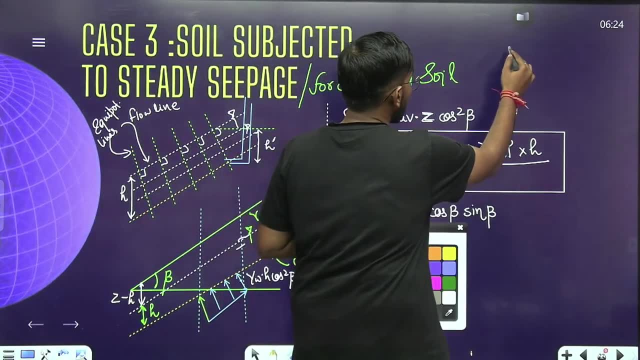 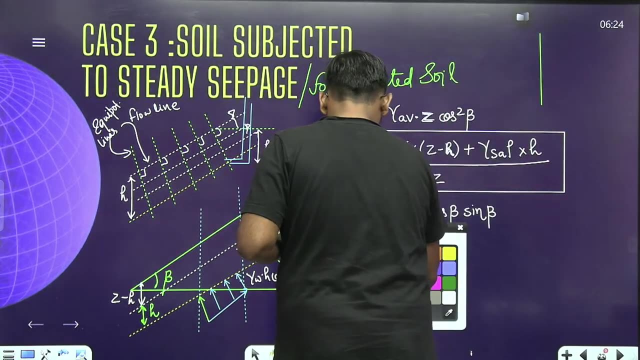 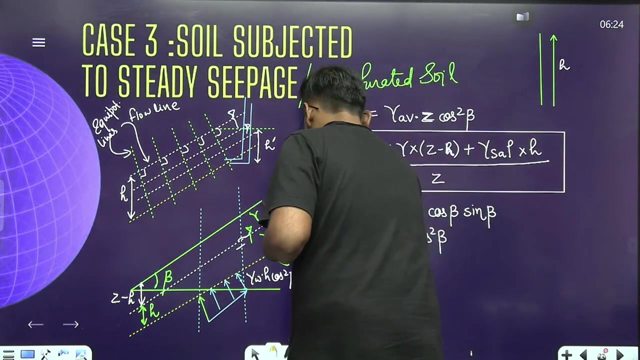 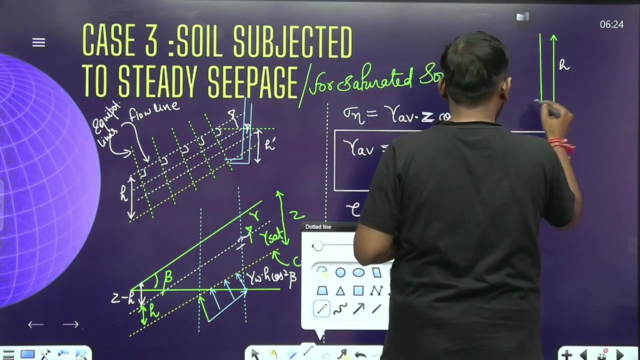 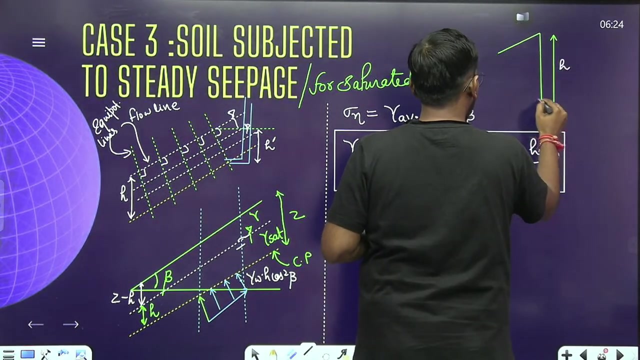 We are saying that This height is Some H- Let's have fun. So, my friends, This is the height of your H, Complete, Okay, You Who asked? He asked: Look here, Do you see a triangle here? Do you see a triangle here? Look here, Do you see a triangle here? 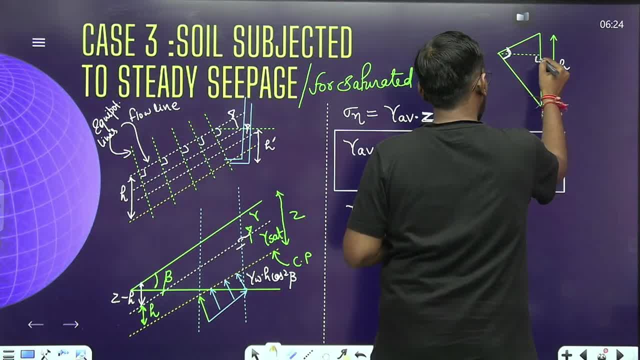 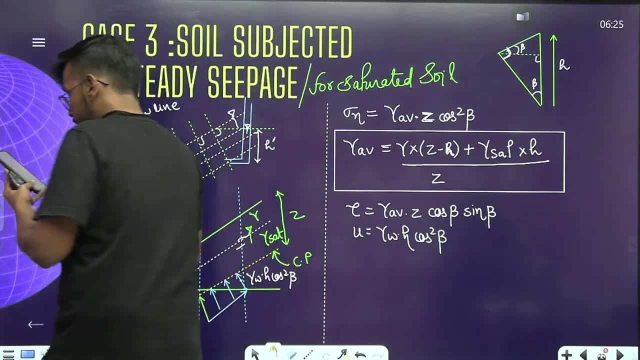 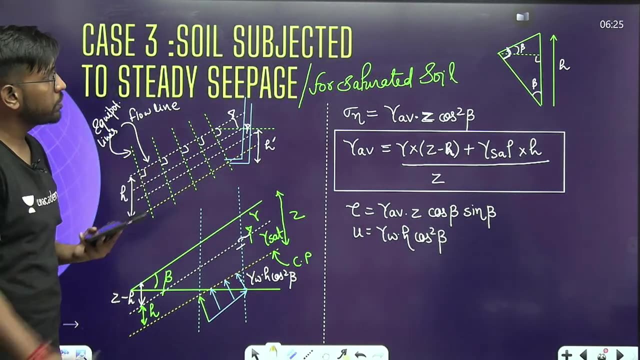 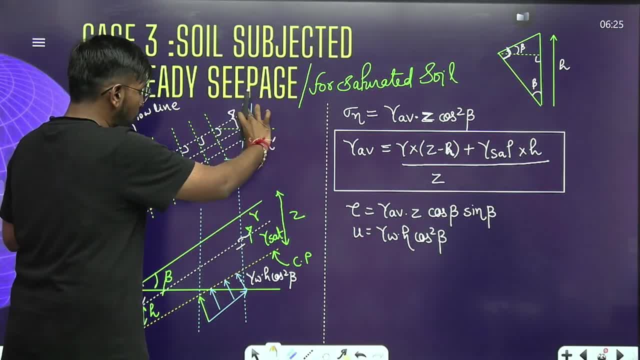 If this is complete, What is the height Means this H dash? If this is complete, H, What is this angle yours? This angle is your beta. If you should form a triangle here, If you should form a triangle here, Then what will the triangle tell you? 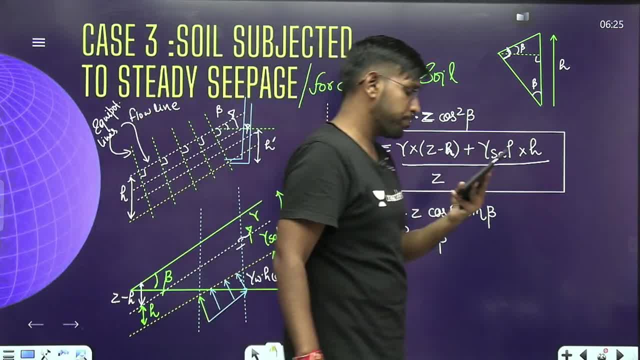 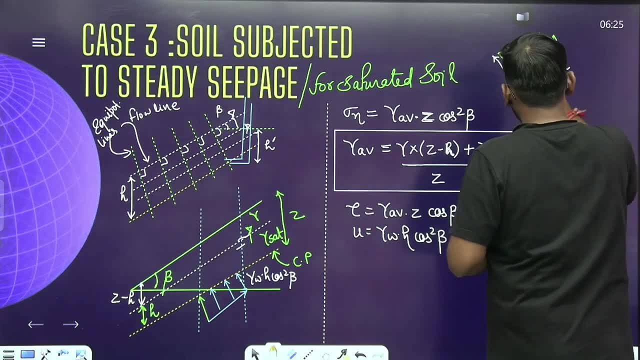 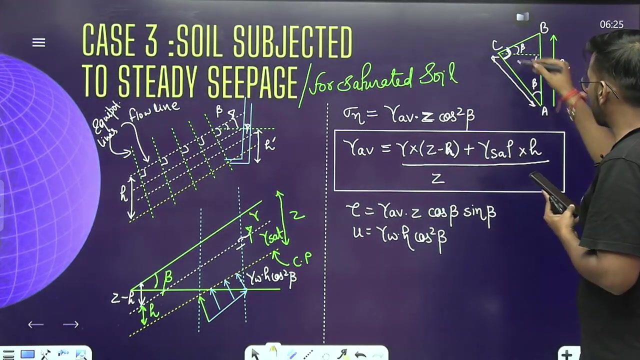 The triangle will tell you That this height is your Capital: H. Right Now, my friend, If this is H, what is this site? My friends, look at the big triangle. ABC. This is perpendicular means, it is hypotenuse. So what will be? AC? 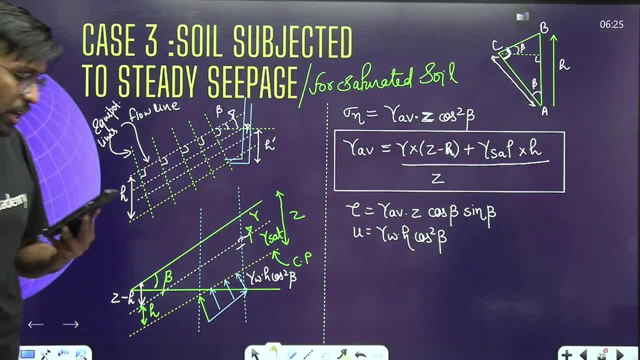 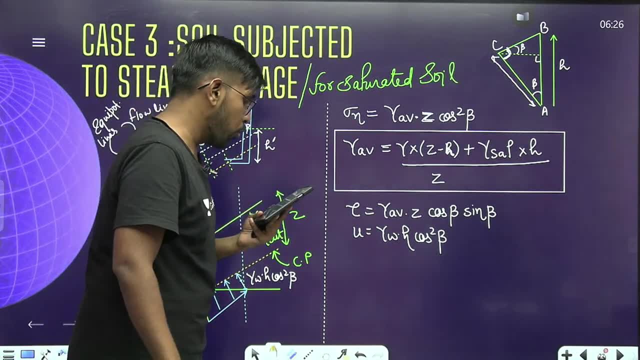 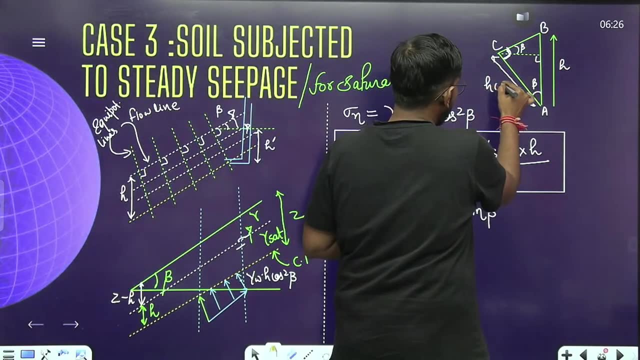 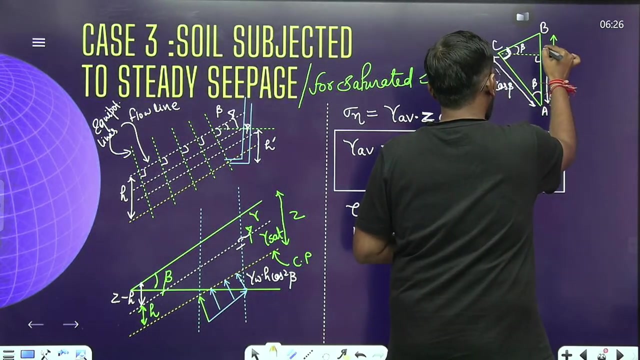 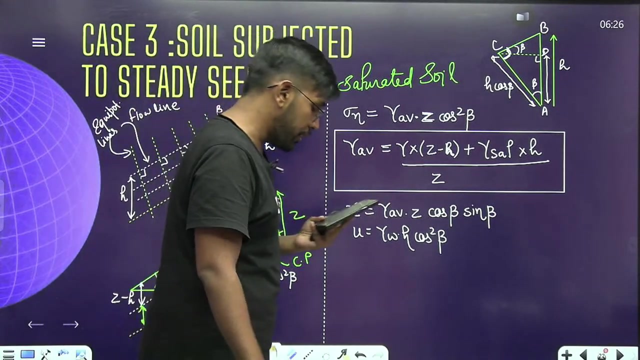 What will be AC? Tell me, my friends, what will be the value of AC? H cos beta? This value is H cos beta. So if this is H cos beta, then what will be this Now? look at the triangle ADC. Look at the triangle ADC. 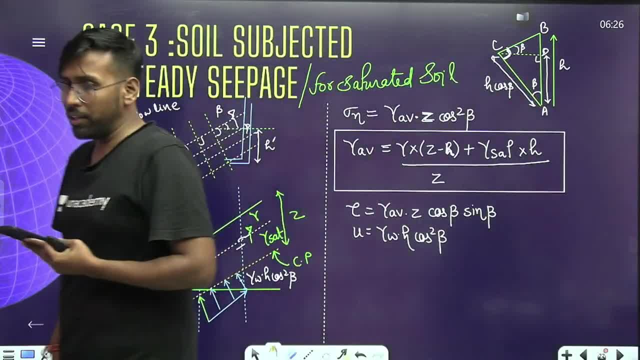 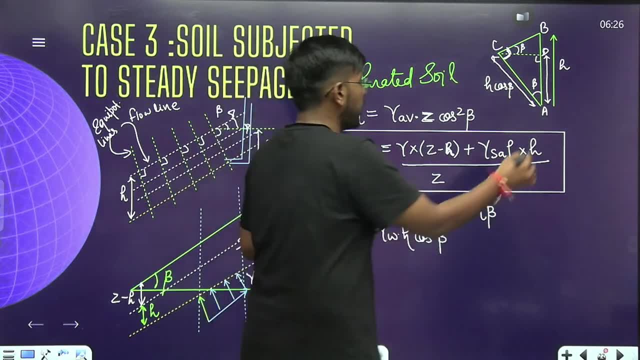 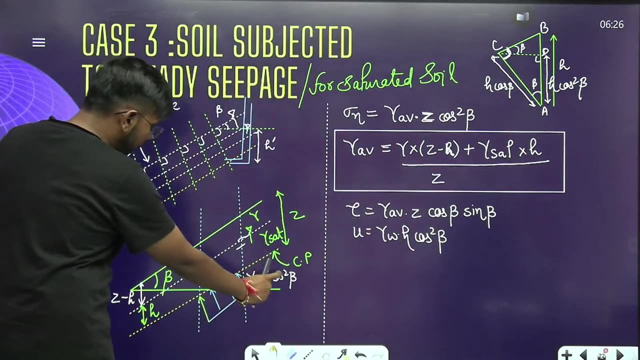 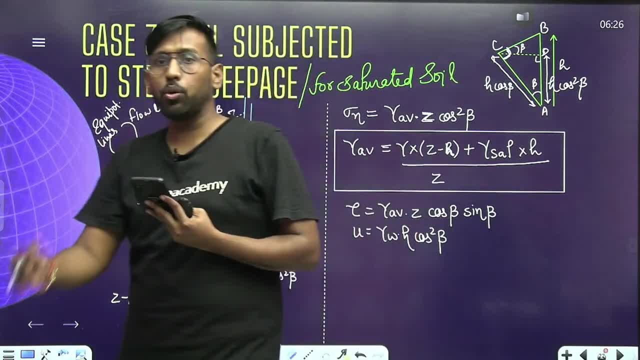 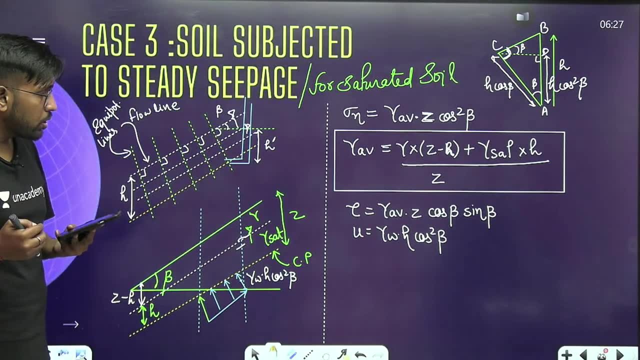 That is why I am showing you the pressure job above. That is gamma W into H cos square beta. Did you enjoy? Did you enjoy? Did you enjoy? Yes, So why is U gamma W into H cos square beta? It should be clear. 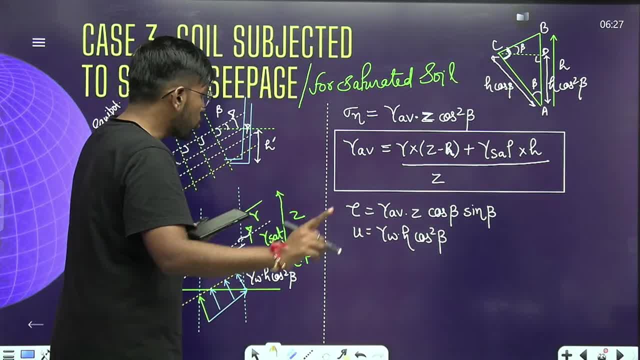 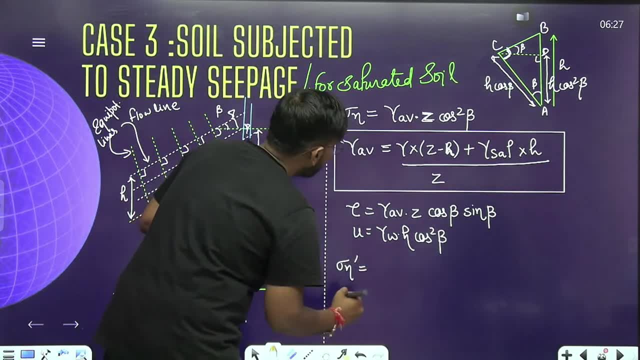 It should be clear, Okay. So now, my friends, when you are talking about normal, you will talk about effective. What is effective, Yes, what is effective? Gamma average into Z cos square beta, minus gamma W into H cos square beta. 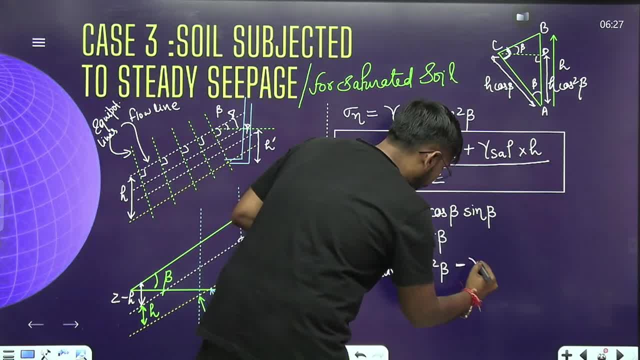 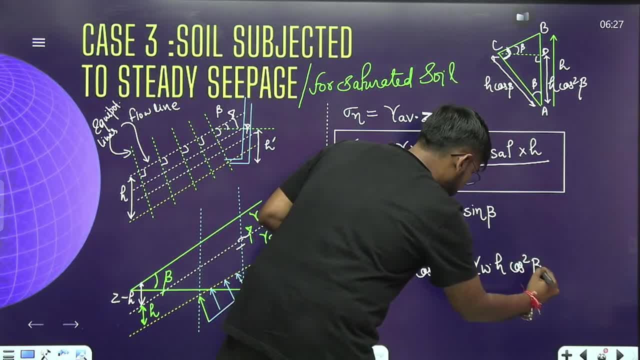 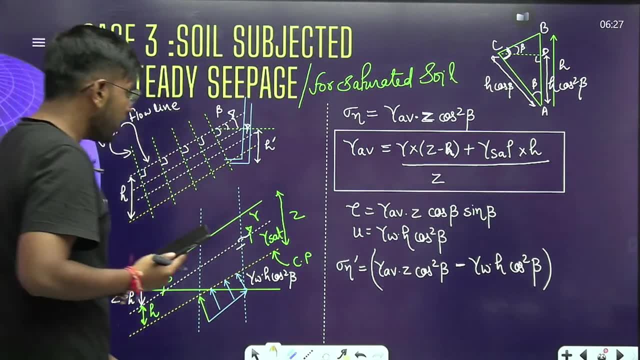 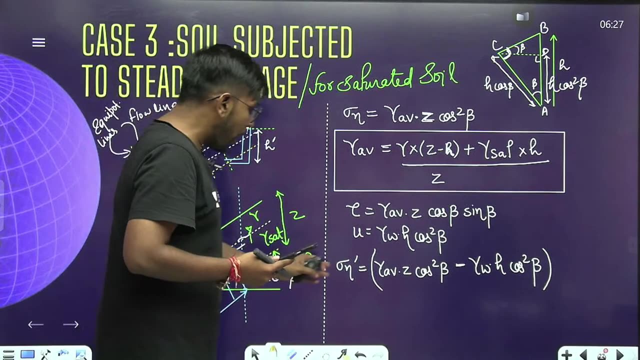 Gamma average into Z cos square beta minus gamma W into H cos square beta. Gamma average into Z cos square beta minus gamma W into H cos square beta: Now this is your effective normal stress. This is the effective normal stress. Is it clear? 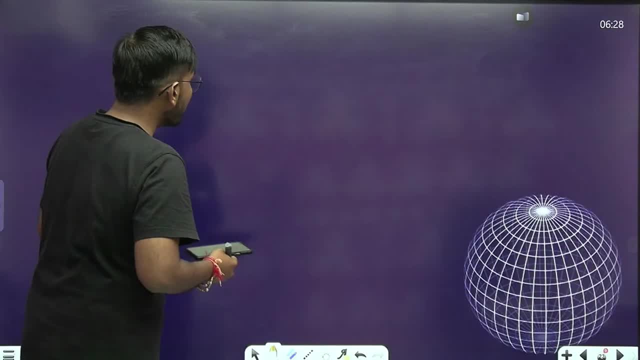 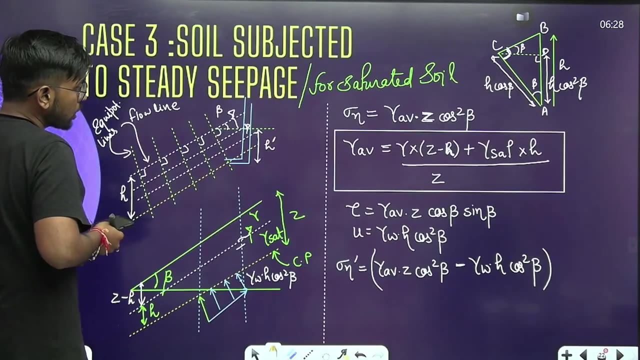 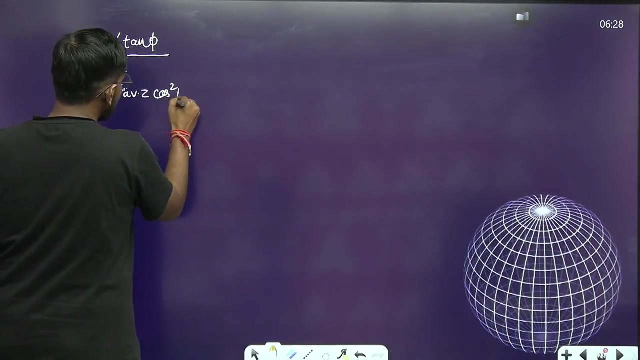 Is it clear. So this is your sigma and dash. Now, my friends, if I talk about shear, Gamma Index Arg, If we talk about shear, then we will write sigma n dash, tan phi and phi dash are almost same upon tau. so what is sigma n dash? gamma average into z cos, square beta minus gamma. 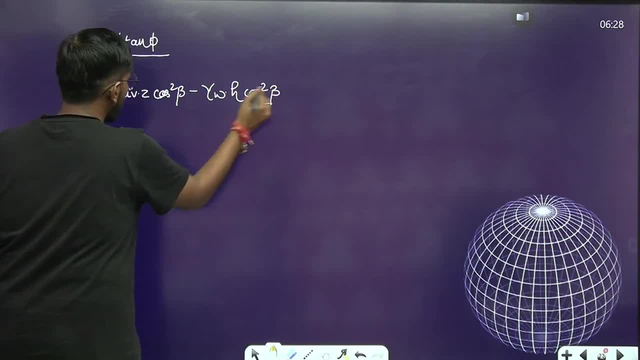 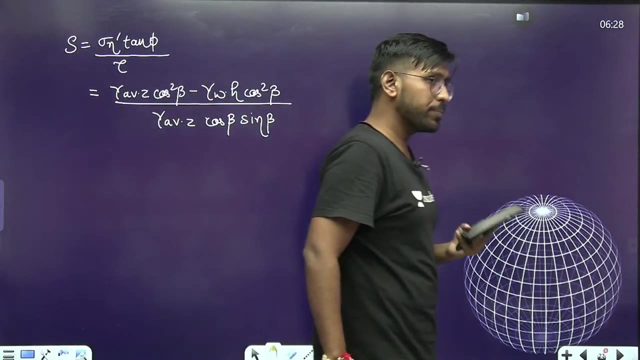 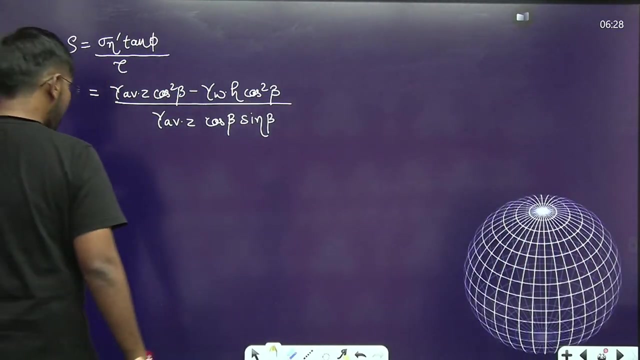 w into h cos square beta whole divided by gamma average into z cos beta, sin beta. here you will not have subtraction, is it clear? so this is the shear strength. this is the shear strength. is it clear? till here, say kids? will you tell till here any doubt? so this: 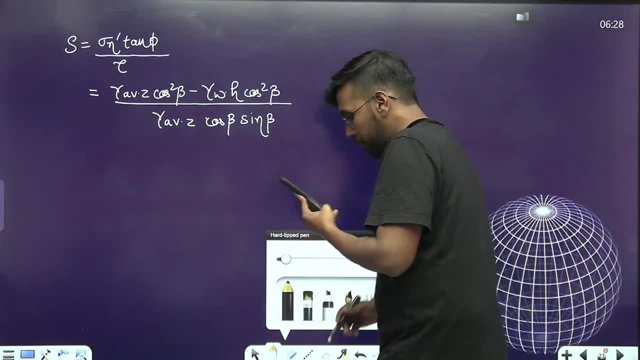 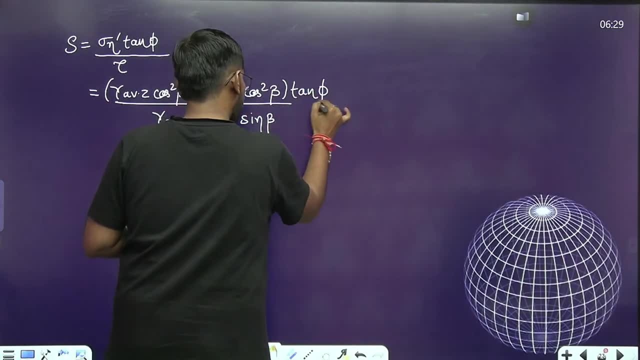 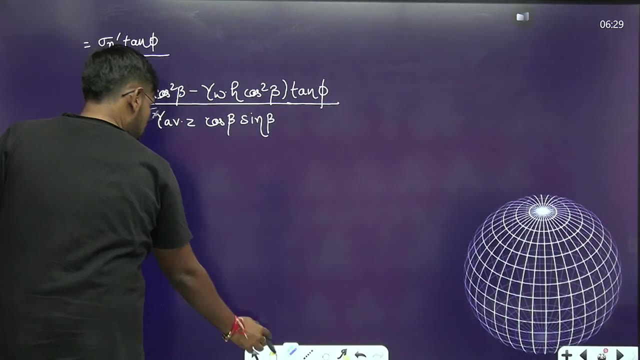 point is clear. This formula is very useful to you. many times directly question is asked in objective: this multiplied with tan phi. this multiplied with tan phi. this directly question is asked in exam. ok, ok, we will write shear, stop, stop, stop. we will write it right. factor of safety. 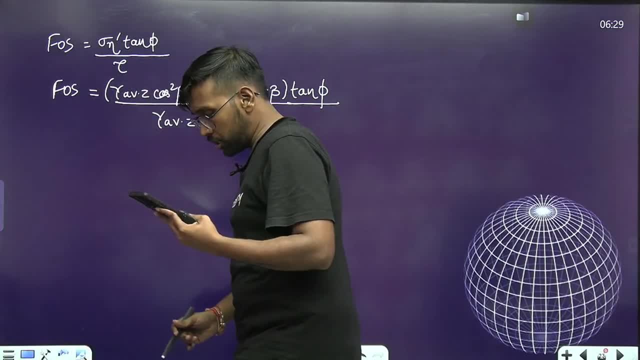 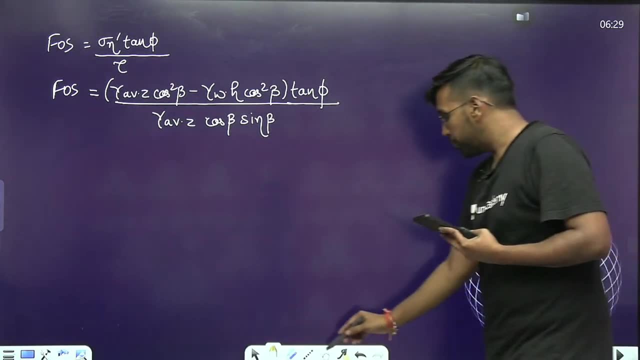 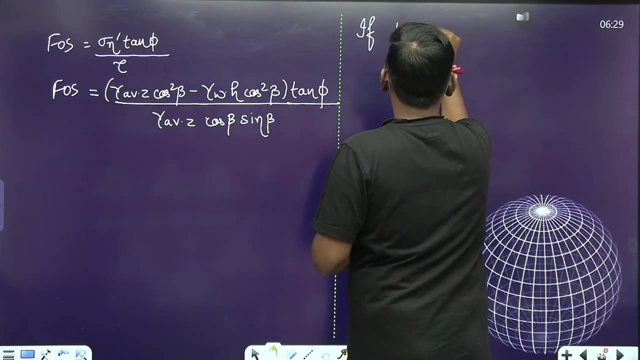 factor of just a minute. yes, is it clear? is it clear? say my friend. so this formula is is clear, This formula of factor of safety is clear. Now, my friends, if water table reaches the ground surface, If water table reaches ground surface Tomorrow, I will do numerical. 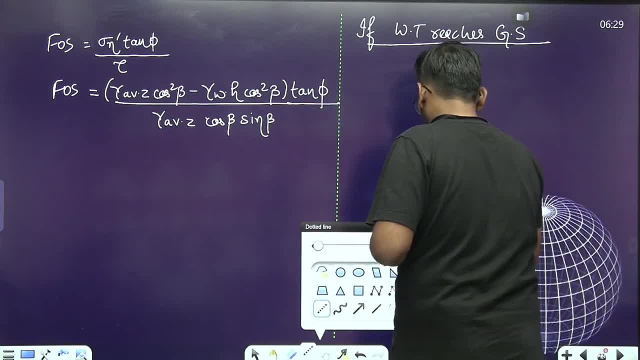 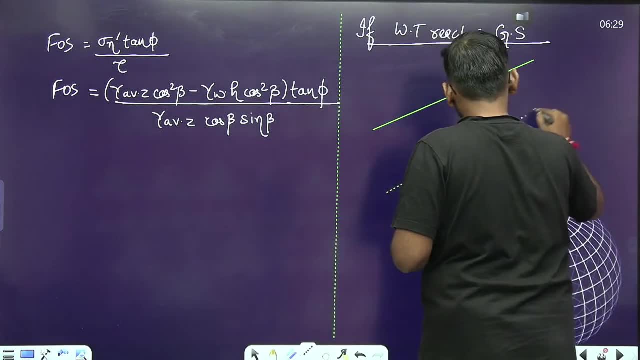 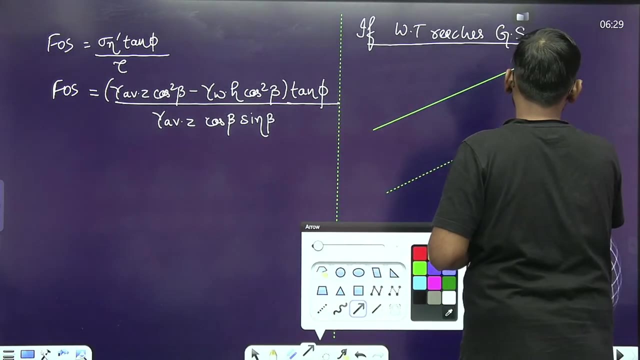 on this. Tomorrow I will do numerical on this. See here. So, if water table reaches the ground surface, This is your ground surface Right and this is the failure plane. Yes, This is the failure plane. So, my friends, This is Z equal to H. The water table is reaching. 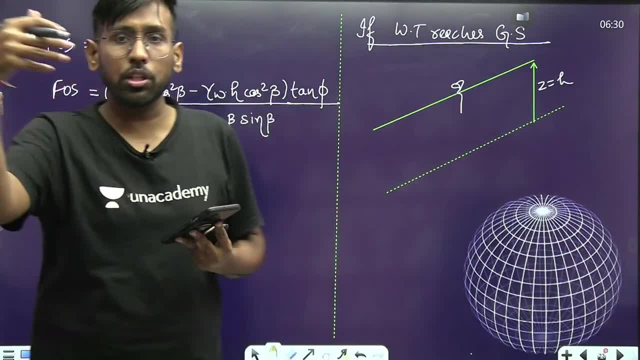 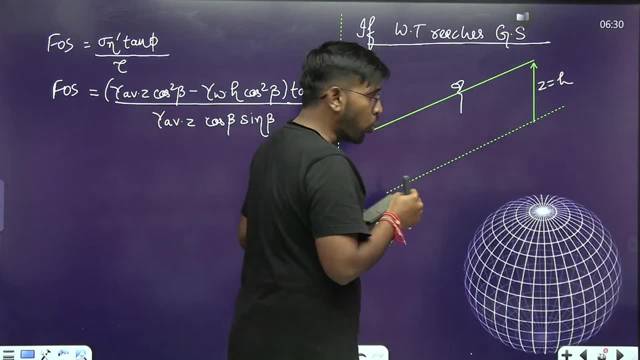 the ground surface. So, yes, there will be seepage, The flow will be there, The flow will be there now, If the flow is there, my dear friend, If the flow is happening, If the flow is happening, So you will understand here, If there is a flow, So now what will happen here? Now what? 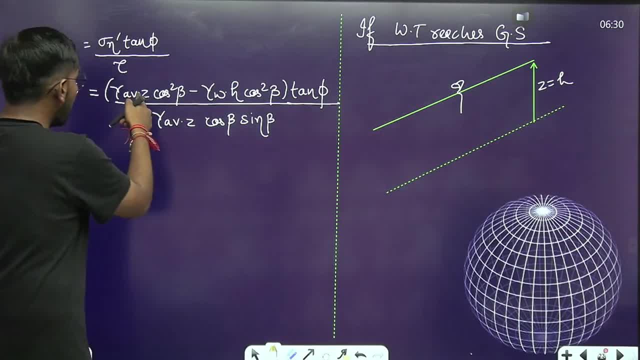 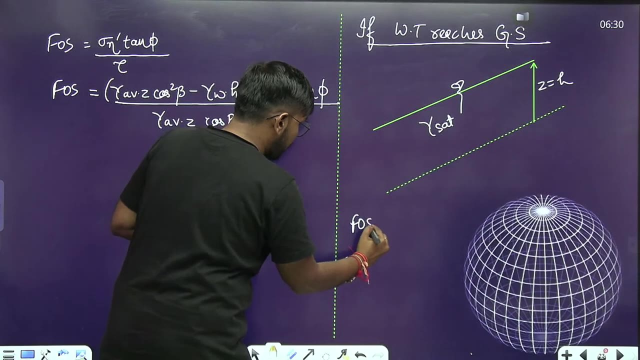 will happen here. If Z equal to H happens. If Z equal to H happens, Then the water table reaches the ground surface. This will happen. It becomes a square. But here, in this situation, z equal to H happens Because water table is at ground surface. So the water table 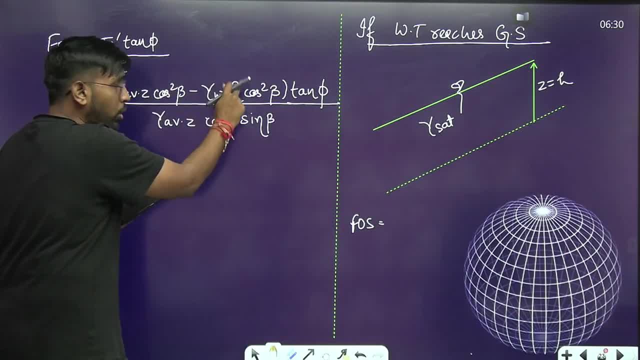 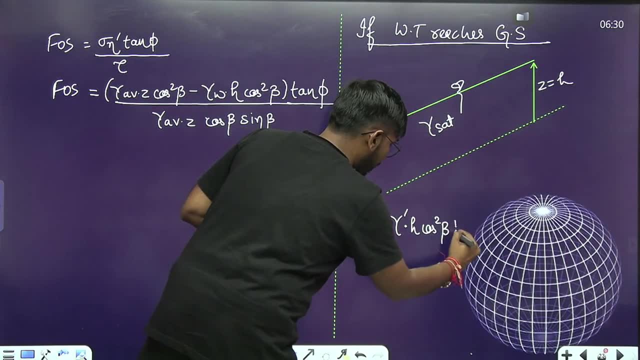 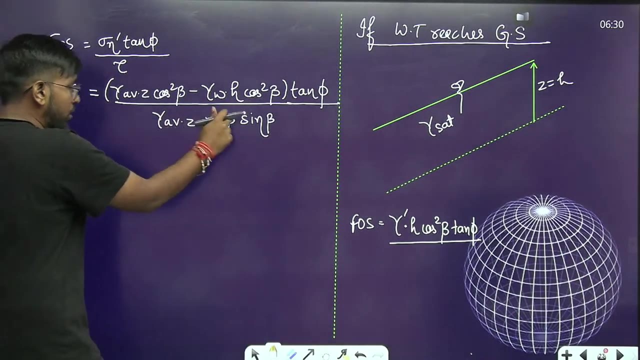 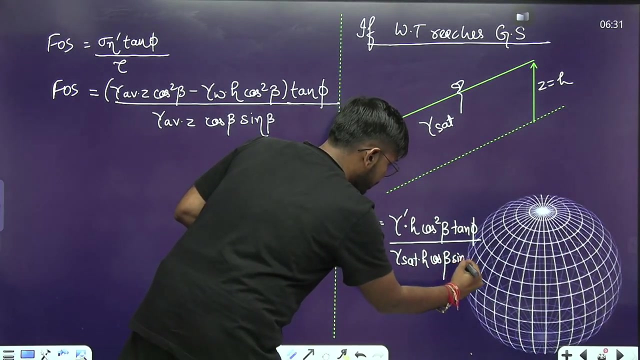 is falling on this. You'll notice that This is very strange figure. today. Usually we tell z is in ground surface, but in anyииi you can't. Yeah, Gamma sat into h: cos, beta, sin, beta, cos, beta, sin, beta okay. 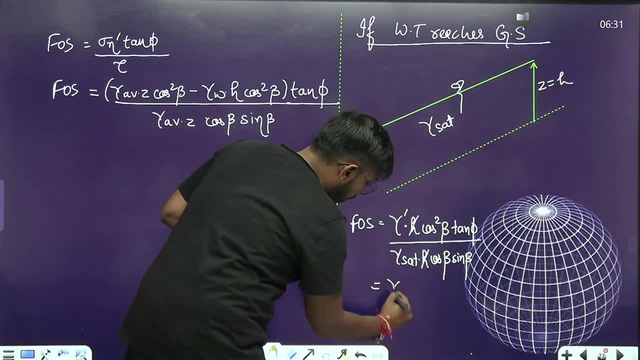 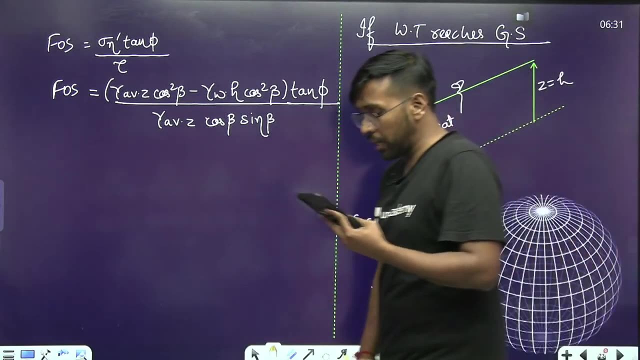 So now my friends h h is gone. What is the formula? you have Gamma submerged by gamma, sat into tan phi by tan beta. Any doubt in this, please ask. I don't have any session recorded, son, I do everything live. 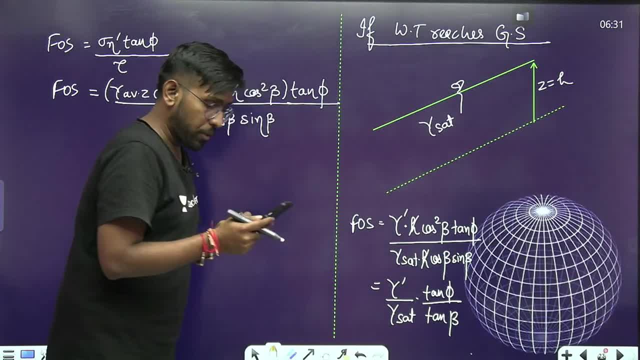 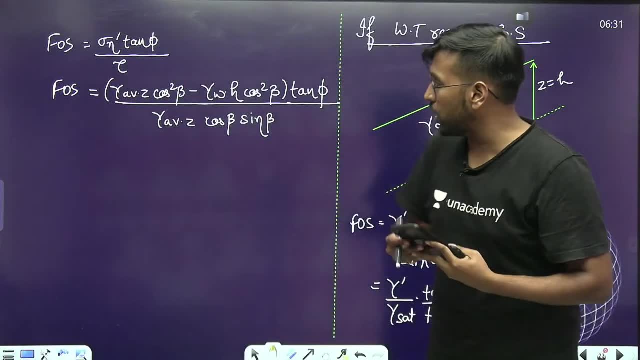 Even the 10-minute session is also live. Come on, Did you enjoy? Did you enjoy? Will you tell everyone quickly? Is this point clear? So, when the water table reaches the ground surface, how does this formula come? You should also understand this. 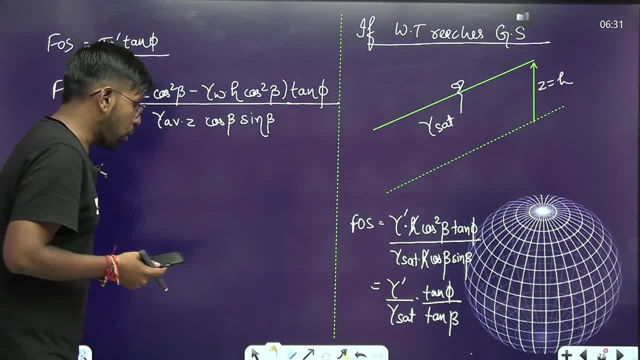 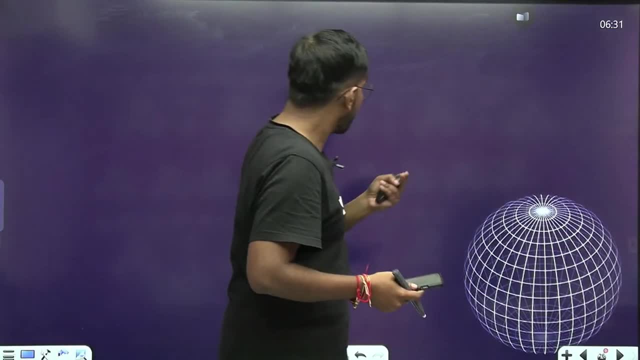 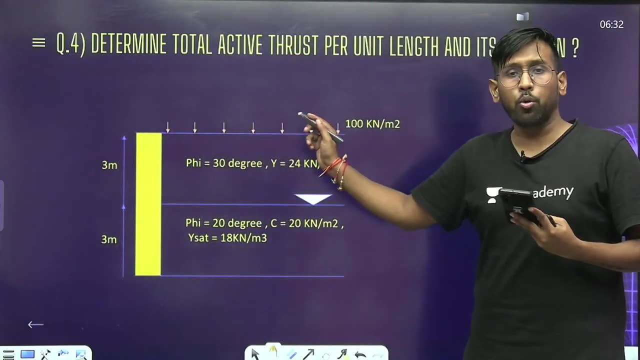 Yes, Yes, Come on. So, my friends, till now you were here. Tomorrow we will tell you more points. We will discuss numerical. Okay, Tomorrow we will discuss more things. I hope you have written this numerical. So tomorrow you have a special session on sheet piles. 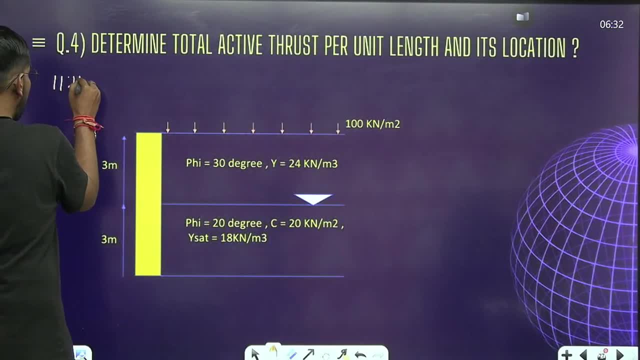 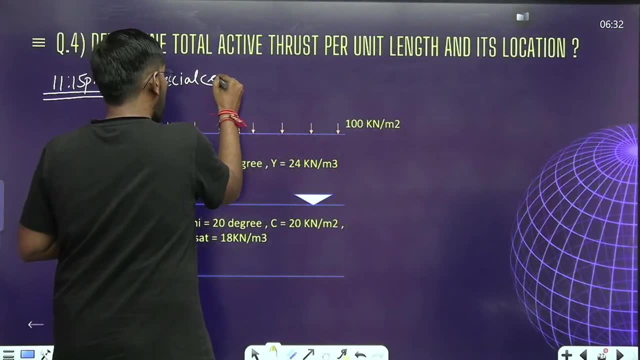 Tomorrow at 11.15pm. At 11.15pm there is a special session on sheet piles. Special session on sheet piles. So there only I will also do this numerical. Okay, I will also do its solution there also. So special session on sheet piles. 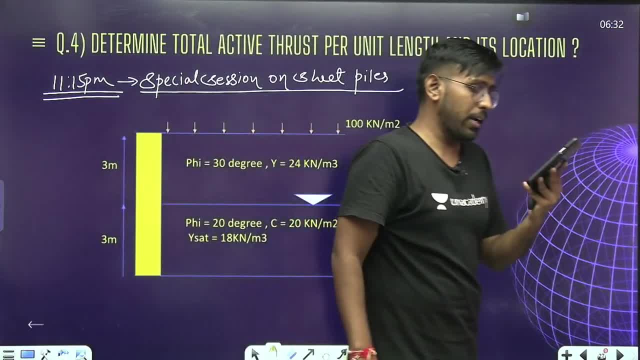 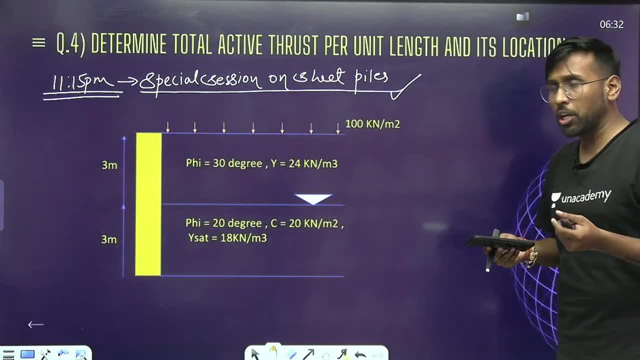 We will be doing a special session on sheet piles tomorrow. we will do it on this only tomorrow, Is it clear? It will be on YouTube only, not on special. it will be on the YouTube Because sheet piles were remaining, so we put a special session. 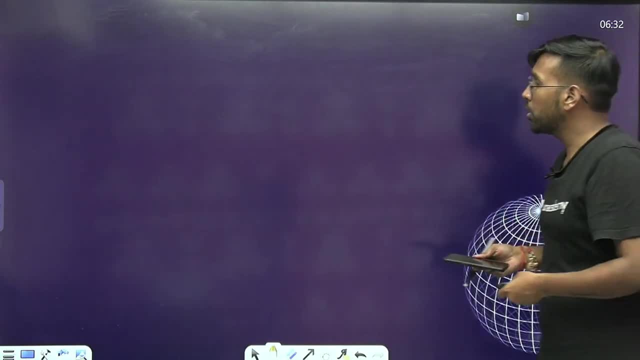 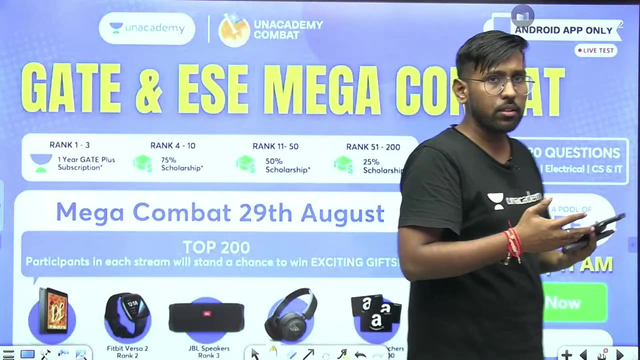 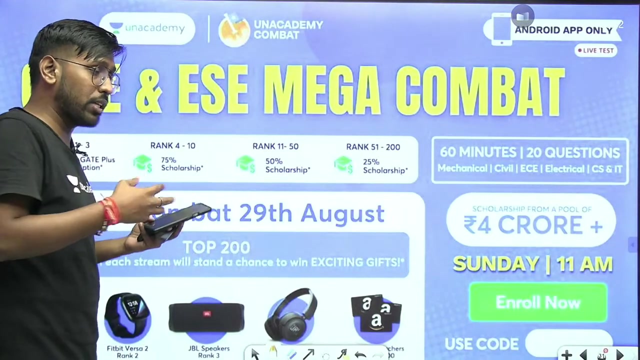 When we will do it, then why do we need an answer? Rest your combat, my friend. the combat is scheduled on 29th- 29th, I think, yes, 29th- Where there is a mega combat in which you can win a scholarship, you can win like a user. 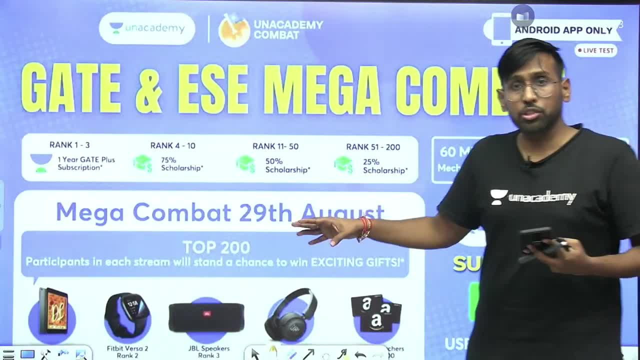 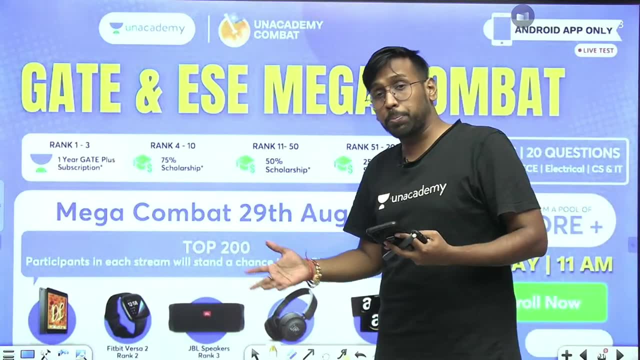 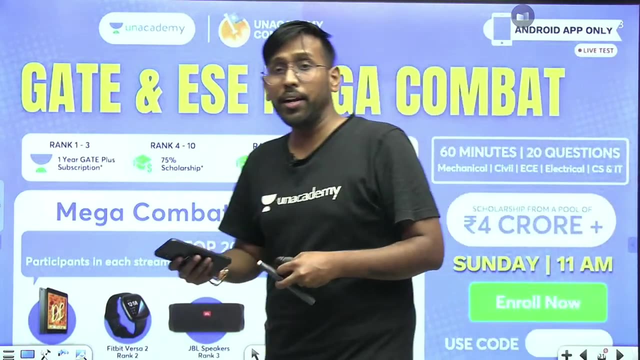 But along with that, you can also get extra gifts. maybe your Apple iPad, right. it may be your watches, it may be your JBL speaker. Amazon vouchers- right, Brother. now it's up to you what to do. Right, so you can join it using the code BHAAT10,. don't forget my friend. so you can go for the combat quiz. 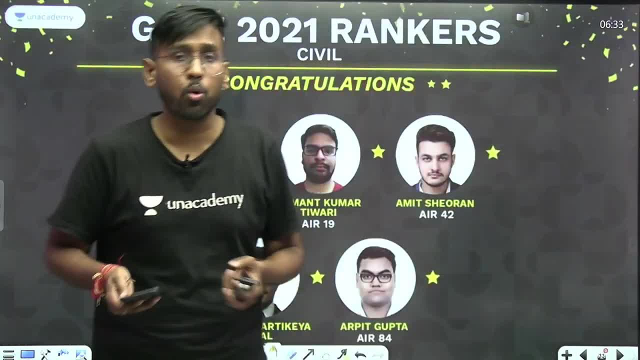 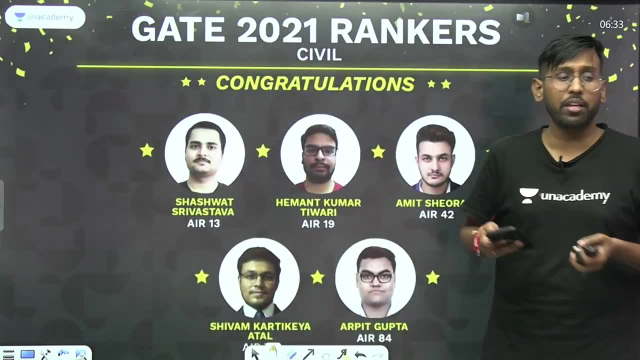 whether it is a test or a plus subscription. you are going to use the code BHAAT10 to promote me more on the Unacademy right And, my dear friend, I want everyone to prepare in such a way that they come in the top 10, 100,000.